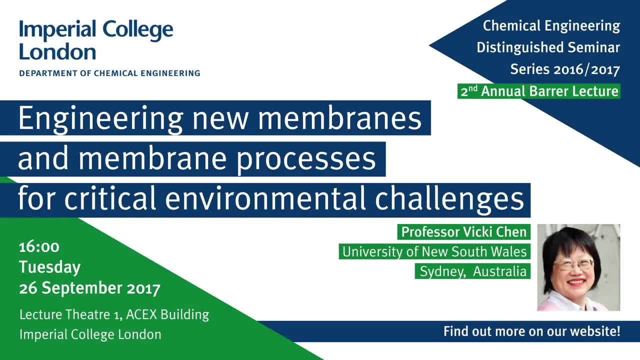 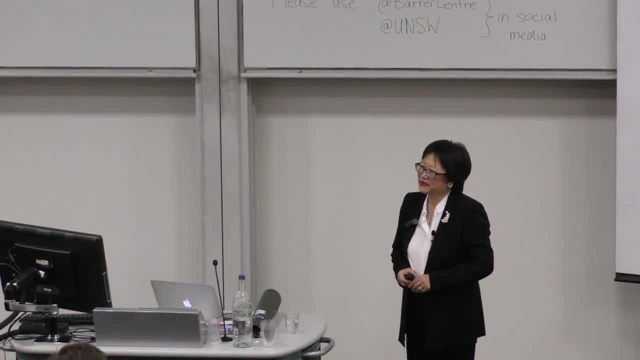 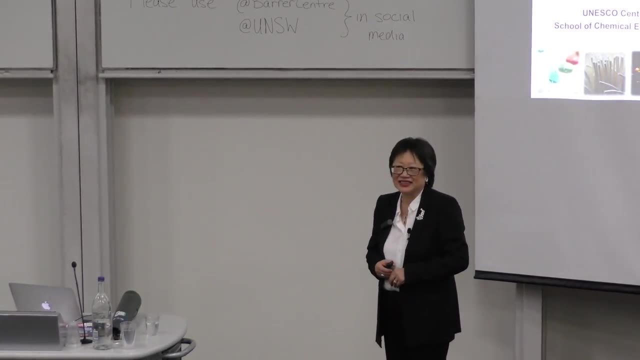 It's my real pleasure and honor to be part of the Behr Lecture Series, obviously following on the distinguished footsteps of Richard Baker, who is the first Behr speaker. The areas that he's covered is very well talking to you about memory processes and today I'm 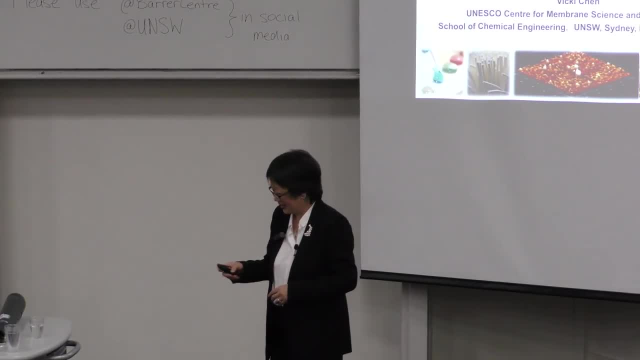 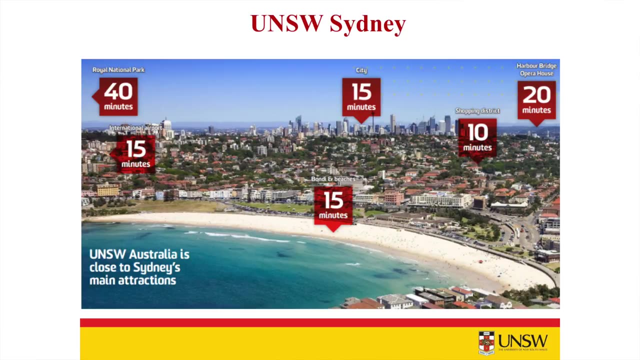 going to talk about memory processes, but a little bit more focused on materials. So first I want to start by saying where is the University of New South Wales in Sydney? I think I only need to show you one slide about where we are: 15 minutes away from the beach and the 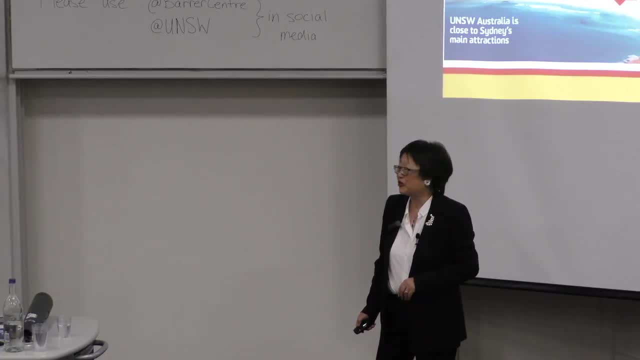 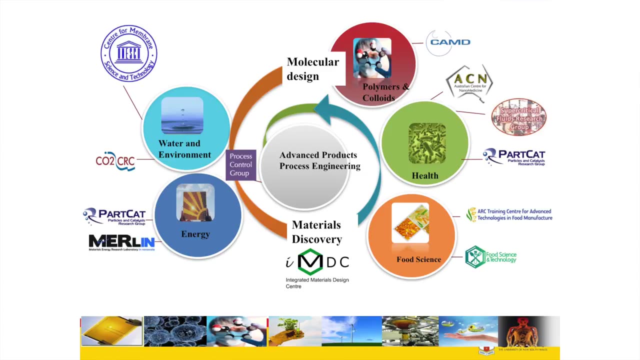 centre of Sydney. We're a very large university, over 40,000 students, and in that respect we are a very large multidisciplinary school covering membranes as part of environmental technology, but also a very wide range of groups from macromolecular colloids to health. 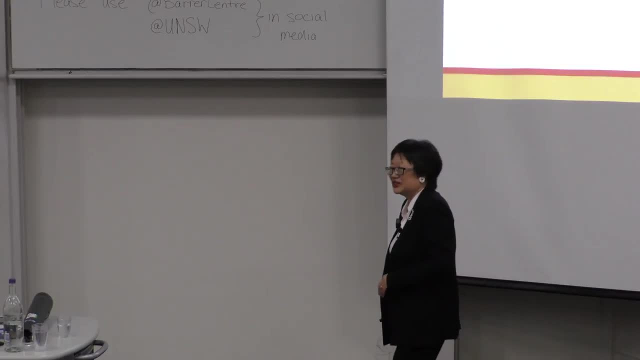 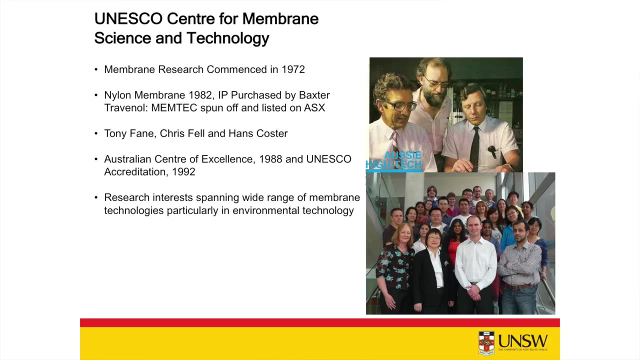 to energy. So the UNESCO Membrane Centre is a very long standing centre, over 30 years old, and founded by Chris Fell, Tony Fain and Hans Costa, and it's really spanning a lot of membrane technology, particularly in environmental technology. So we want to this. 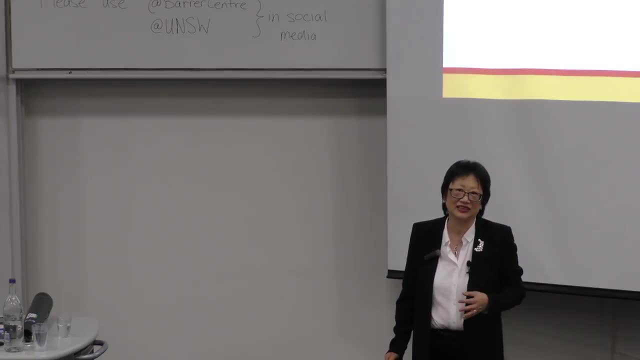 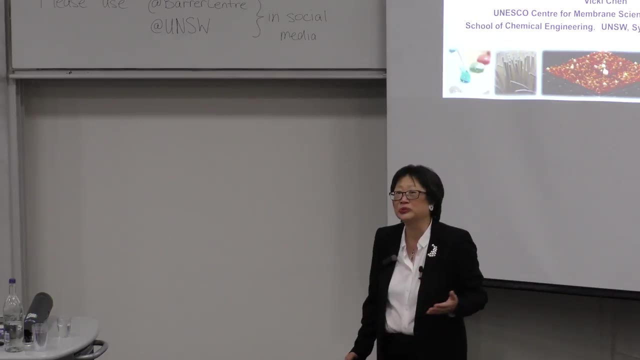 is one of the areas that we particularly have a great deal of focus on. So today I want to talk to you about some of the challenges that we generally chase as a global community in the environmental technology area, and some of the new membrane materials and processes. 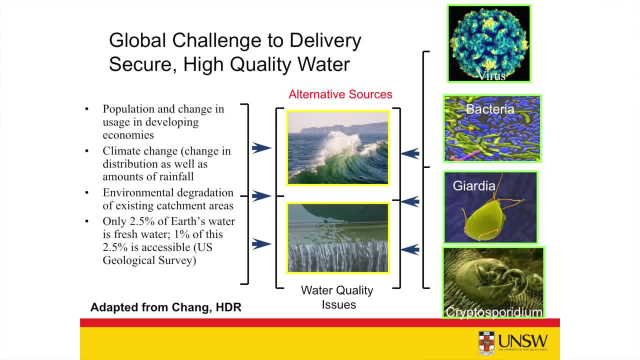 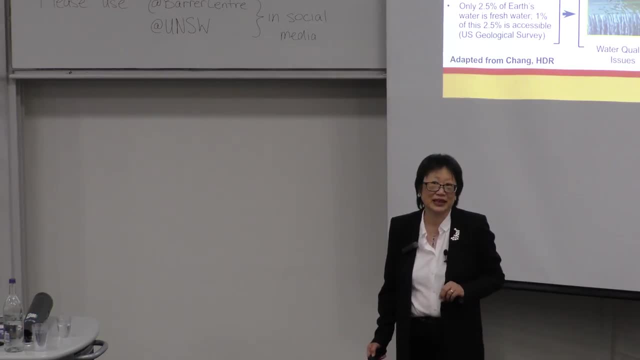 that we are working on within our university. So, of course, one of the challenges is water, both in terms of looking at new alternative sources, but also water quality issues. We have contamination from pathogens, but also of chemical contamination: contamination of chemicals of concern and crime disruptors. 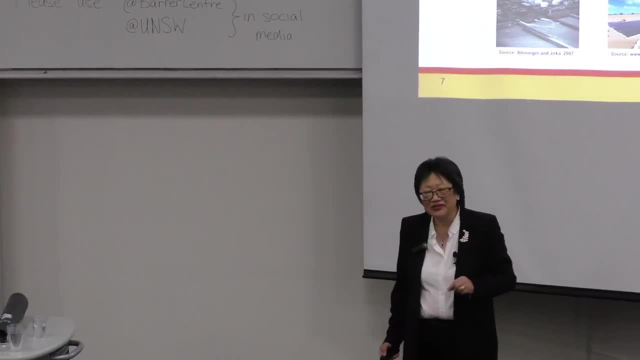 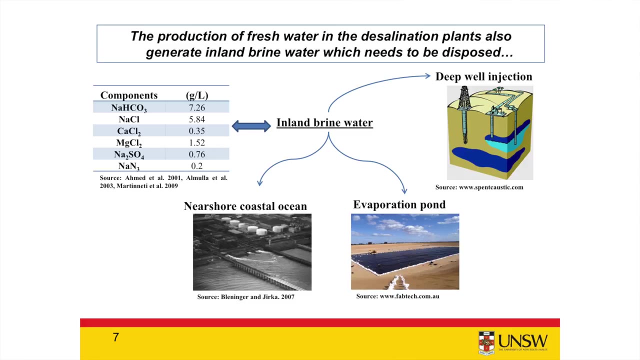 and things like that. However, one of the new areas emerging in terms of water quality treatment is also in terms of brines, How we have concentrates coming out of our membrane processes, reverse osmosis and others which now need to be disposed of, And these formerly were done in injection evaporation. 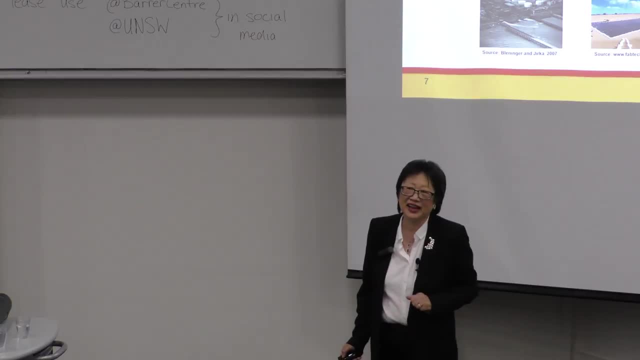 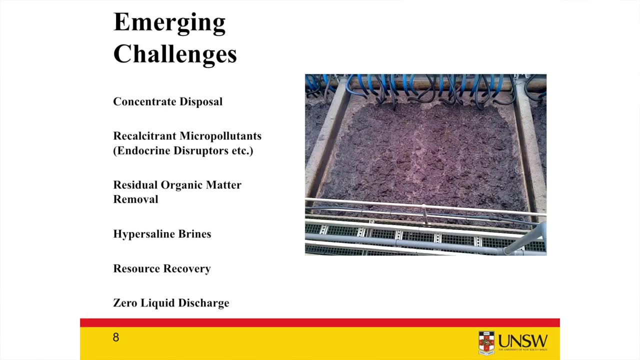 ponds. but the critical thing is: can we do more with that and how can we dispose of that more sustainably? The other emerging challenges, especially in water, are things I mentioned- concentrate disposals, costing us now potentially to dispose of the concentrate of our membrane. So we 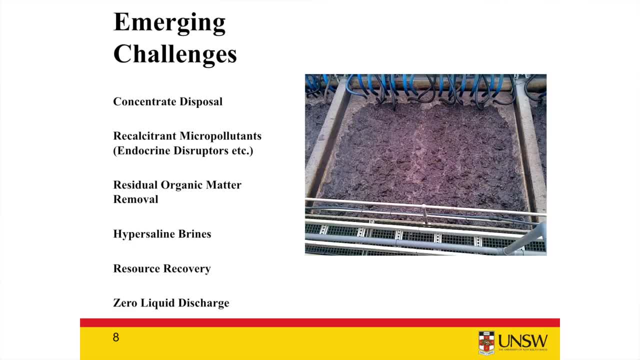 need to get rid of our membrane processes as much as to actually treat it. The recalcitrant micro pollutants, as I mentioned before. Residual organic matter removal: once you get to very small levels of organics, you still have issues with disinfection byproducts. How do you get? 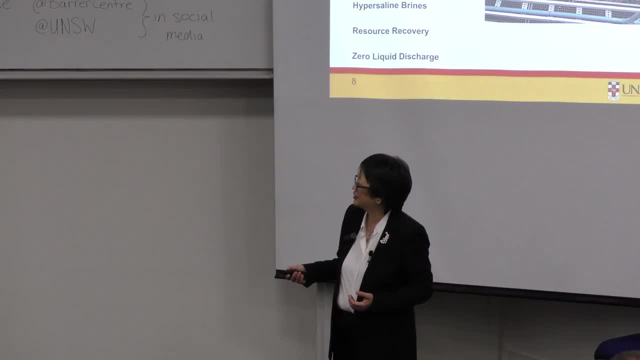 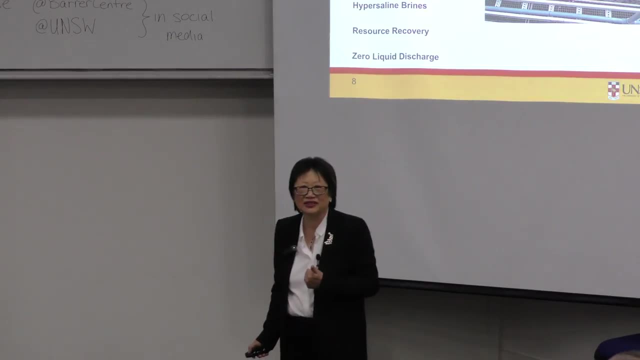 that last bit of humic acid out without going to full resourced osmosis. I mentioned hyper saline brines and one of the things is also resource recovery. Can we recover valuable mineral salts such as lithium- other valuable minerals- from those processes? So we need. 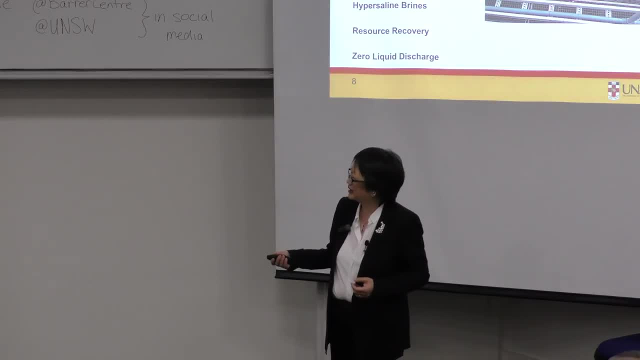 to get rid of that And we need to recover the mineral salts so we can do that with the other liquid And we need to do that with the other liquid too, And finally, a lot of our interest now is going to total zero liquid discharge. So those are some of the 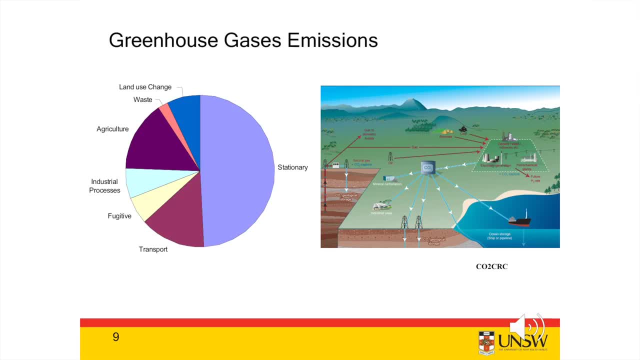 challenges and terms from the water point of view. If you look at greenhouse emissions, we typically think of stationary sources, power plants, etc. but there's also others: fugitive emissions, industrial process, agriculture. Now, a lot of the work that's been done is really on carbon capture and storage. So just to summarize, 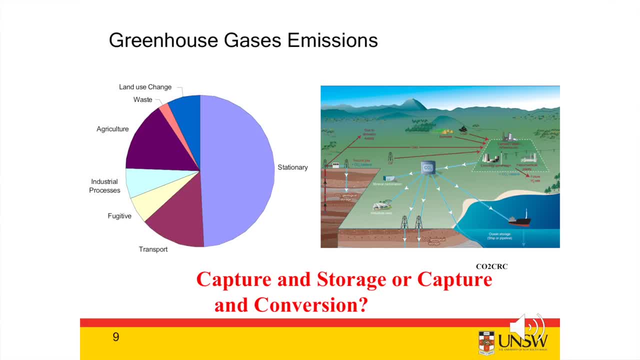 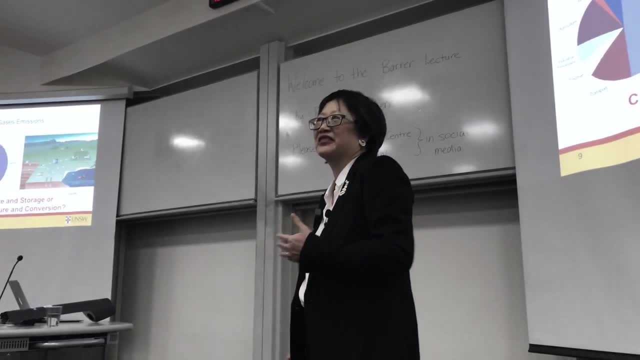 here's the first example, But we are now going to, in the future, thinking about also carbon capture and conversion, And that's a very challenging but a very interesting place to go. So I won't have a lot of time to talk about the conversion. 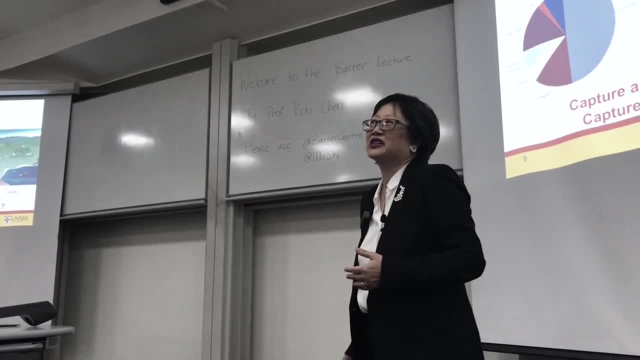 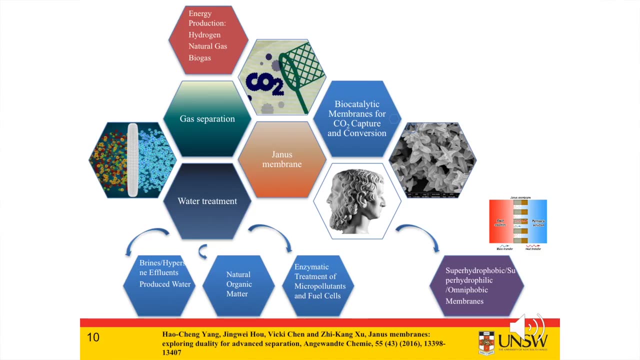 issue, but I will talk a little bit about things that we're doing in terms of carbon capture with membranes. So the scope that I'm going to talk about today is, as I said, gas separation and water treatment, specifically on CO2 capture. 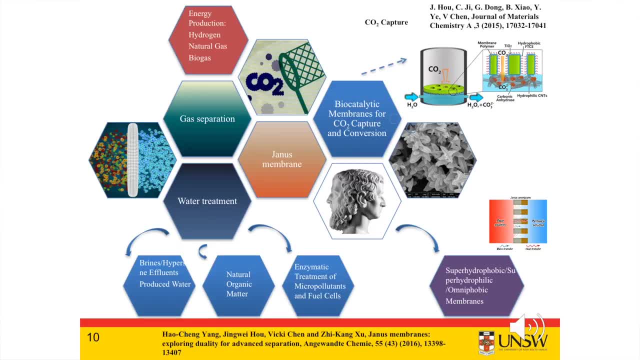 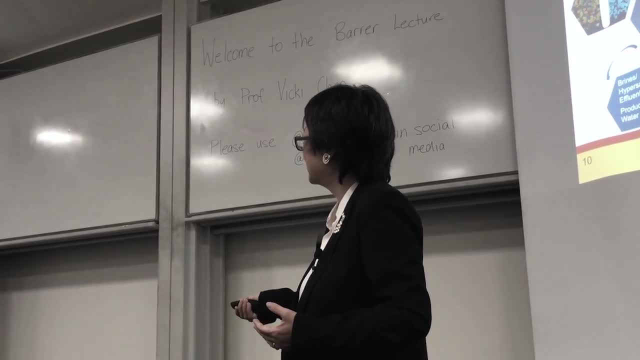 But we're also doing a lot of other work in the bio-catalytic processes for CO2 capture In the water treatment we have brines. I will talk specifically about this. The others we also are doing work in, but I won't have time to go through them. 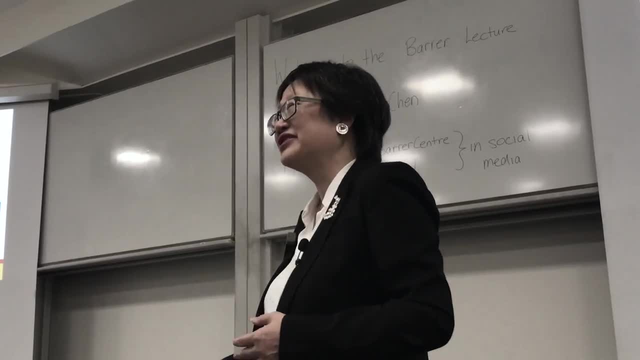 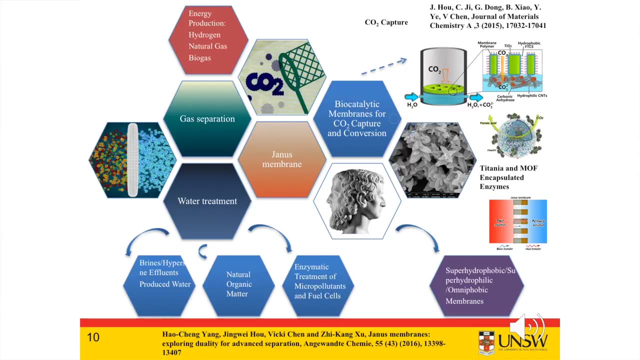 But the bio-catalytic membrane is also a combination of membrane contactors and enzymes. Part of the work was done recently in our group And we're also moving into, for example, encapsulating some of those. So we're going to look at some of the enzymes that. 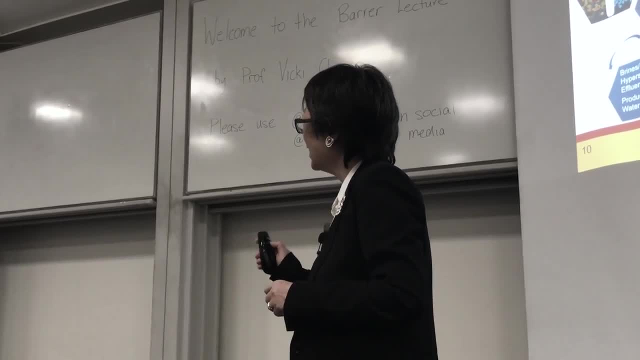 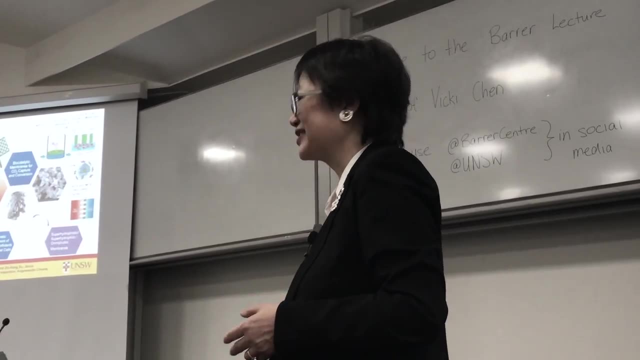 capture CO2 into MOFs and other nanomaterials. So today, for a few minutes, I'm going to touch upon a few areas I think of interest that look at some of the slightly different ways of functionalizing membrane, developing new membranes. 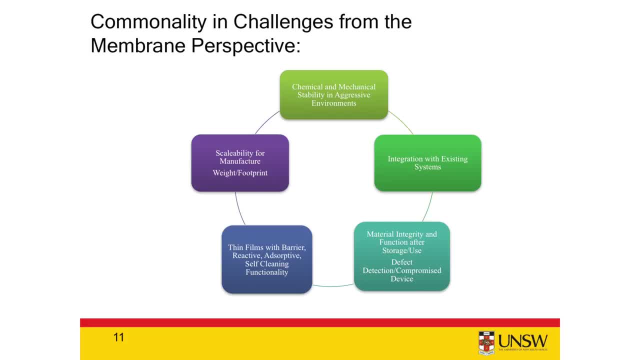 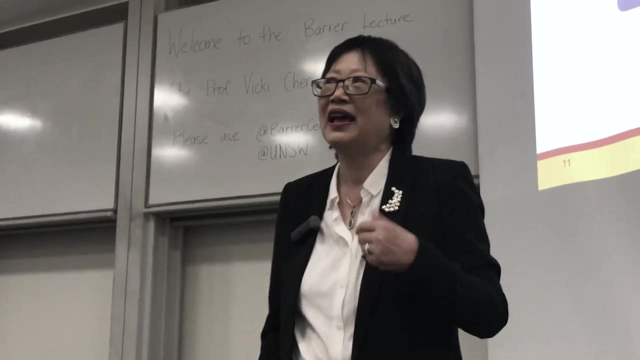 for these processes. So let's look at the commonality in developing membranes. First of all, we have issues with chemical stability. We need scalability, We need the ability of manufacture, We need integration with existing systems And this is very important in terms. 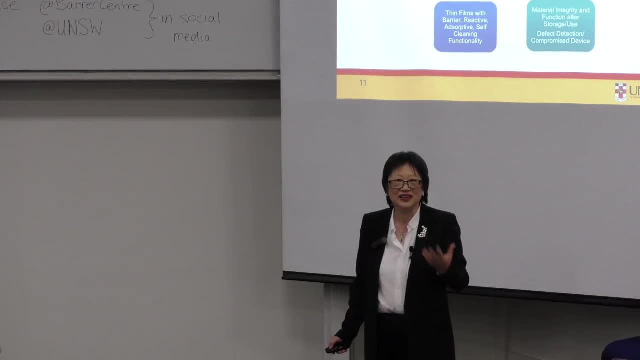 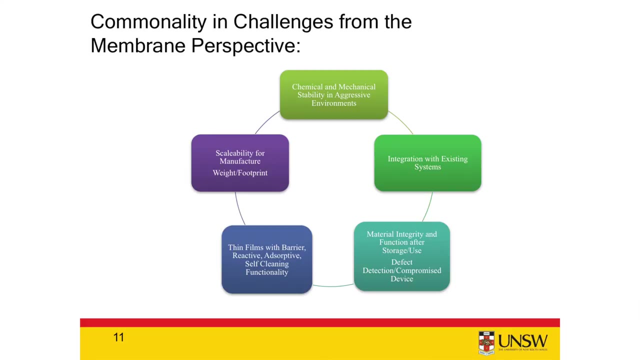 of talking about how membranes will be targeted for specific CO2 capture. It's not a silver bullet membrane that does everything: high selectivity, high permeance. It's got to fit into the overall CO2 process train. Other things are thin films. 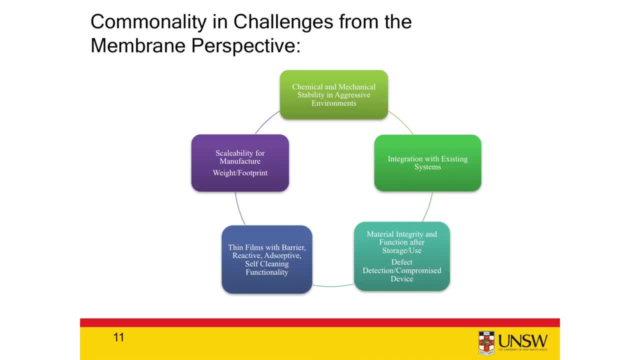 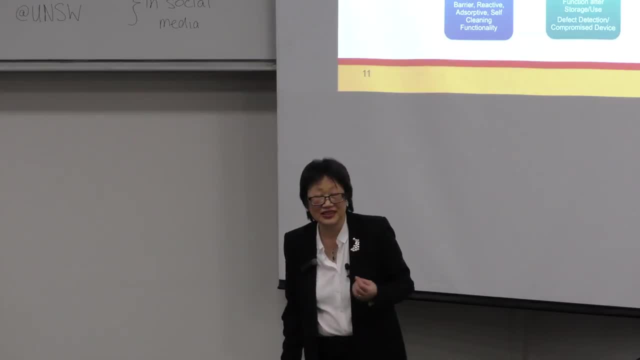 Are they just barriers? Are they reactive? Do they have self-cleaning functionality? some of the new areas- And also membrane integrity. Are there any defects? validation: Those are some of the challenges of developing new membrane materials that are beyond just simply synthesizing. 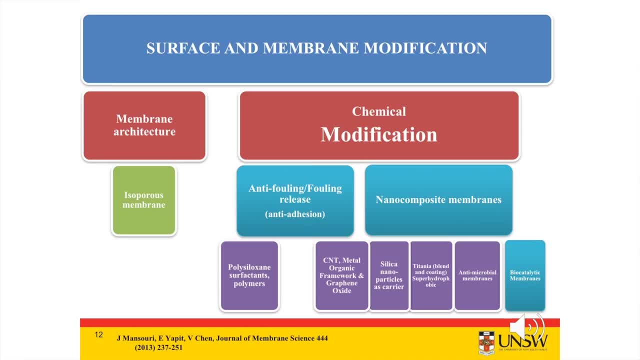 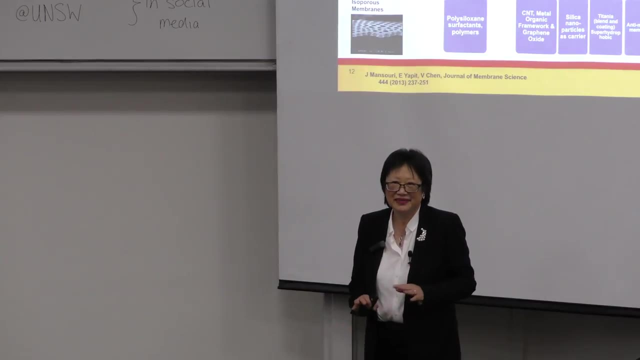 of next, wonderful nanoparticles. So in terms of surface and membrane modification, we can talk about looking at wonderful membrane structures. So see some of the isopores membrane: They're wonderful but not scalable And in fact, when we look at the separation, 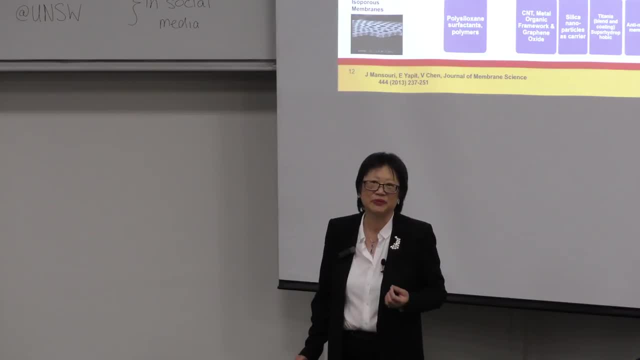 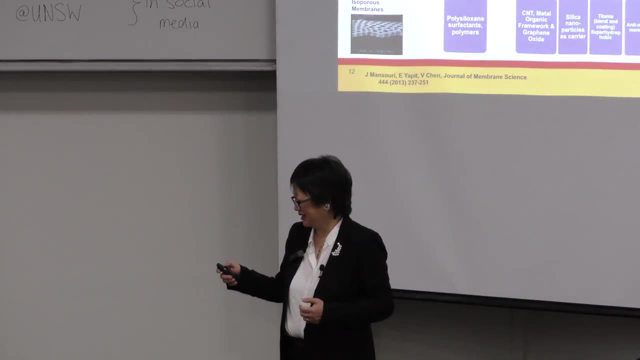 they don't actually give that much additional separation capability. They're, I say, beautiful as an image, but one of the I said in terms of application a little bit less, But what's really useful are more like things that. 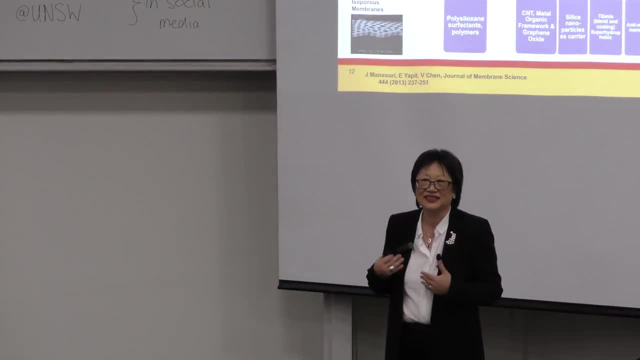 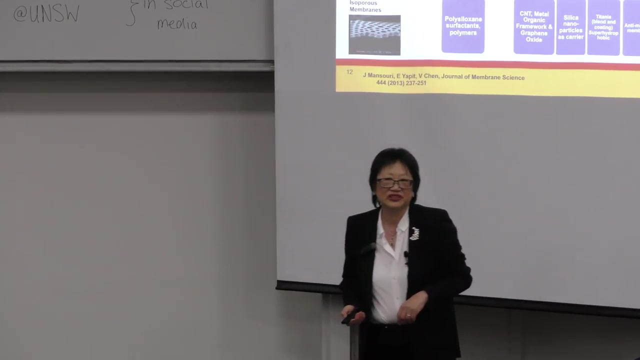 how can we actually integrate materials that gives you self-cleaning functionality and things like anti-fouling, anti-release, low-energy material? How do we integrate that into membranes for water treatment? Nanocomposite membranes are the ones that I'm going to focus on today. 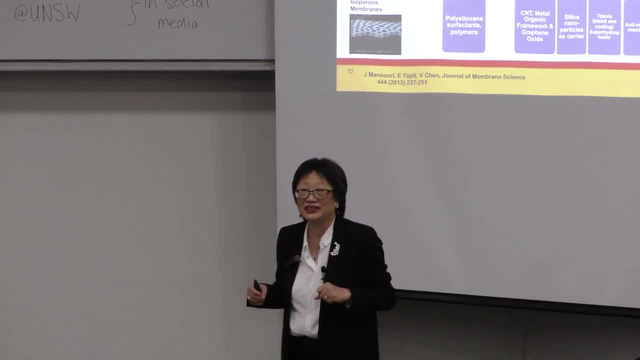 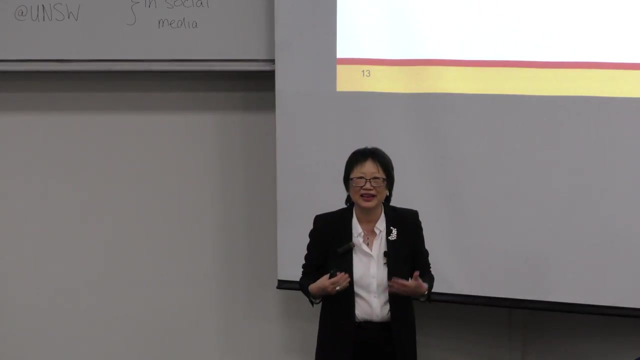 because they're basically giving us a different handle, different levers for us to tailor membrane materials in a way that we haven't been able to do so in the conventional polymer synthesis. So the opportunity now are even looking at hybrid materials. I'm talking organic, inorganic composite. 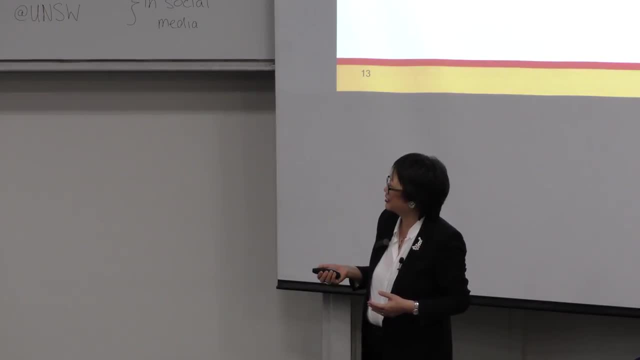 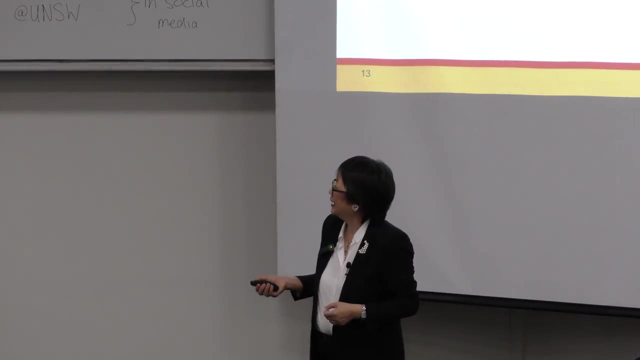 And what we want is usually when you talk about nanocomposite, you're looking at mechanical strength, thermal stability, but really thinking about: are there better ways to improve separation and permeability, both chemical and mechanical stability? and, as I said, it gives us another lever to change the membrane properties. 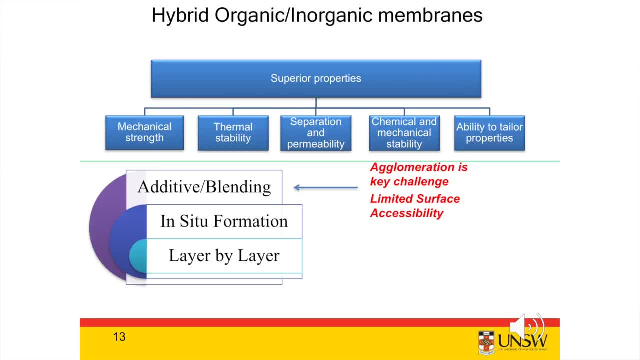 So the approaches people have done in terms of either additive blending- but that has issues with agglomeration- If you just simply add nanoparticles and nanomaterials- limited surface accessibility- we can form these nanomaterials- or inorganic. 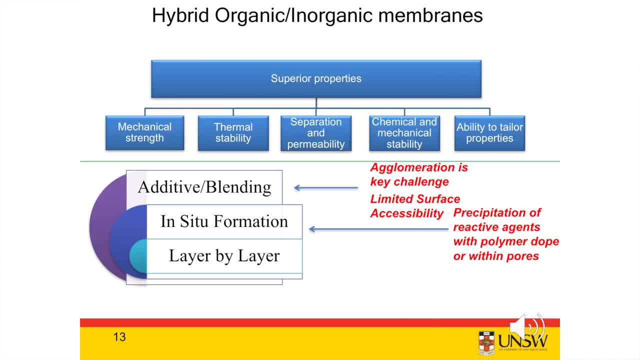 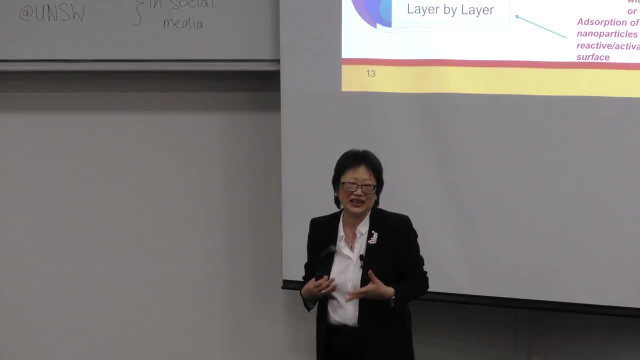 constituents at the interface, But that requires some reactive agents or controlling where they form. And finally, we can think about how we can actually do nanoposite membranes layer by layer, And this is a little bit different from the normal way that we think about nanocomposite membranes. 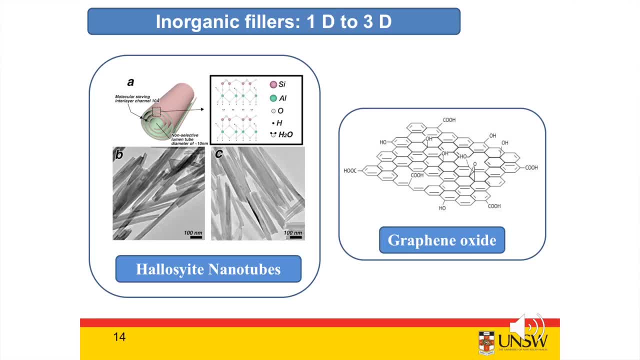 Oops, let's go back here. So let's look at the type of fillers we're thinking about. We can think about 1D material. Calcite nanotubes is an example. Carbon nanotubes are another. These are functionalized clays. 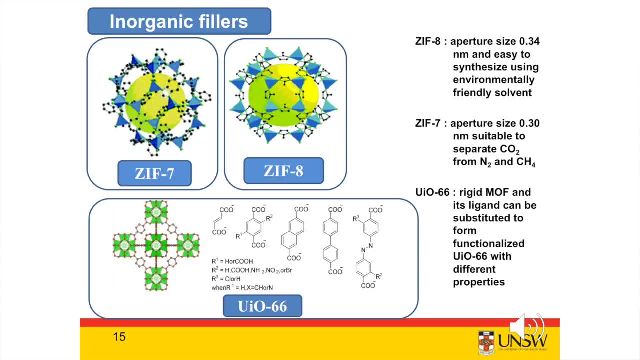 We have 2D materials like graphene oxide, one of people's favorite alternatives, And we have 3D materials, framework material with ordered structures, and these have ability to control your aperture size, things like ZIF-7, ZIF-8.. 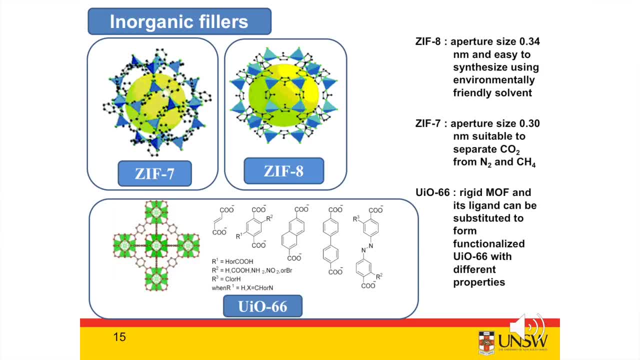 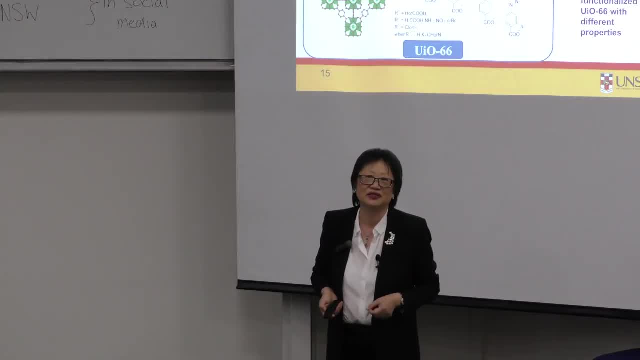 But also we have things like UIO-66, which is a metal-organic framework with a lot of functionalities. I've been able to functionalize with different properties, So I'll talk about some of the consequences of some of those functionalization. 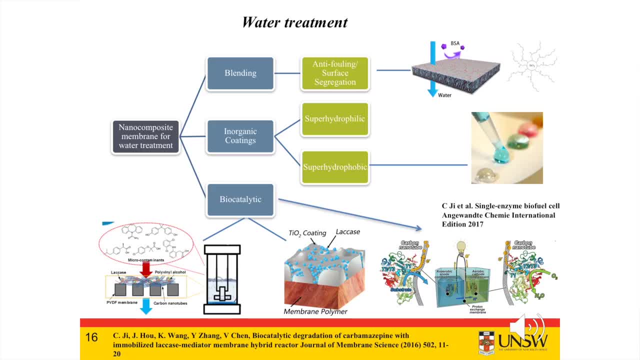 Now I'll start first by looking at the water area. In the water treatment area we have several very important applications. I said the cleaning, self-cleaning application making surfaces, But we also have issues in terms of: can we make a new types of membranes for water treatment? 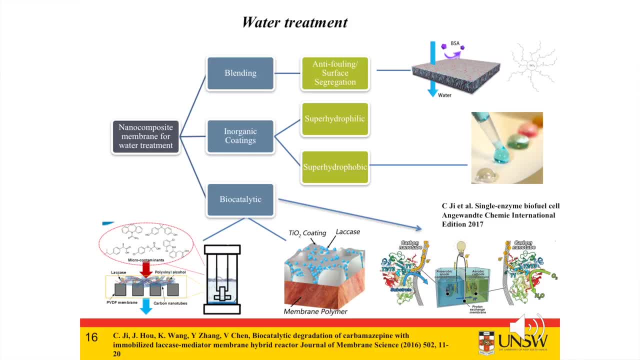 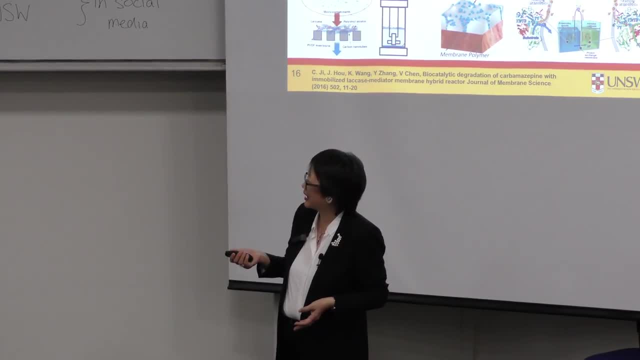 that are a composite, The membrane. These are inorganic coatings, not just blended-in component. They're super hydrophilic, super hydrophobic and we also can functionalize them to biocatalytic. We won't have time to go through this particular piece of work. 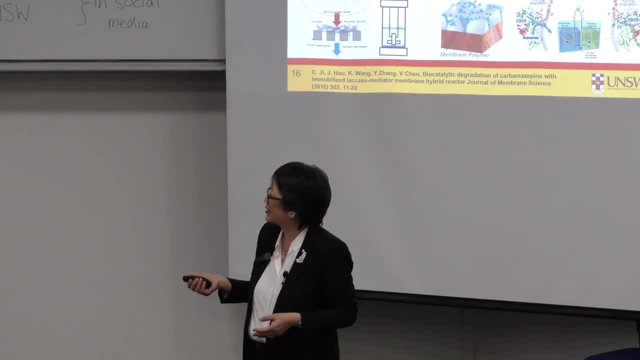 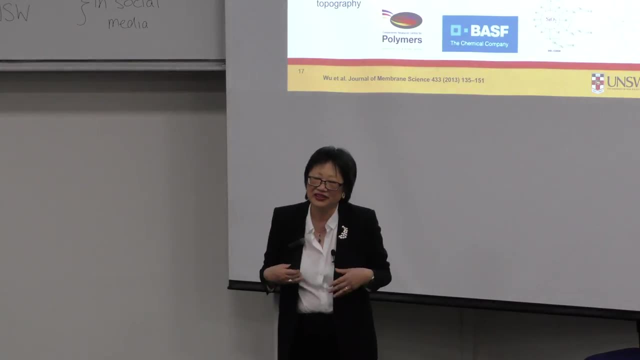 but it is an area that we are particularly interested in: combining enzymes with functionalized membrane surfaces. So in the area of anti-fouling, most of the people have looked at grafting surface functionality, But one of the things that we've found is that 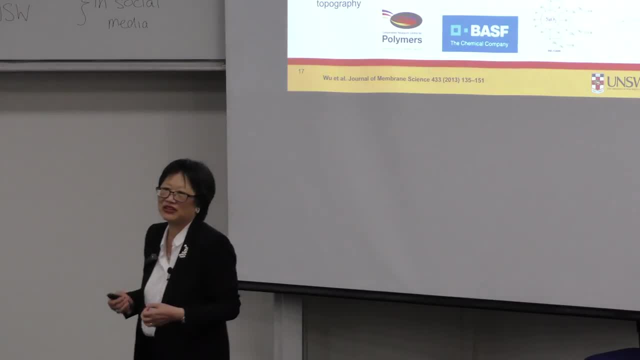 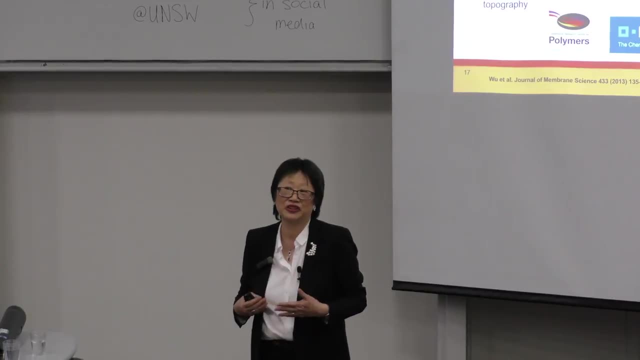 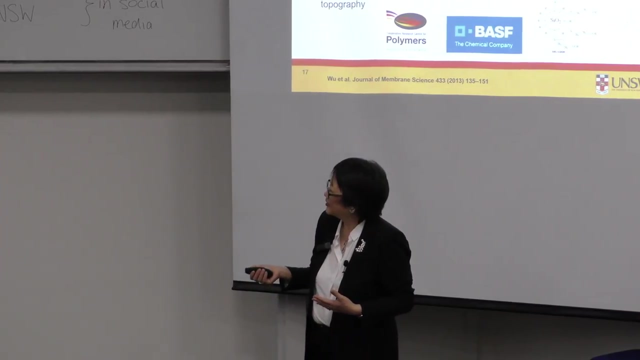 one of the things is that is often quite difficult from the manufacturing point of view, Post-fabrication grafting. most membrane materials are mechanically chemically stable and therefore you have to use quite extreme conditions to get that functional groups and enough density to give you surface functionality. 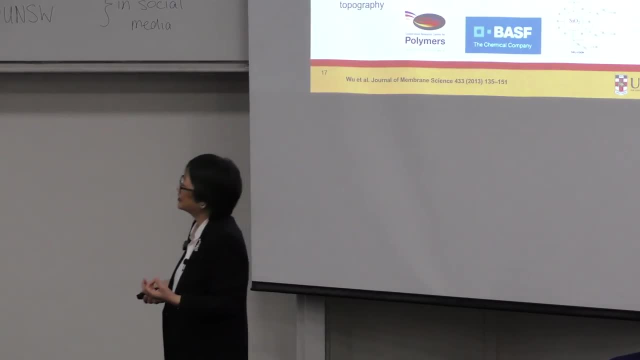 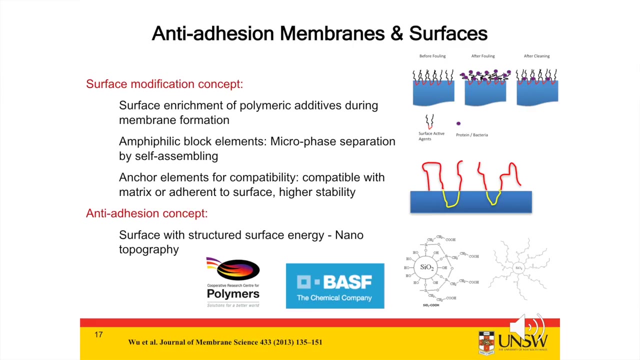 What we want to do is looking at another way. We can add materials that self-segregate to the surface, So we can have low-energy blocks with tethering polymer chains which allow for a very high degree of surface change that these spontaneously surface segregate. 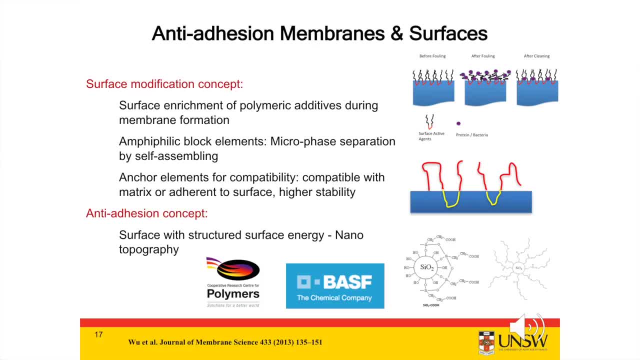 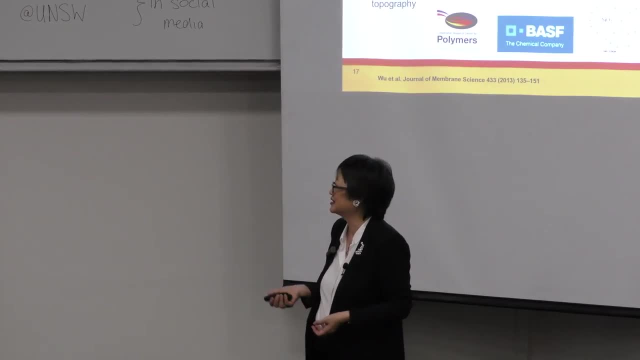 during the phase inversion process, driven by the thermodynamics of solubility, relative solubilities of the different groups, And these allow us to then basically blend these materials without changing the manufacturing process and allow us to not use as much, because these all enrich at the surface. 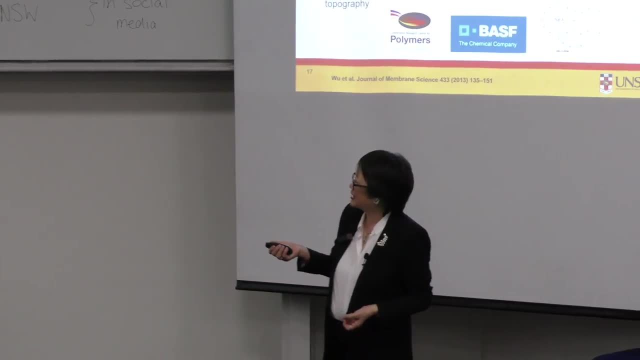 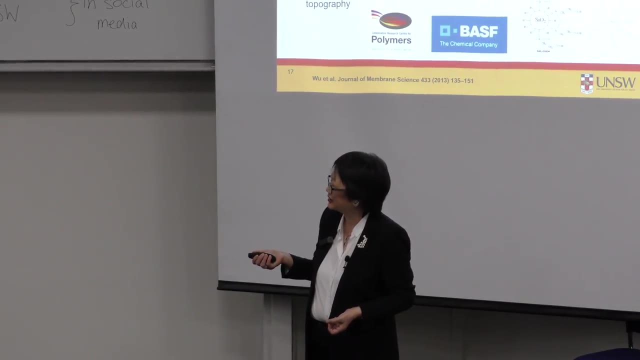 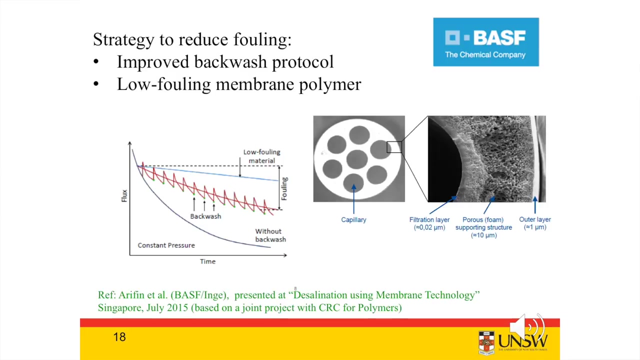 So this is part of the work that we did with BASF. Another way is tethering these, clean, these hydrophilic or low-energy components onto nanoparticles. Again, these will also spontaneously self-segregate. So do these work? Well, in fact, one of the things that they've actually now done- 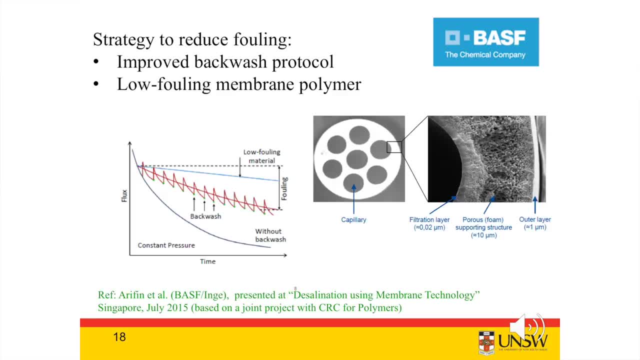 is upscale this particular technology. The BASF developed a range of a library of these materials. They've put it in capillary membranes and you can see here, without the version material, you get a continuous drop in flux over time With these low-fouling materials. 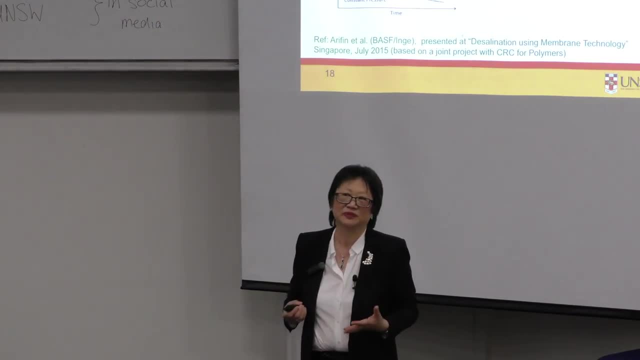 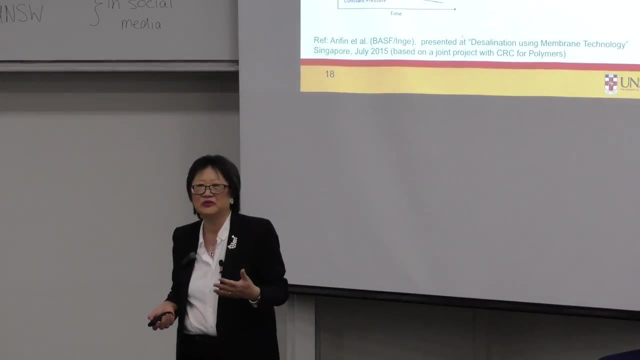 you still don't get a complete self-cleaning, but you get much better fouling resistance and fouling release, And this is quite critical. Many people focus on the initial fouling. What you really want is fouling release- ability to clean. 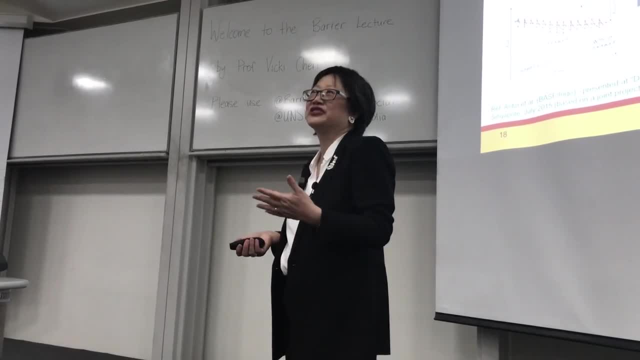 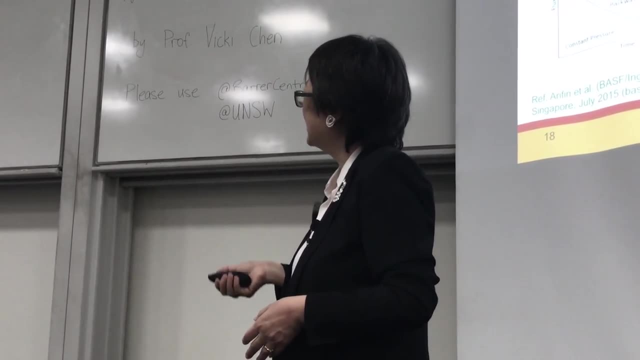 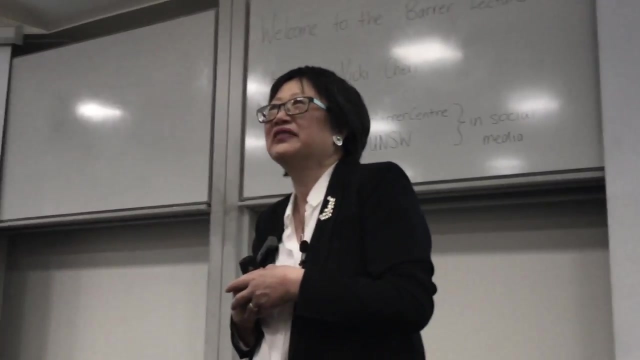 That's even more important in most cases than simply the first instance of fouling. So this is part of the work that's been actually starting to be translated into practical applications. Now, the second technology I want to talk about is membrane distillation. 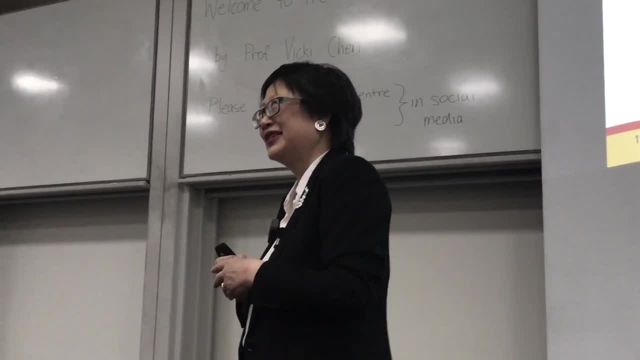 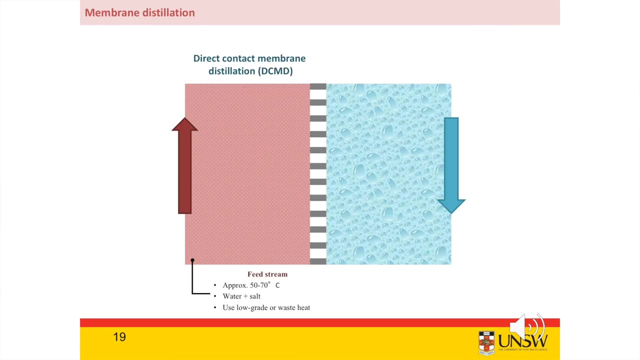 Now, membrane distillation was very fashionable about 20, 25 years ago, but in fact it's come back again And one of the things is membrane distillation basically involves a moderately hot stream, feed water stream, a permeate stream. 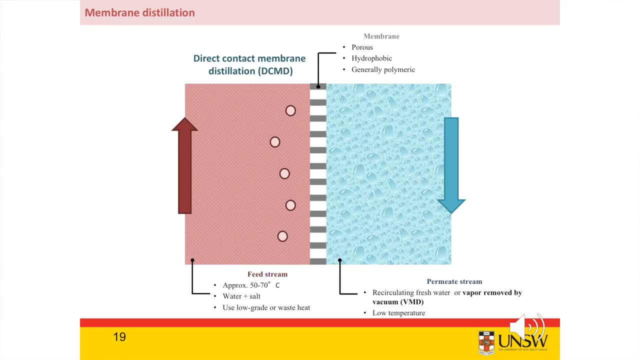 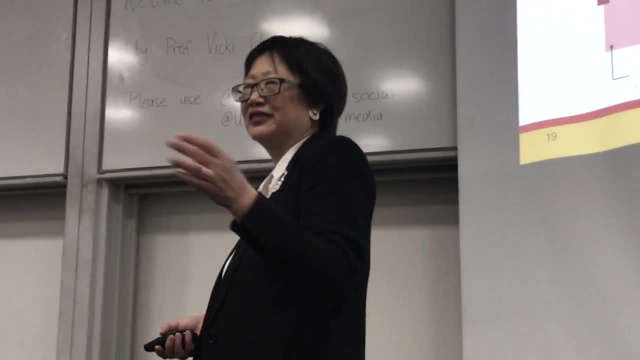 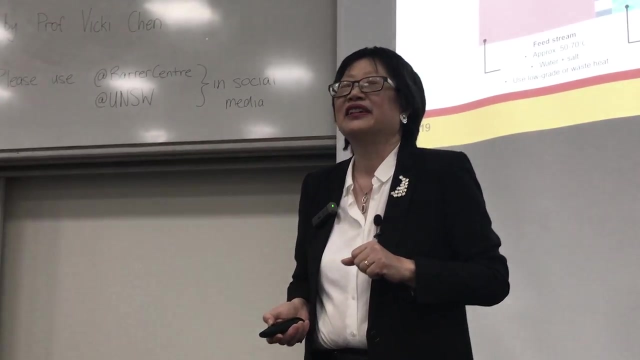 which is either cold water or a vacuum, and basically you've got a hydrophobic membrane, which is a liquid barrier, And what you have is basically water vapor going from one side to the other while rejecting the contaminant. So why is this particular application important? 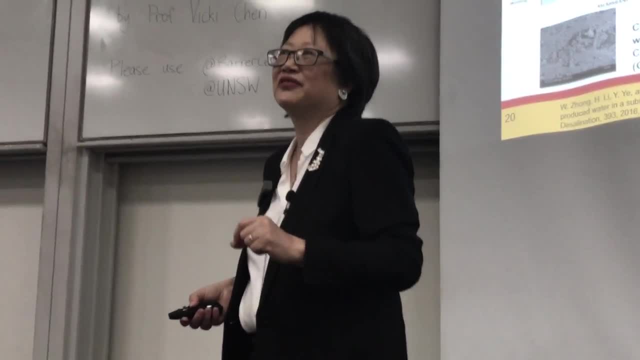 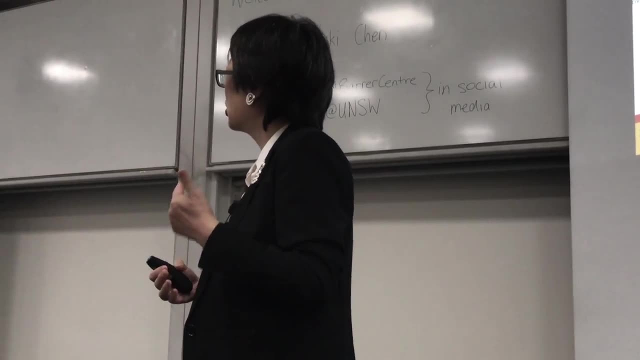 Well, the applications now coming up comes back to the fact that we're treating much more with calcitrant streams. now It's not just clean seawater. We're talking about industrial wastewater. We're talking about things with 100 to 200 grams per liter salt concentration. 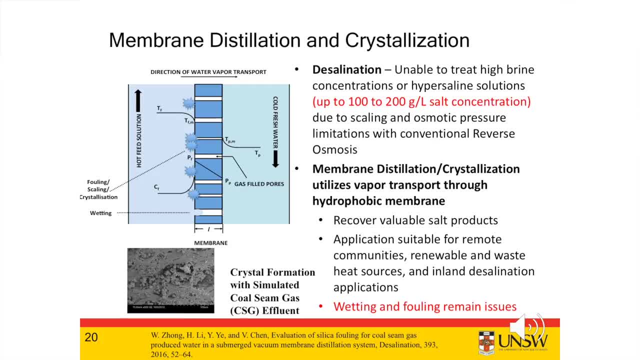 That's not something you can do. with reverse osmosis scaling, We've got osmotic pressure issues. The second thing is the interest now in using renewable and low-value heat, which is from solar, geothermal or actually just from waste heat. 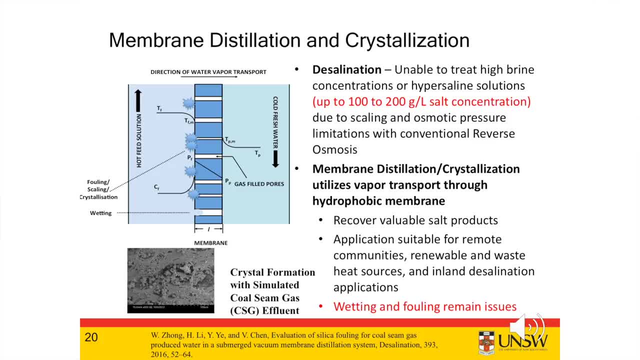 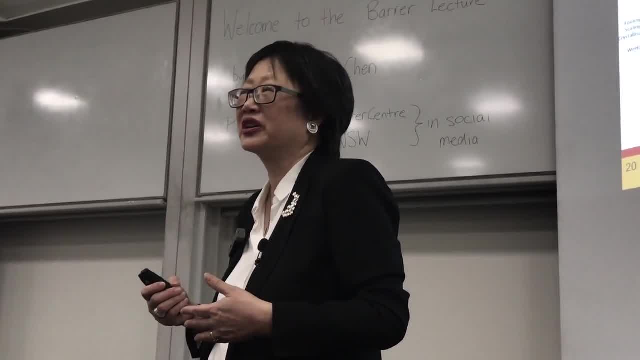 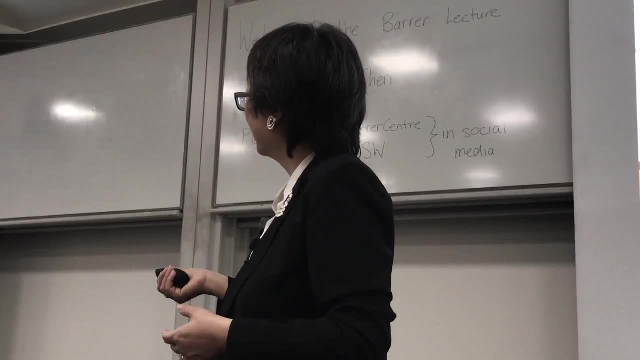 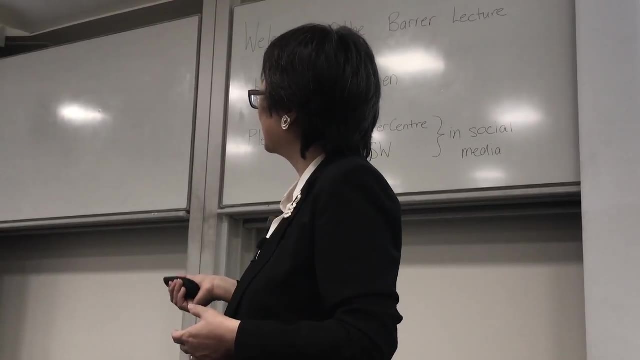 from power plants and inland, remote commuted heat sources. So this allows us to really start to concentrate those brines and actually produce fresh water using, as I said, relatively without going to high energy, high valuable energy usage. Now the problem is, of course, you've got wetting and fouling is still the issue. 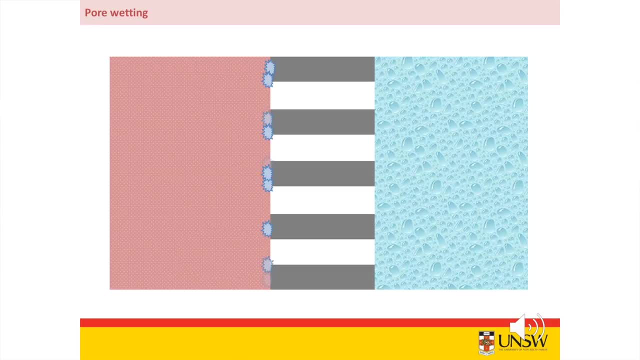 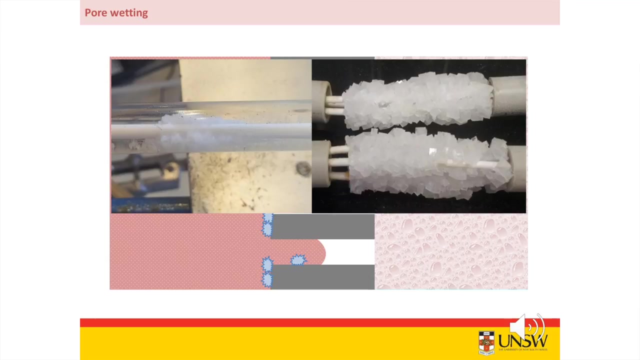 because as we increase the concentration to very high degrees, we could get scaling, we could get wetting. So we look closely at the interface. As we increase the concentration on the feed side, we get precipitation, especially divalent salts, And of course what that allows us then is hydrophobic membrane. 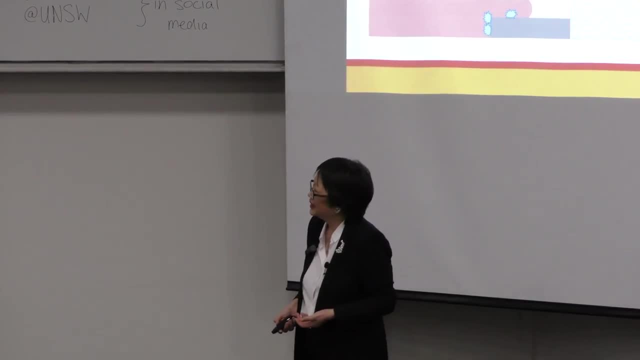 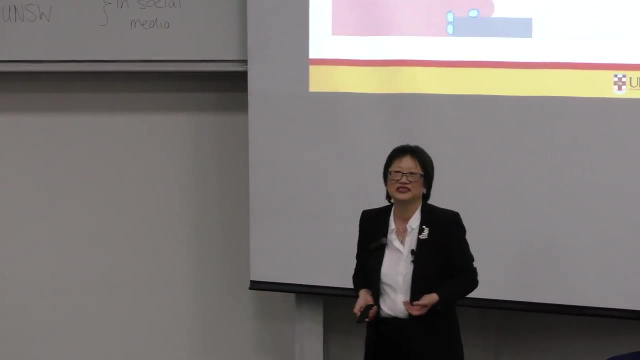 It would come eventually wet out. then you get contamination. So the approach that we want to do- and, as I said, it can be as severe as getting full-on crystal growth- In fact, these membranes still survive, which is pretty incredible if you think about it. 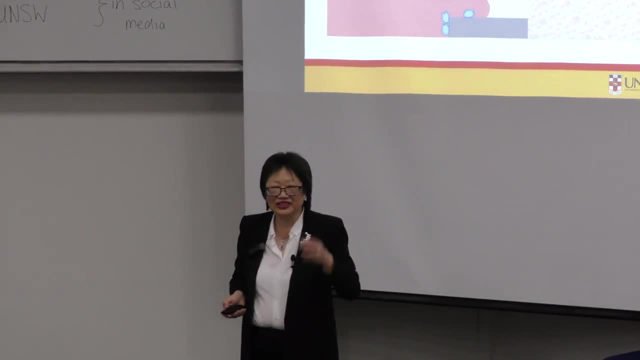 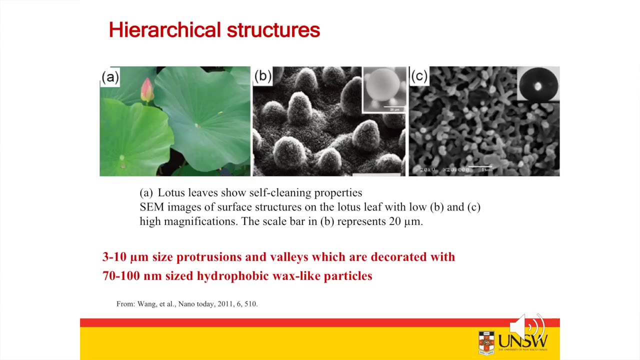 These membranes are recoverable. But how do we actually overcome that? So, first of all, we can make the membrane more hydrophobic. So what we can do is take a page from Nature and think about we can roughen, use the surface, make a hierarchically rough surfaces and make them super hydrophobic. 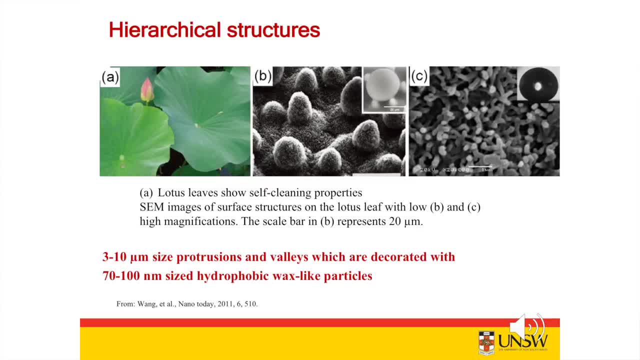 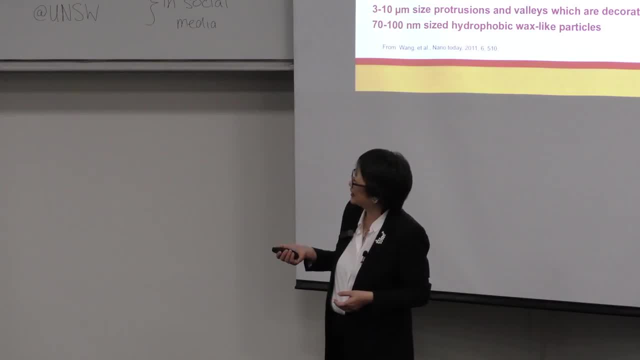 So one of the most famous examples is the lotus leaf, which has a dual hierarchical structure, a sort of a micron-type structure and then a sub-micron, and you can see a very, very high contact angle. Now it's hydrophobic because it's got wax-like particles. 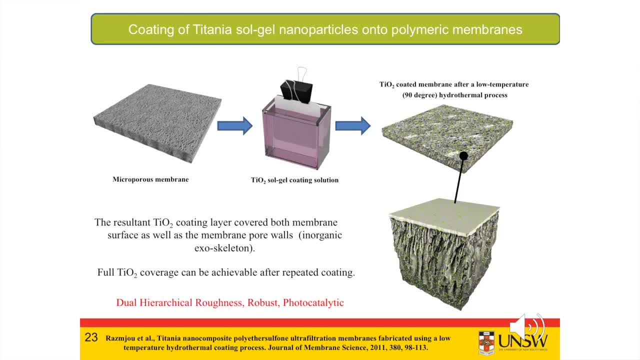 How can we actually replicate something like that kind of structure on the membrane surface? So what we do is actually: we thought about it and say: well, can we actually coat a polymeric membrane with a sol-gel solution? That sol-gel solution would actually crystallize under very low hydrothermal. 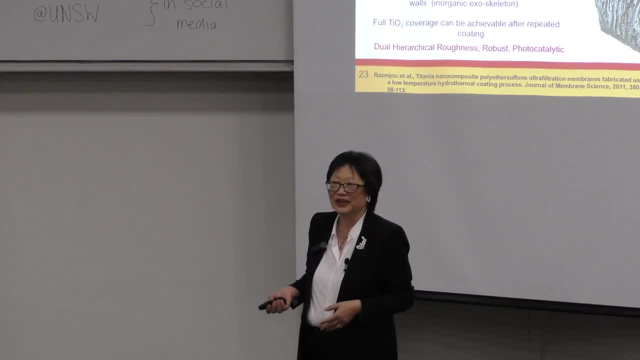 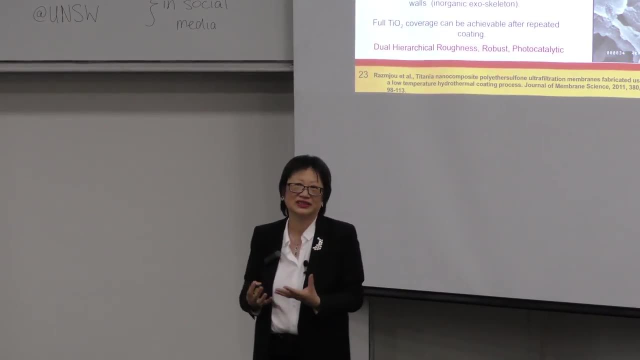 just basically hot water treatment and basically form a titania crust on the surface. So what we see here is the membrane now covered with this ultra-thin titania surface functionalization- What's really interesting, if you think this is being very brittle. 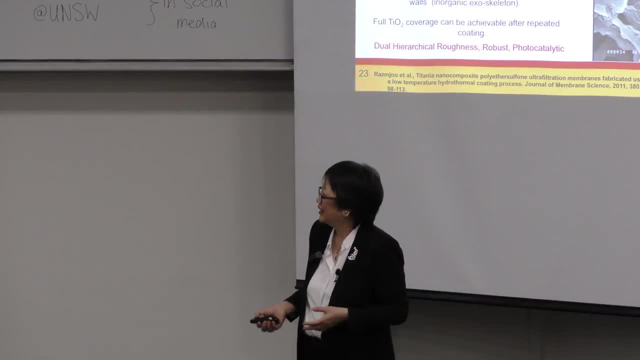 it's actually because it's so thin. it's actually quite flexible. And the second thing: we get this dual hierarchical roughness. It's actually robust. I can bend the membrane and it turns out to be photocatalytic. We don't use that functionality. 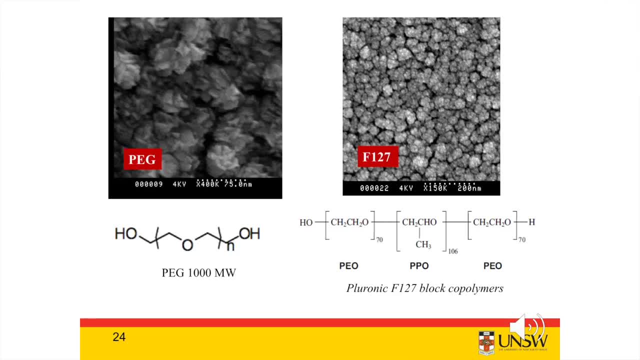 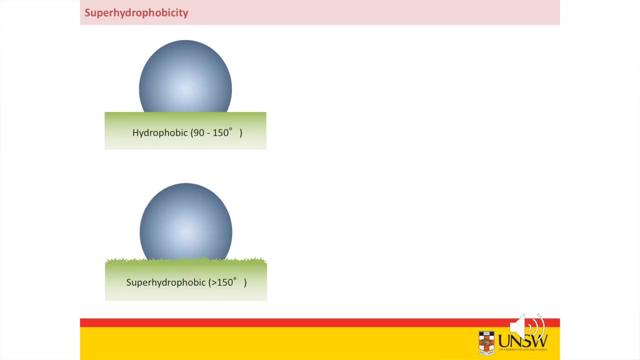 but it actually exists as well. So with that dual hierarchical structure we can actually play around with the architecture by using different templating agent in a sol-gel solution. So that gives it quite a different lever in terms of the structure, the surface architecture that we can achieve Now. we can now 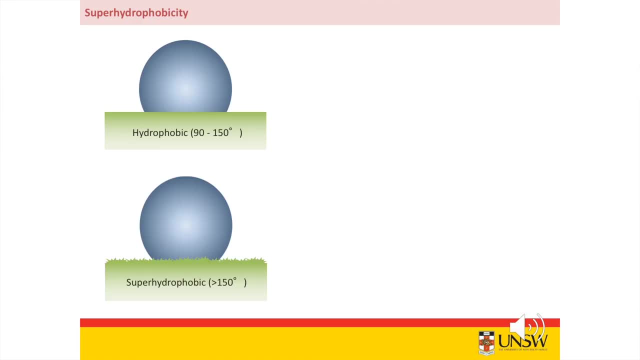 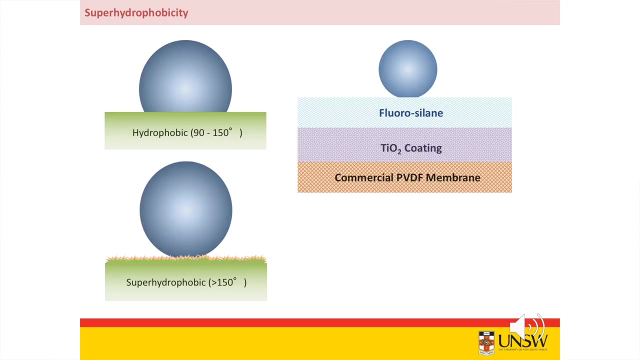 take that dual hierarchical structure and we can functionalise it by putting a making that super hydrophobic surface, by putting a silane group. So we've taken our commercial PVDF membrane, polymer membrane, we've done this roughening due to titanium dioxide And we now put a floor. 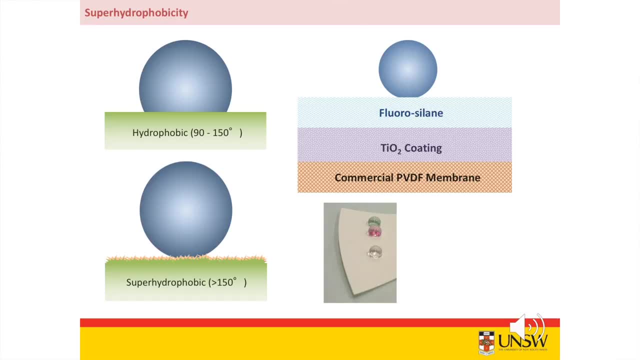 height, silane coating and now being able to achieve much higher contact angles. So we can see here that here's water, humic acid and other solution lovely beating up on our membrane surface And this is easily translatable to being hollow fibres, flat sheets. so it's not dependent, it's not. 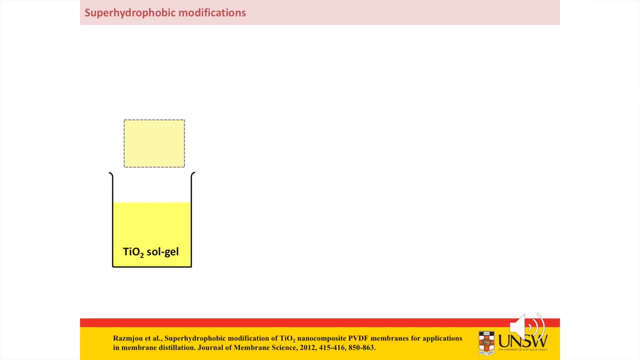 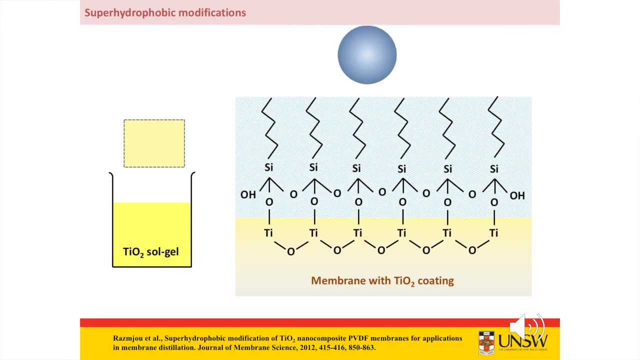 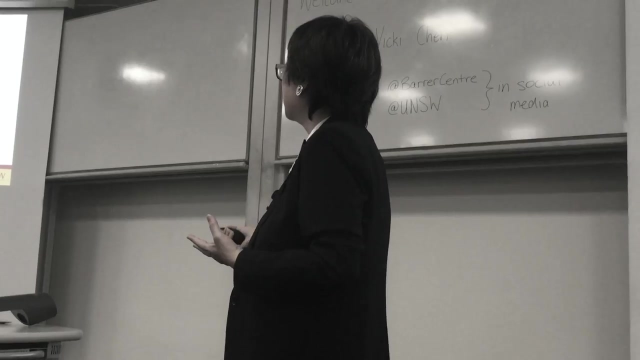 very heavily dependent on morphology. Okay, so, as I said, we've done this coating technology, we've taken now taken this: we now made this rather inert surface now functionalise with, basically, it's imitating a ceramic membrane In terms of this chemistry. we have those. 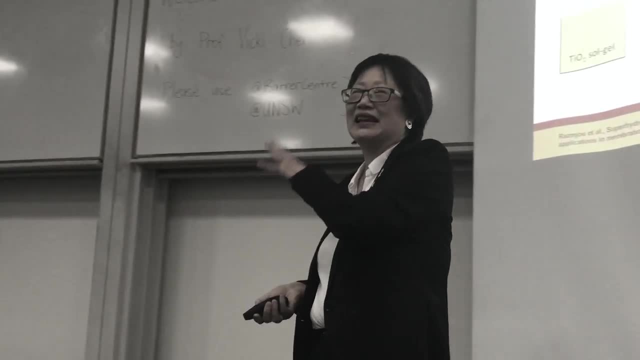 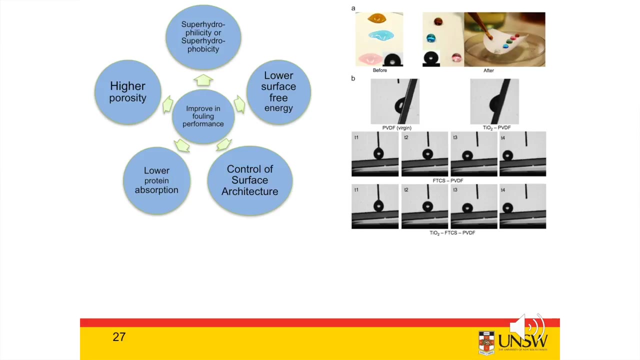 lovely hydroxyl groups. we can do a condensation reaction and get our silane groups on and we can achieve our super hydrophobic obesity. Now, this now shows you a way that, in terms of, rather than simply doing chemical grafting, we can 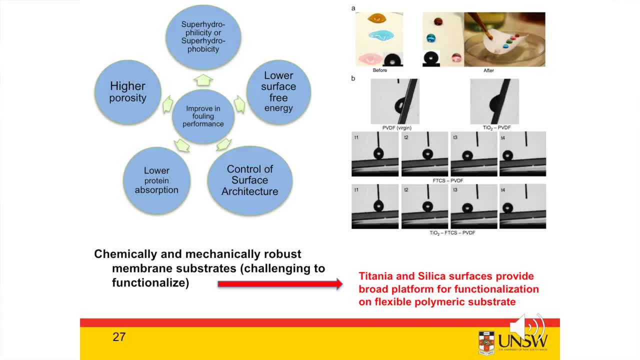 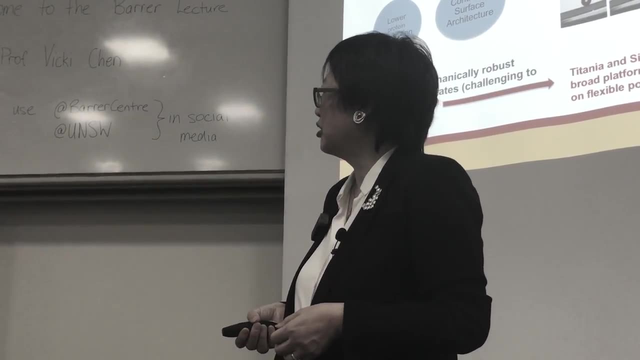 now, as I say, have a polymer membrane with aspect of a ceramic membrane surface, chemistry and the functionalisation that you have with a ceramic membrane functionalisation, So that allows us to get a chemically and mechanically robust surface and allows us to think about what other things that we can put on. 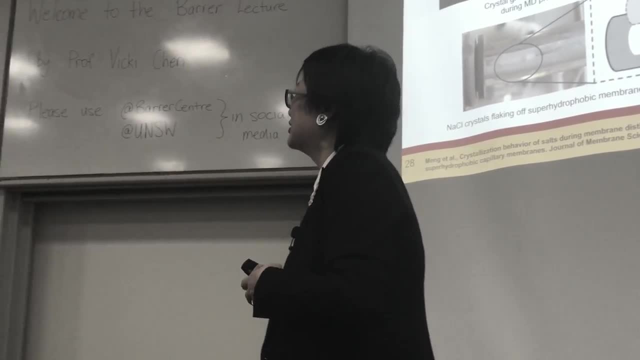 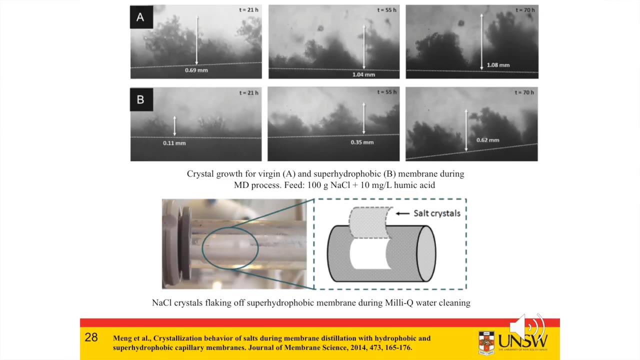 that that surface. The other thing is quite interesting is that when we do this coating, we've also changed the way that salt crystallises on the surface. if the version membrane, we get much more heterogeneous salt forming. With this titania surface we actually get much. 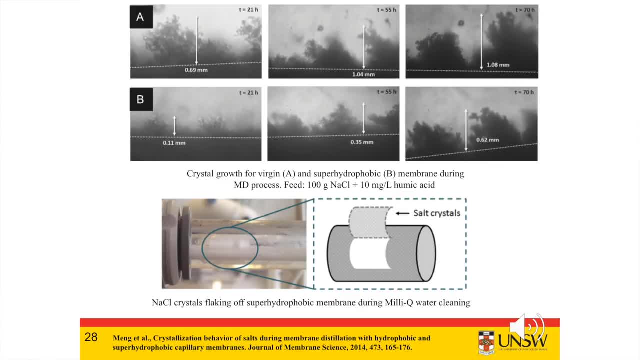 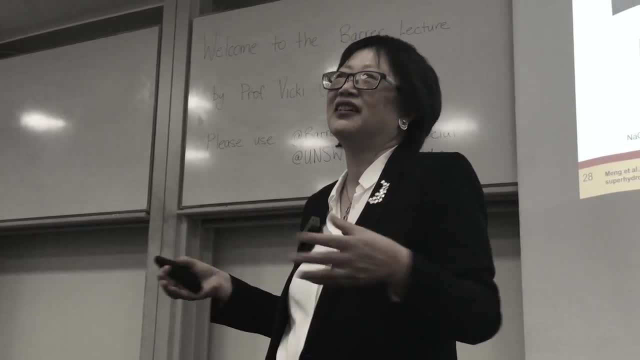 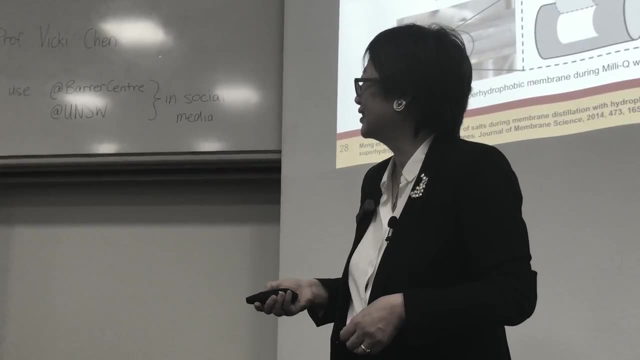 more, even crystallisation Later on. this will be important because we will use this for a different application. But the other thing is this: the salts actually will peel off the surface much more easily. they actually released much more easily from that super hydrophobic titania coated. 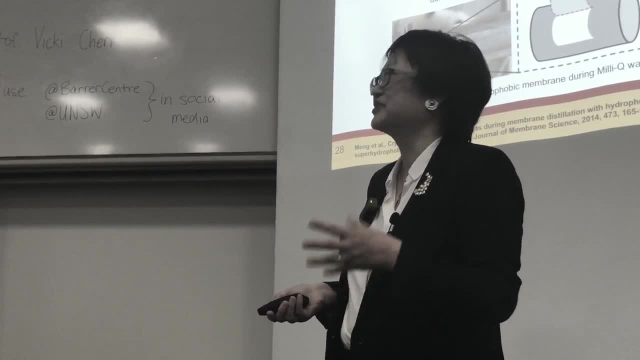 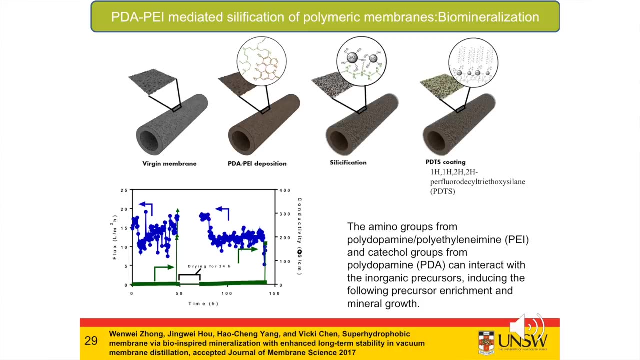 surface. So it's one of the very interesting side effects of surface texturisation, as well as the physical change. Now we can also play this game in the same way. it's called biomineralisation. Instead of using the titania substrate, we can use things like polyethylene amine and 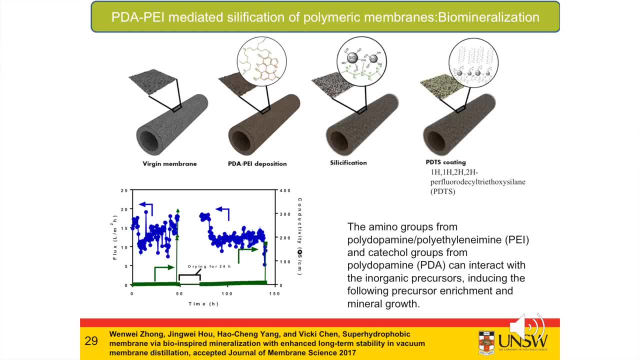 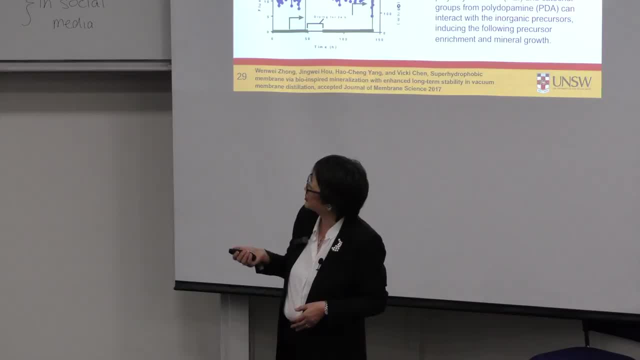 polydothamine to produce catechol groups on the surface. that interacts with inorganic precursors such as silica. we can then functionalise those with, with fluorosilane, or we can also get super hydrophobic surfaces that way. So it's. 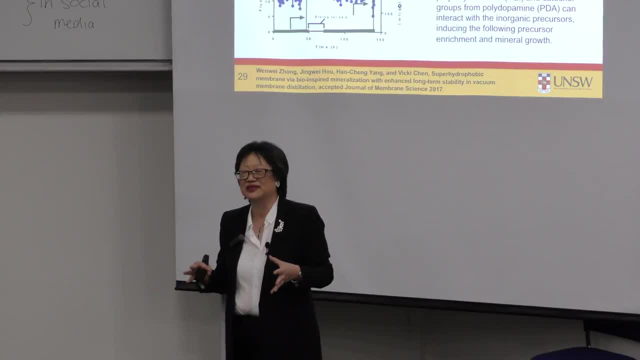 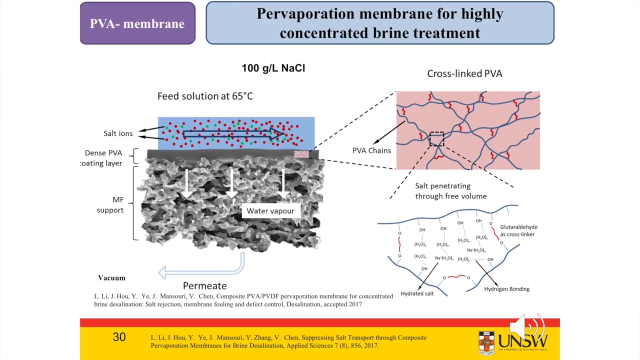 another way of saying: you can change the architecture and play around with giving you a much different surface without having to go to a chemical grafting or covalent bonding. Now the challenges of working with brine. as I said, 100 to 200. 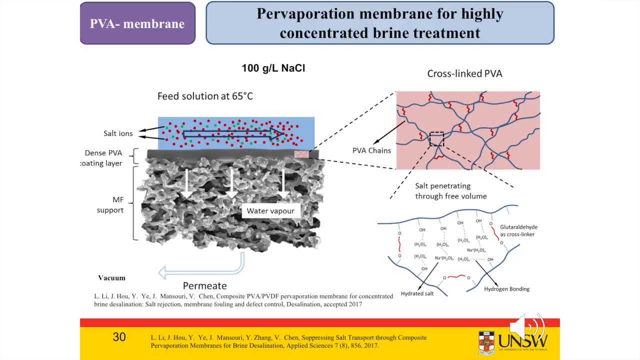 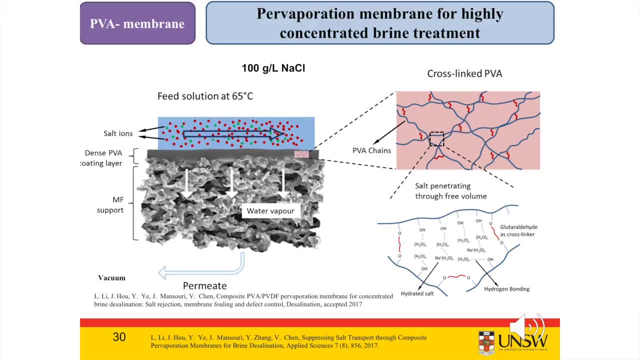 diluted, highly diluted, highly diluted components. if you are working with a lot of calcium, another divalent, that eventually those crystal- you can see the house of purely those crystallisation processes can foul the membrane, can actually then wet the membrane. So one of the things we consider is if 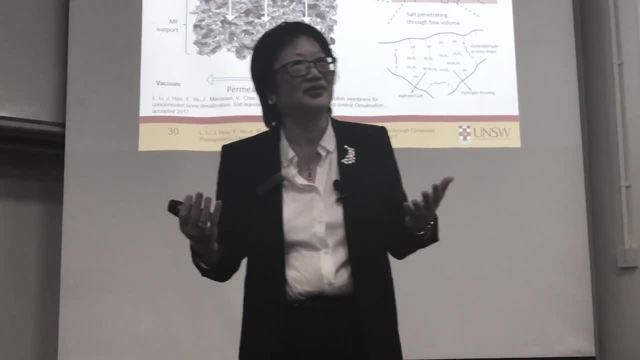 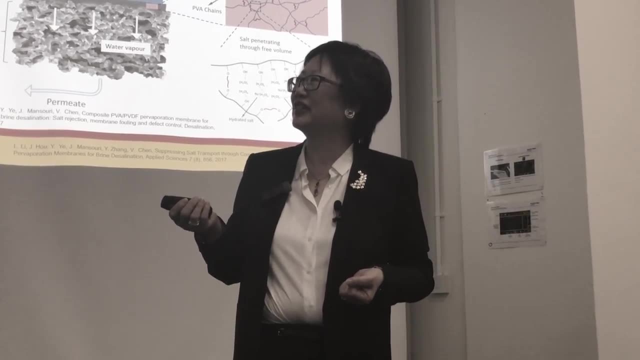 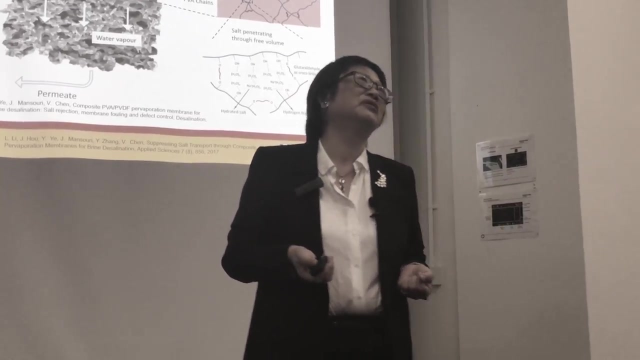 we wanted to protect the membrane. let's just go all the way to the dense film surface And in fact what we have is we coat the membrane with denso. here is polyvinyl alcohol again, and now I Like the other case. instead, we're going to use vacuum to pull the liquid water from the 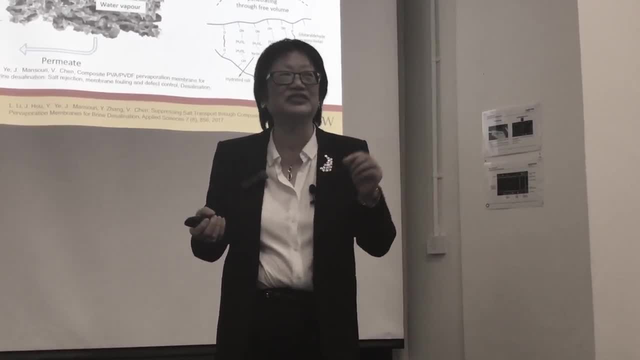 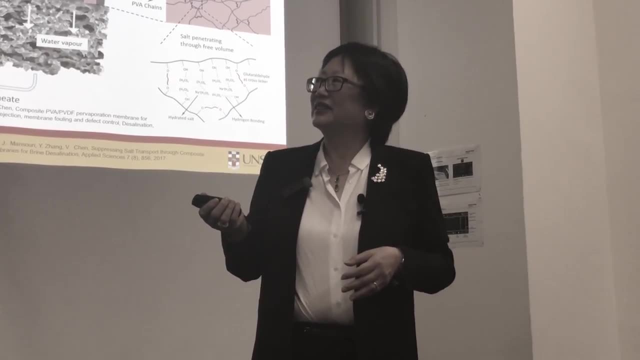 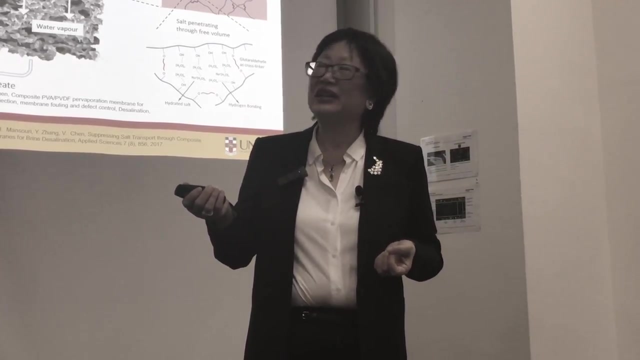 other side- Sorry, the water vapor from the other side. So we now have a solution: diffusion process, not a water vapor transport process. Now the same principle in terms of using a hot feed- 65, but we are working as I say. 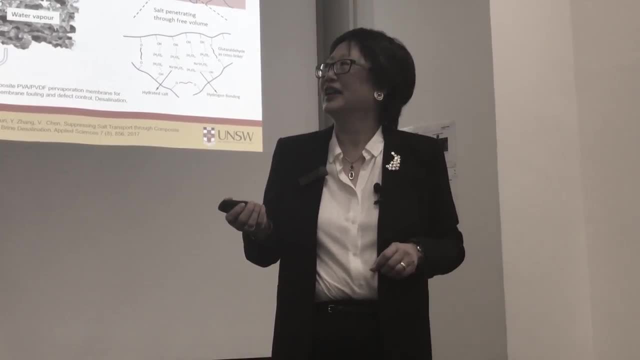 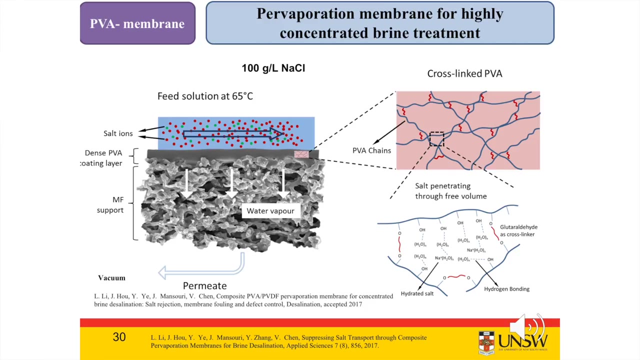 quite challenging concentrations: 100 grams, 200 grams per liter. So this process for evaporation has been around for a long time, but most people use it for dehydration of organic solvents. Here, basically, we're absorbing water from the hot feed and then, at this interface, vaporizing. 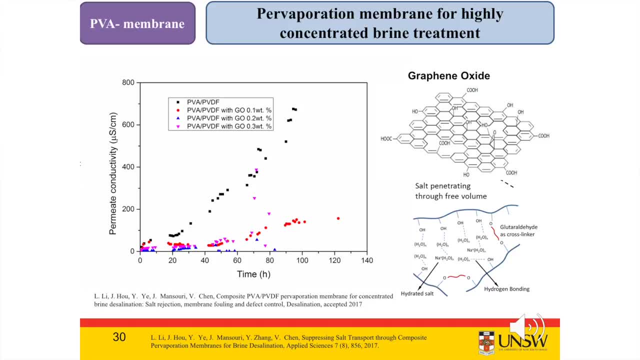 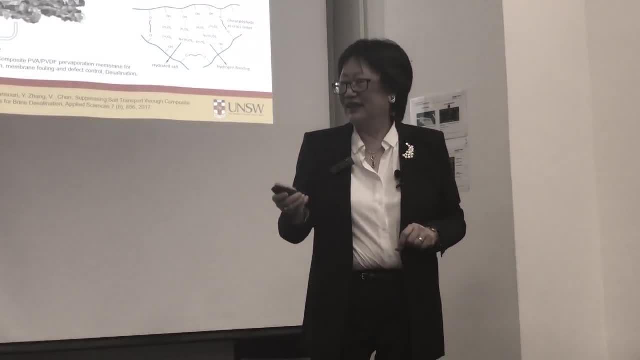 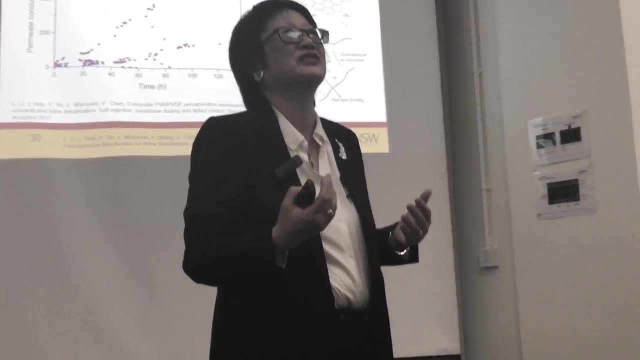 Now we found that even with a dense film with crosslink polyvinyl alcohol, we were still getting some hydrated salt actually diffusing through. So what we did was actually say, well, can we put other barriers? We might compromise the flux, but can we put other barriers to kind of rigidify those polymer? 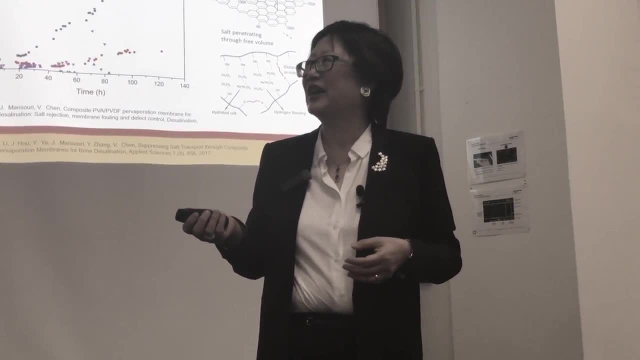 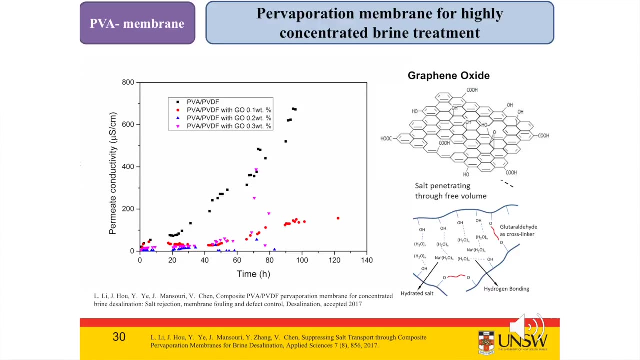 chains. So we added graphene oxide and, surprisingly, rather than just simply dropping the flux, we didn't get much flux drop. But in fact what we did was we got suppression of the salt migration which is- and this is at not perhaps up to 10% of the sorry- only 0.3 weight percent in the in the in. 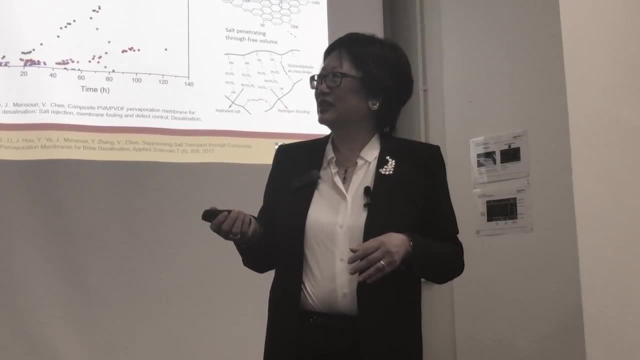 the, In my opinion, in the material that we add to it. So we thought that was because we've got this carbon or more carbon, and if you kind of you know, if you add this to like or if you you know the one that we're putting. in here. that's a quite a lot of carbon. but you have to change in order to you know, really, you have to be able to go up and add in this this coating material. So it's really quite interesting when you add in, add in these nanoparteials. it's not. 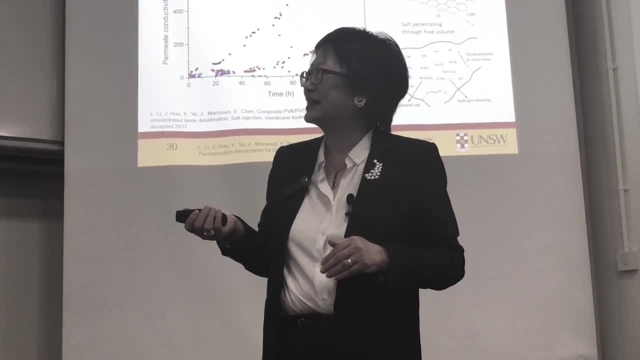 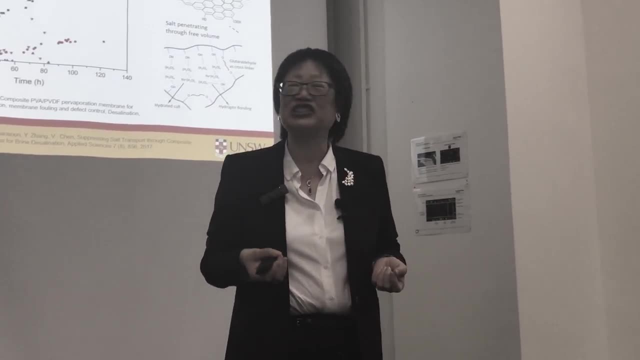 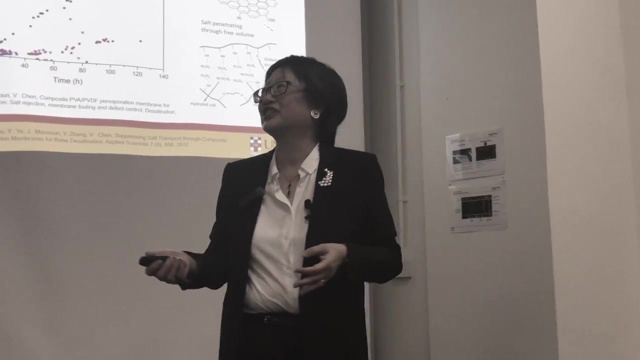 as simply they're using as porous fillers, They have some interaction with the polymers. to, as I say, basically, instead of crosslinking this with a just simply adding the more, more longer reaction times by putting a graphene oxide, you actually having, as I say, hydrogen bonding and other interaction. 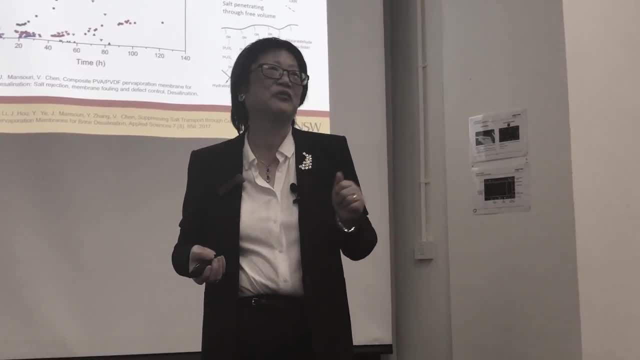 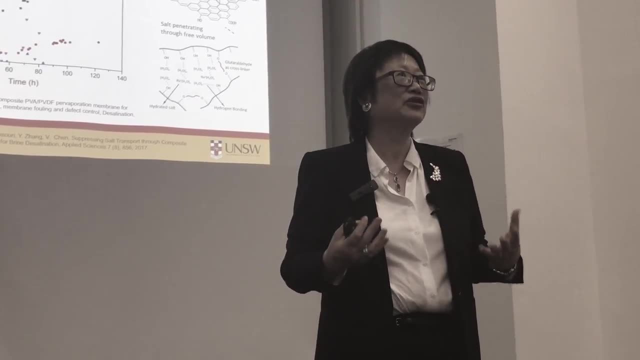 between the nanofillers and the polymer, And this is something one of the things I'll talk about is, when we think about nanofillers, think of them as just putting like a porous material. They have quite strong interactions with the bulk polymer. 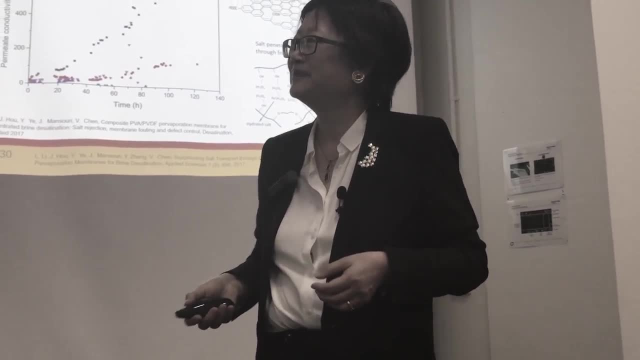 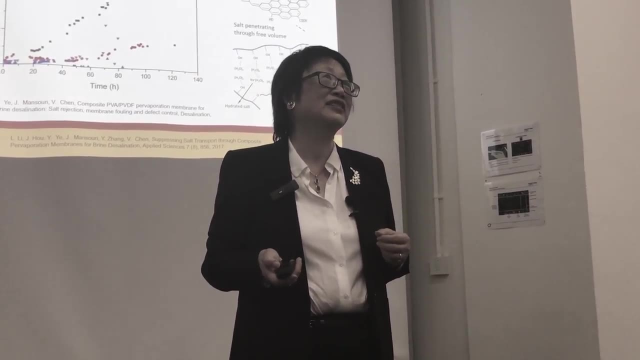 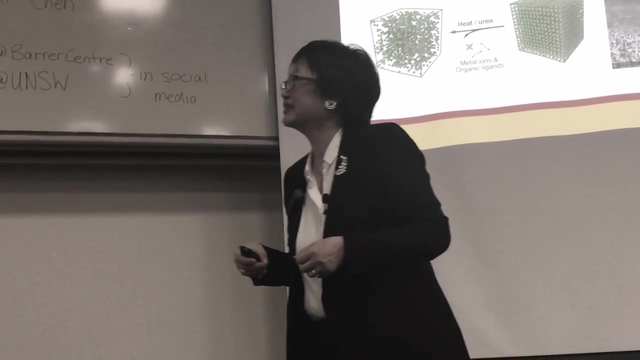 and that has some consequences that perhaps was not foreseen. So if we look at that, say, well, how else can we improve the water permeation in these particular pervaporation processes? So one of the things that we use is metal-organic framework material. 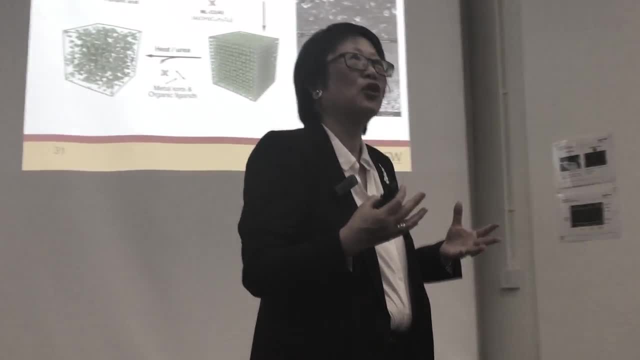 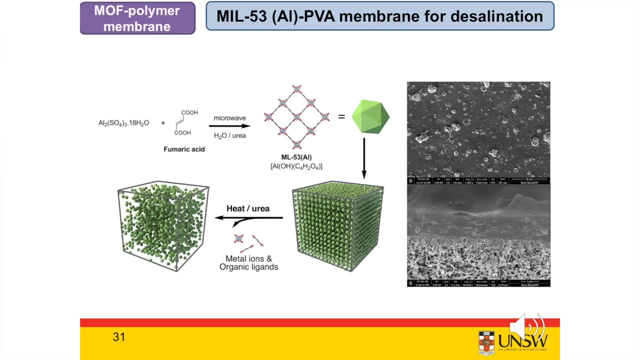 Now, metal-organic framework is simply organic ligands coordinated through metal, sorry, metal-coordinated organic ligands. Now, here we're using MIL-53, which is a fumigastic-aluminum-coordinated framework material. Now that makes a nice tight material. 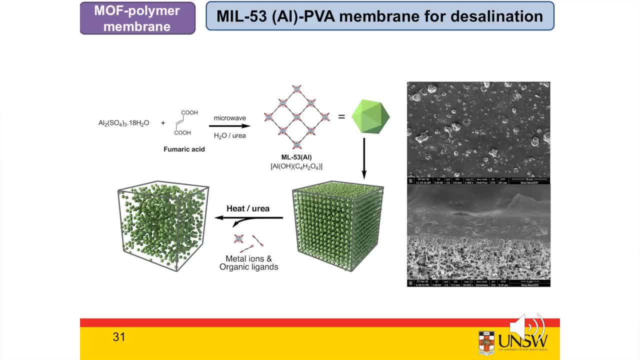 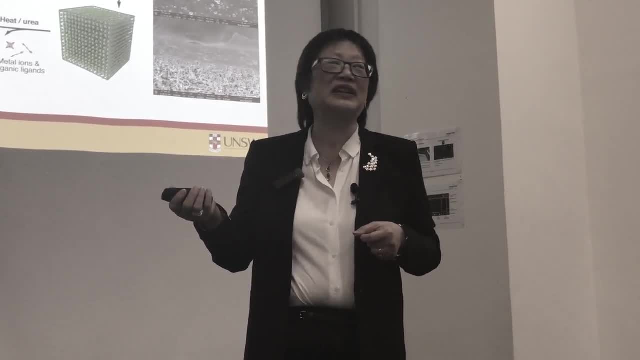 It's hydrophilic, it's iron, but one of the things is, can we actually improve on that? Because when we have a dense metal-organic framework, we have some sorption of water, but it's not a very efficient sorption of water. 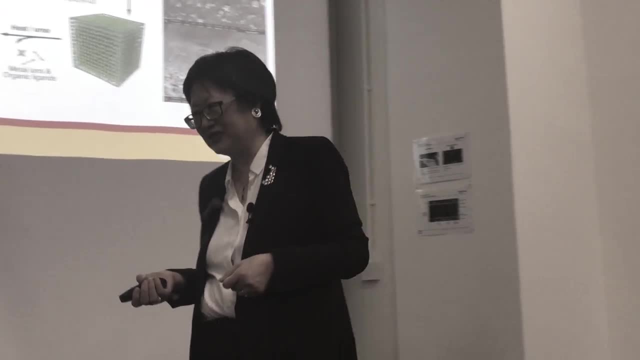 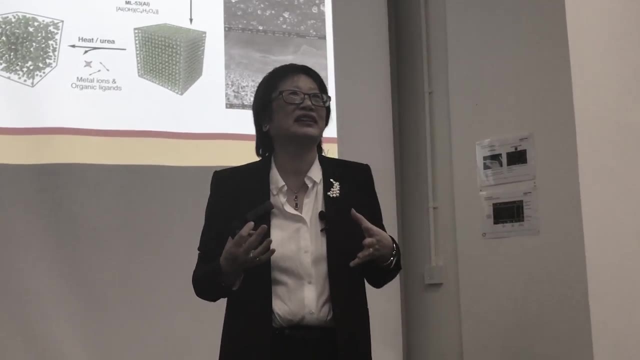 into the bulk of the material. So one of the things that we can do in the metal-organic framework areas is actually what they call defect engineering. We can etch out parts of that metal-organic framework material so you can make these pore more accessible. 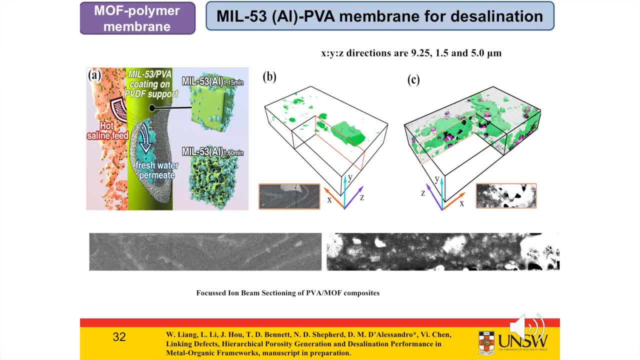 And you can, using urea heat in this case. so we found was you can actually section the untreated material. We can find that we have in fact quite dense patches of metal-organic framework, but and then here we have the defect engineered. 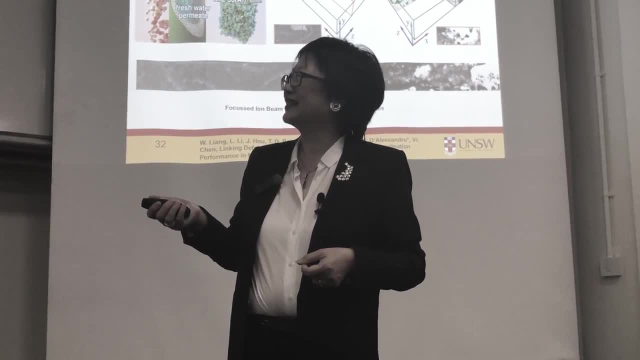 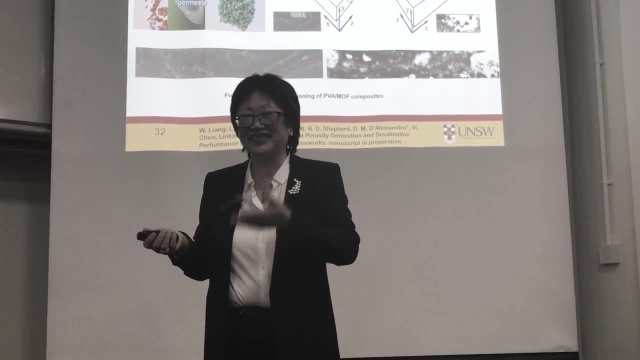 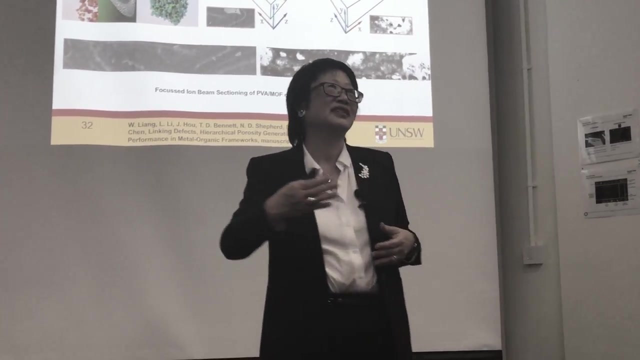 basically with the moths in the green and the voids in the purple area. So one of the things is we use- I'll say result just fresh off the shelf two days ago- is using focus ion beam to allow us to section those particular material, to show us the distribution. 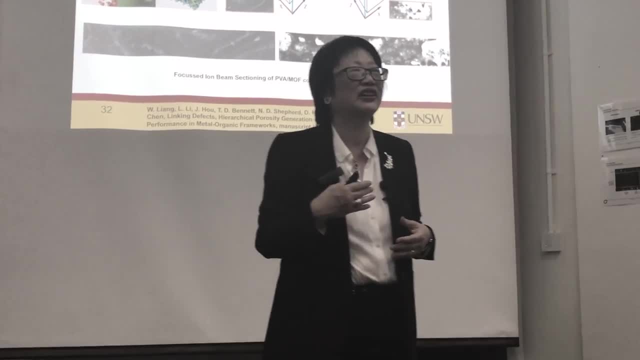 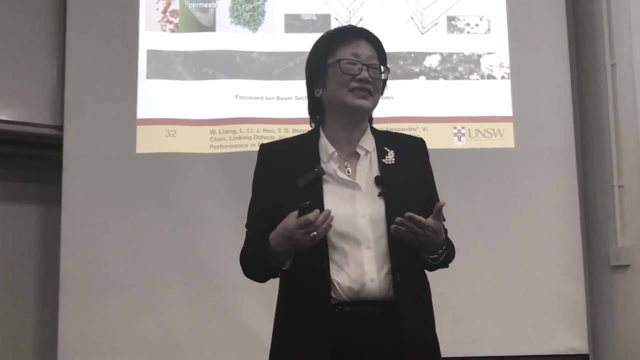 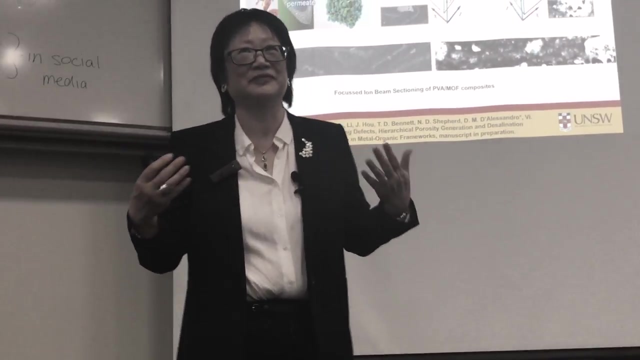 and the density of those materials in that polyvinyl alcohol. So what we found is when we put these sorts of material in, we can increase our fluxes for 30 to 50%. So the presence of that defect engineered material allows us to improve not just the permeability. 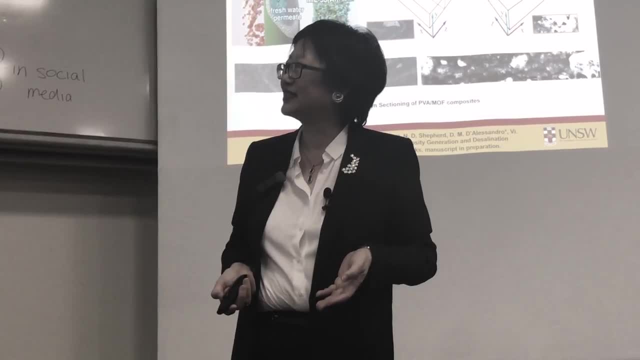 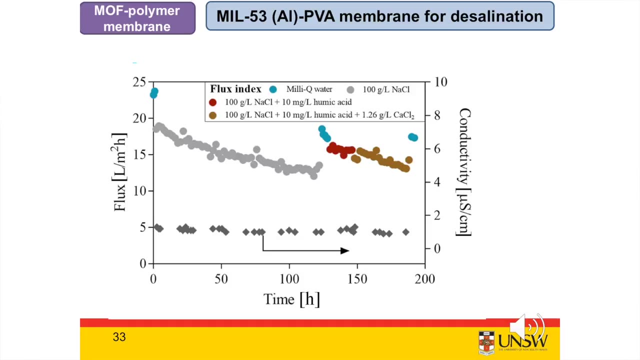 but in fact we get in fact ability to suppress the, the salt process. So are these things robust? One of the things that people have concerns about metal-organic framework is they are- can they stand up to water resistant, sorry? 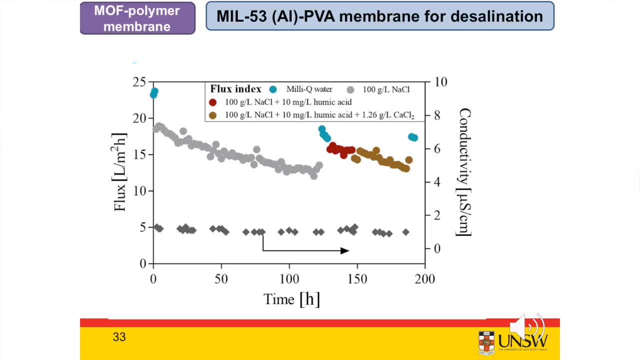 not water tolerant in terms of stability And what we can show you here, that we were actually running about 150 hours and we are using 100 grams per liter of salt and with the presence of humic acids, presence of calcium. 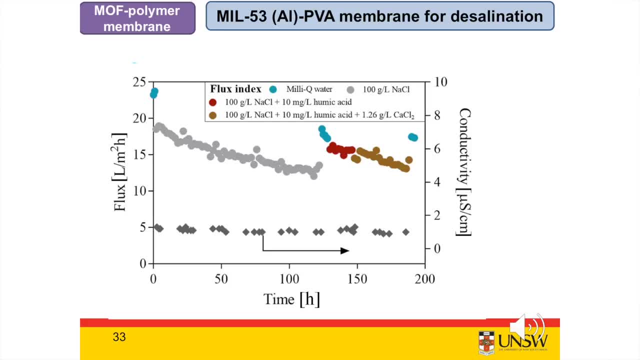 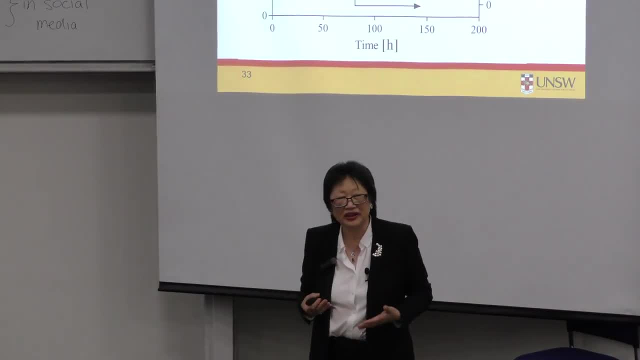 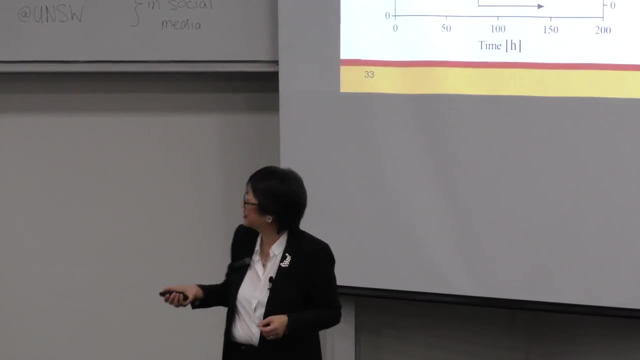 we can wash this membrane and we can get recovery and the flux declines because we're concentrating continuously, concentrating the feed. but it is actually quite a robust system. And I said we're looking at very, very high salt concentration. So you can look at the conductivity. 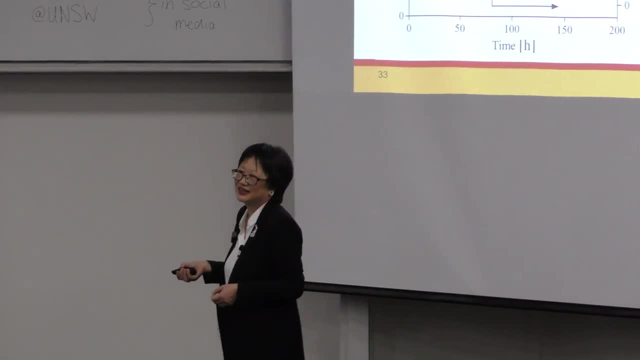 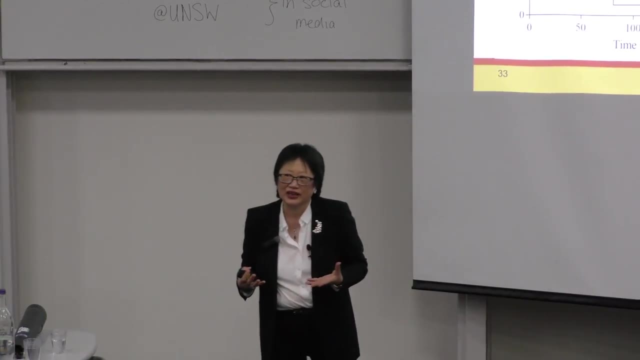 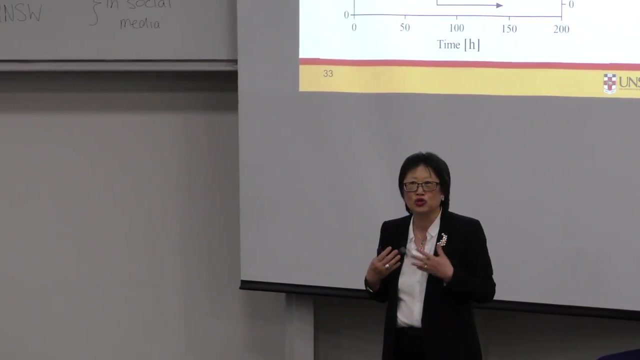 it's ultra low conductivity and you do not often see that kind of salt rejection with these sorts of types of membranes. So this shows you the strategy that, in fact, when we think about treating brines, the challenges of scaling and trying to drive, 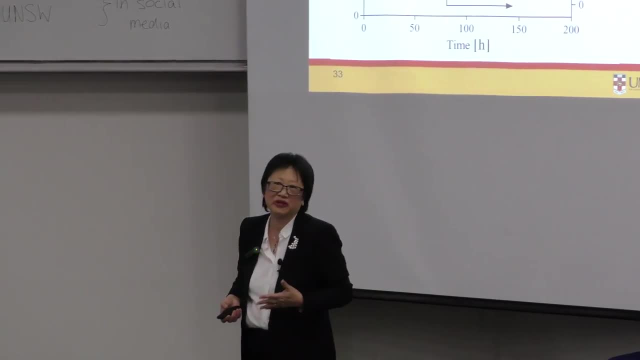 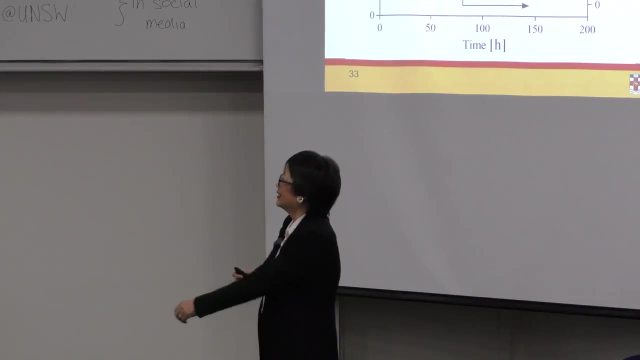 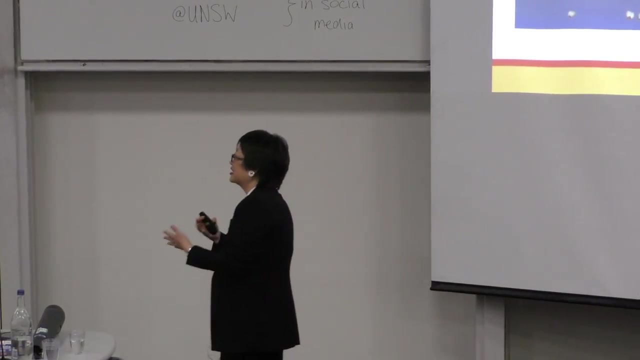 to the point of crystallization requires. we have quite robust membranes and here's perhaps a generation of membrane that can actually be able to tolerate that kind of challenge. So some of the areas of working on in the ongoing I don't have time to cover. 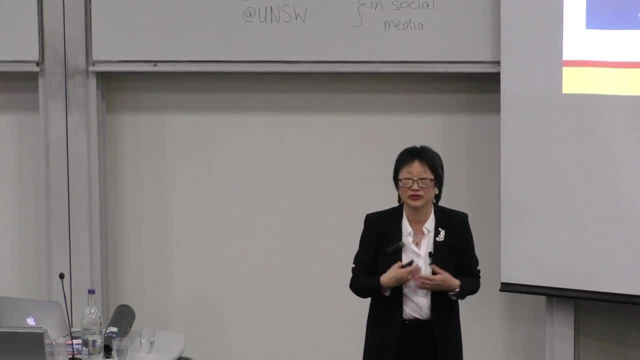 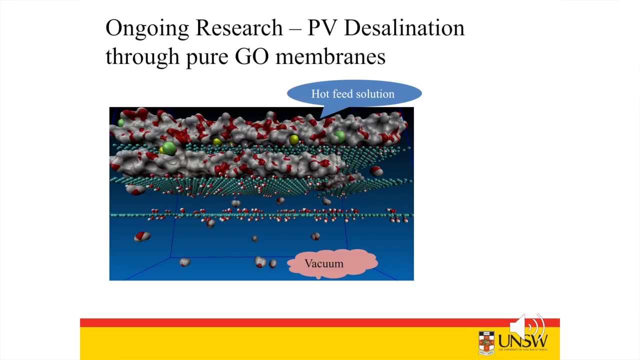 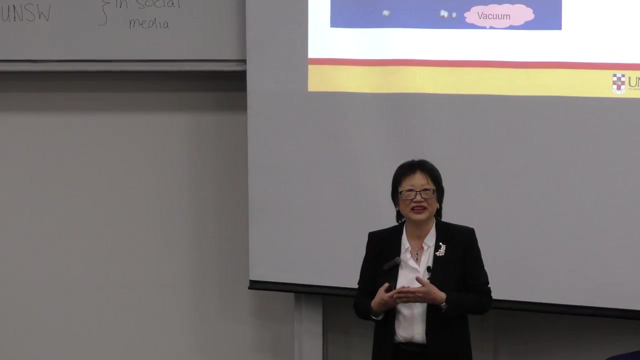 is really to compare these against pure graphene oxide membranes for pervaporation. Graphene oxide has really interesting transport properties in terms of in the hydrated form, but when we put them in a pervaporation situation, we have a combination of vapor transport as well as a swollen graphene oxide layers. 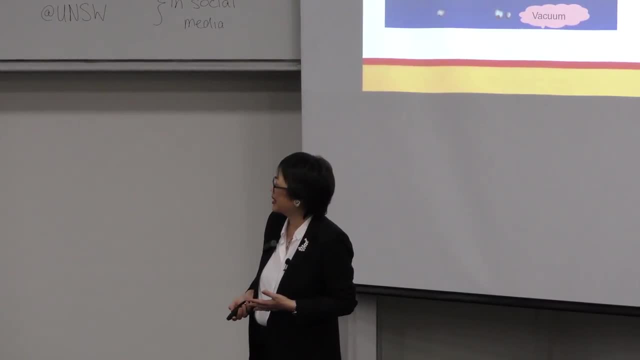 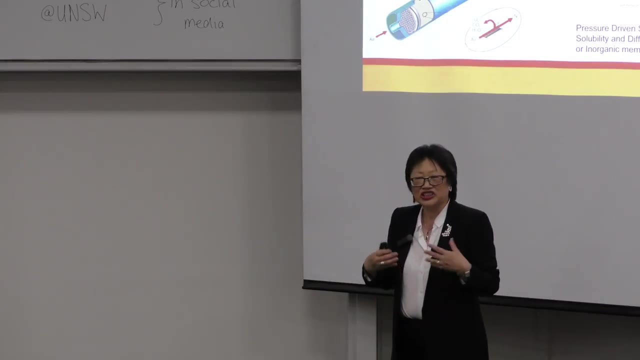 So one of the things that we are looking at now is looking at what are the mechanism, potentially, of that transfer from liquid phase to the vapor phase. So I'm gonna switch gears a little bit now and talk about our work in gas separation Now, just to give a little bit of background. 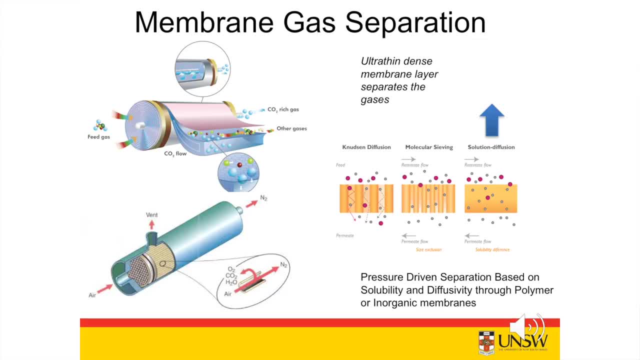 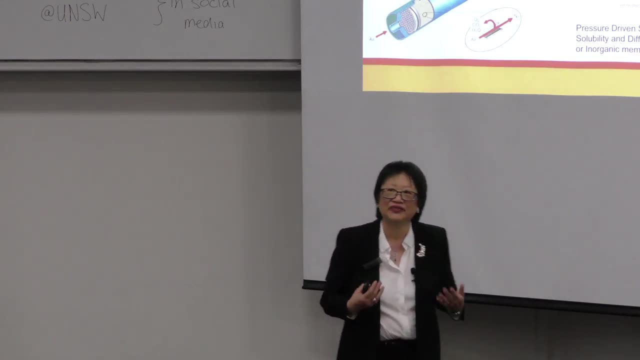 you think about membrane gas separation pretty much driven up. we're looking at pressure-driven gas separation, typically in hollow fibers or SPAR rounds or conventional modules, And most of the gas separation is in the solution-diffusion approach where you have an integrally skin membrane. 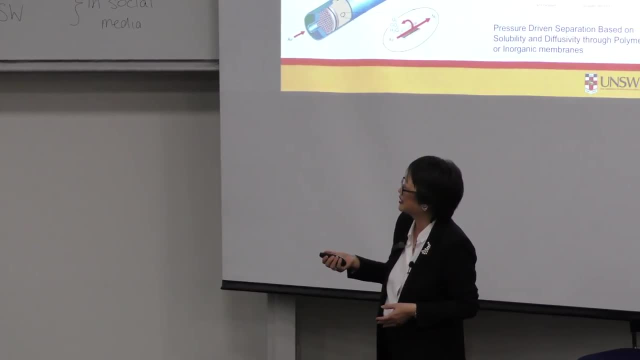 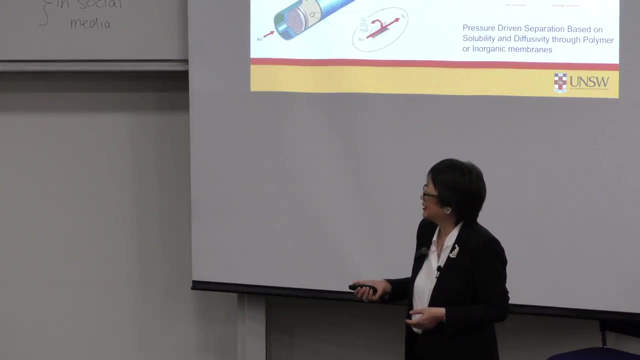 very tight, ultra-thin membrane separation with a porous or super-thin membrane separation, And you can see that there's a lot of pressure and a lot of support to give you the mechanical strength Now these materials can be, of course, 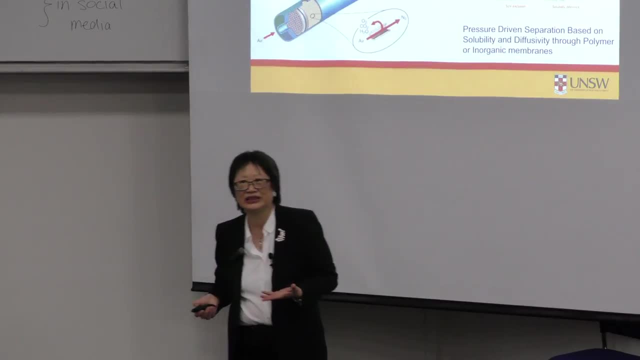 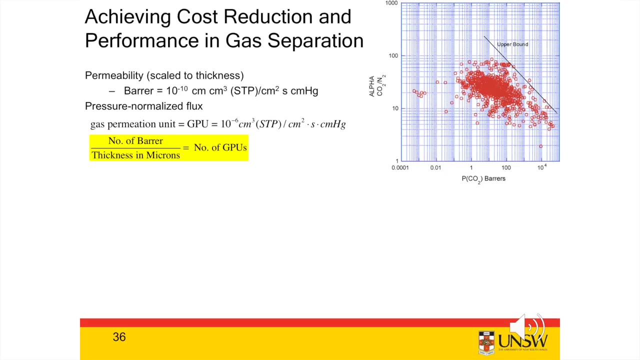 both polymer and organic materials. but we'd like to say: can we actually achieve the best of both worlds? Inorganic materials have issues of brittleness and also cost. Polymeric materials are limited by the solution-diffusion mechanism. So if we want to achieve both, cost reduction. 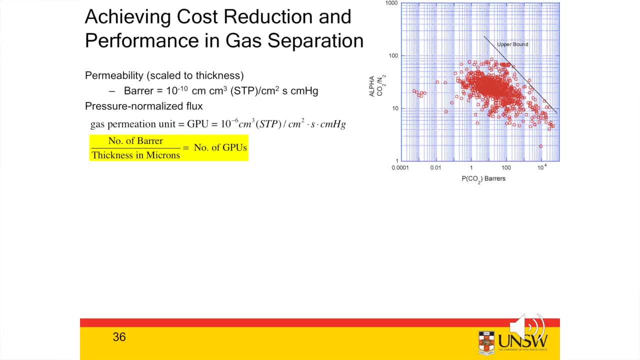 we need to have the right materials, but we don't need to have a very high cost reduction And that's why we're looking at the material aspect, The permeability, which is materials aspect, and the name lecture comes into defining the permeability of the materials. 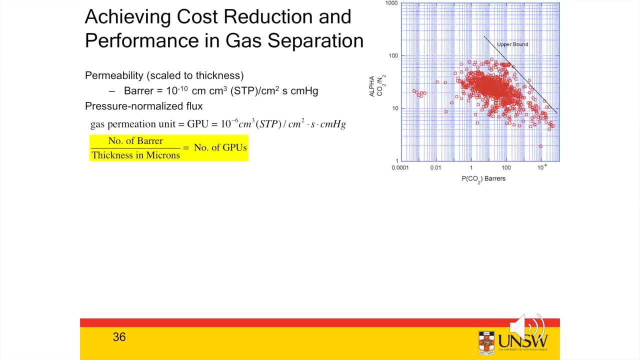 but that's actually scale to thickness. But what we really want in terms of productivity, we want the pressure normalized flux which is actually in gas permeation units, polymeric materials in the solution diffusion mechanism. it basically line up, roughly controlled by the relative permeability and selectivity. 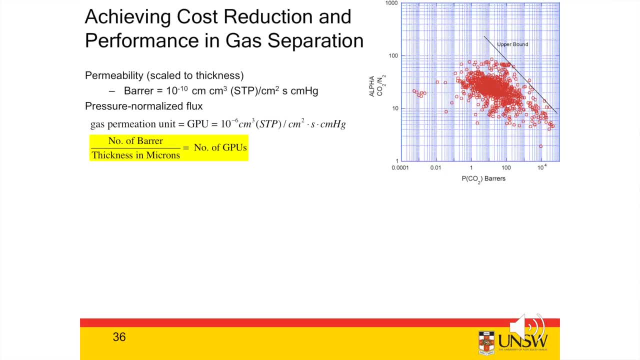 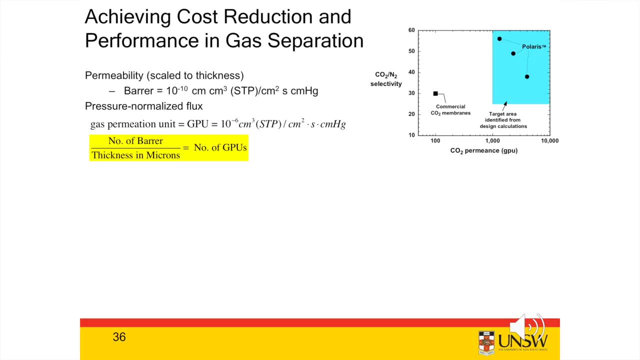 But we really want to think about in terms of application and cost is basically the selectivity and the permeance, which is the productivity, the flux of the membrane that you can achieve. There's been a lot of work looking at what is the optimal flux and selectivity. 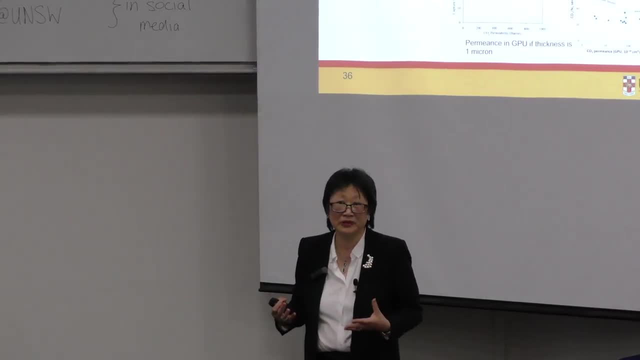 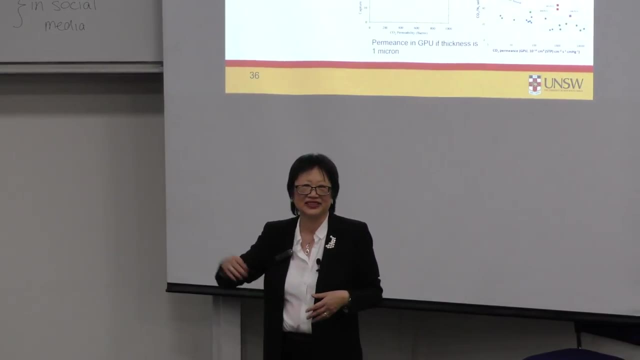 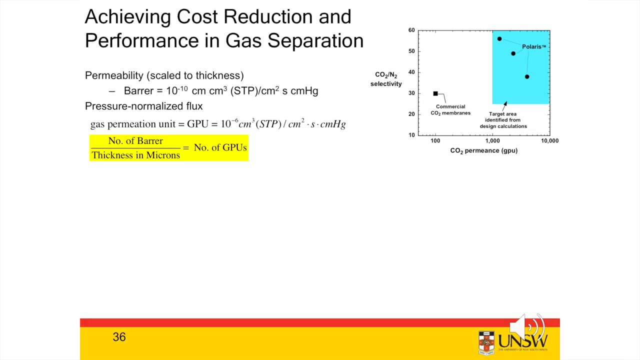 because even if you get too selective, it becomes a problem in terms of designing the module design and the process train. So it's not simply saying that we want complete, huge selectivities and huge permeability simultaneously is going to answer all your problems. So there's people looking at: well, what? 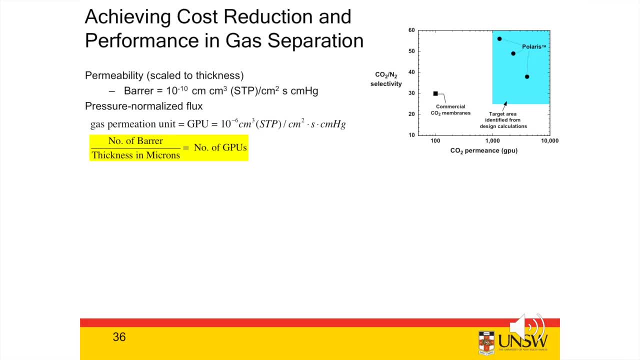 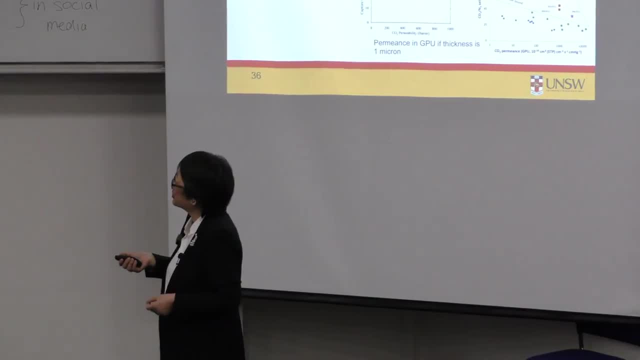 are the areas of interest. So the areas that are in probably are in about the 40 in terms of CO2 nitrogen selectivity if you're looking at treating things like flue gas And the permeance is probably a little bit around the several hundred thousand GPUs. 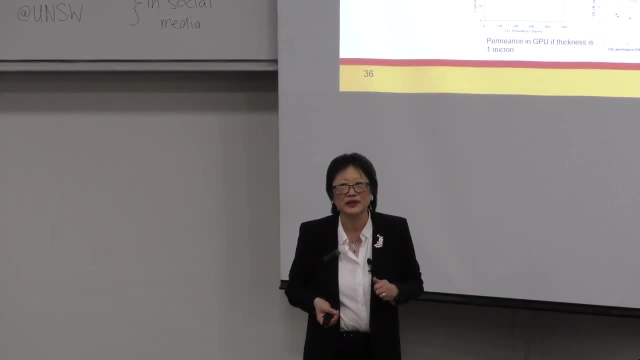 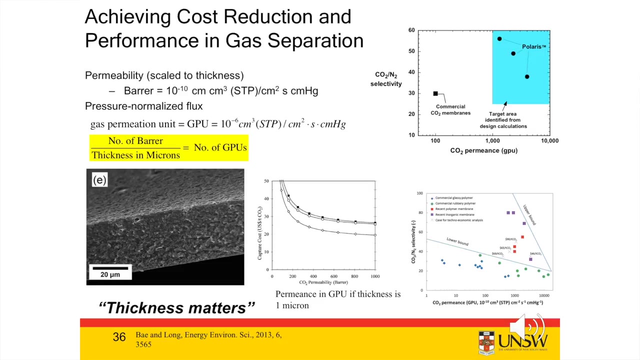 Now this has been done in some respect in flat sheet membranes, but it's been actually quite difficult to do in hollow fiber membranes. So my takeaway here, which I think will answer, is: thickness matters, because many people talk about permeability- wonderful materials of permeability. 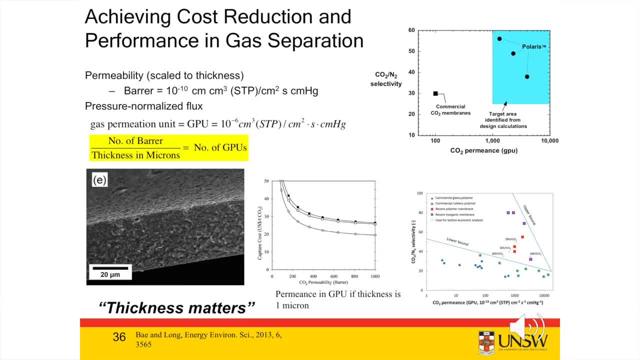 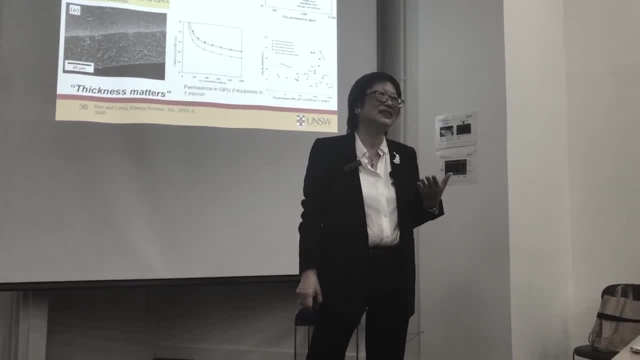 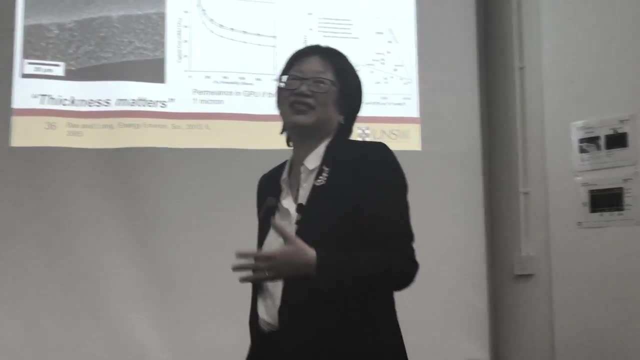 but they can only make it in 100, 200 micron thicknesses, So in terms of practical productivity it's extremely un-economical and difficult to scale. So thickness matters when you think about how we can get that thickness down with using a material that is cost-effective and scalable. 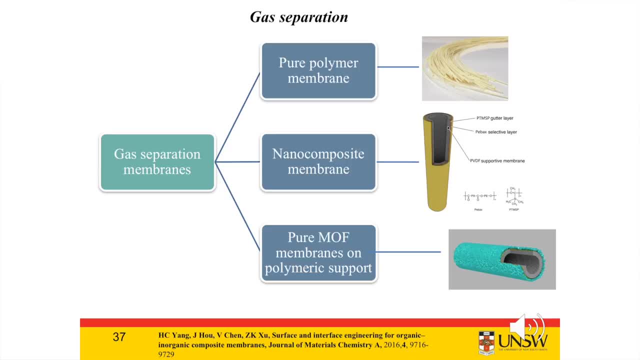 So the approach that typically people use in gas separation is, of course, pure polymer materials: spinning so you get the ultra-thin, ultra-tight selective layers. We're going to talk about nano composite material, which is basically using a list laissez-faire. 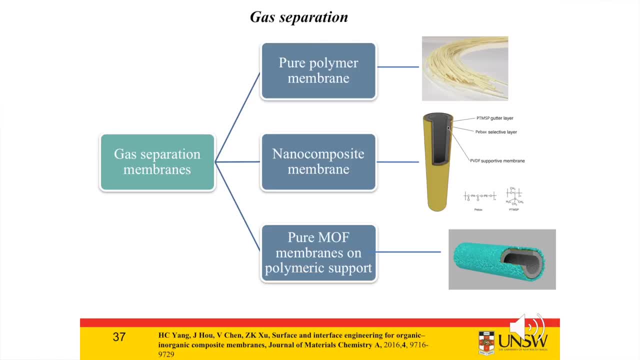 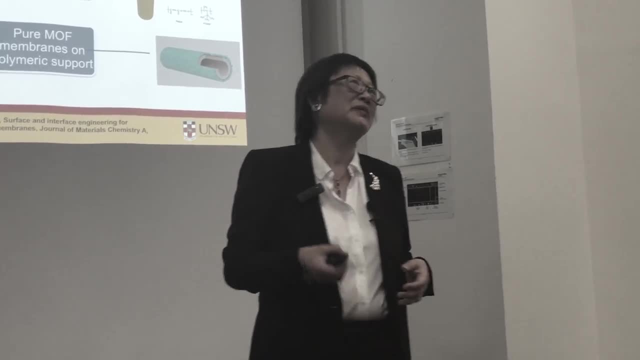 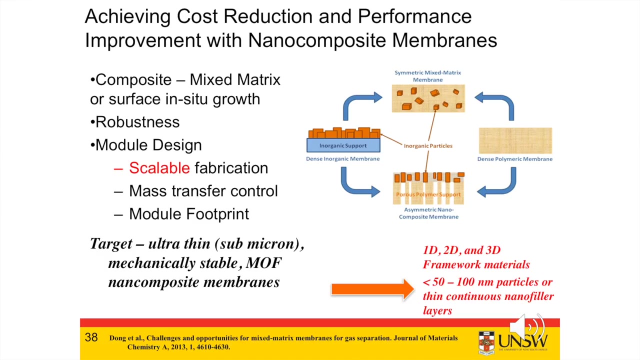 support allowing us to use much more mechanically weaker material but maybe much better separation processes. and finally, I'm going to talk about growing pure net organic framework type of material on top of a polymer material. so we talked about, as a reducing cost and increasing importance, the conventional 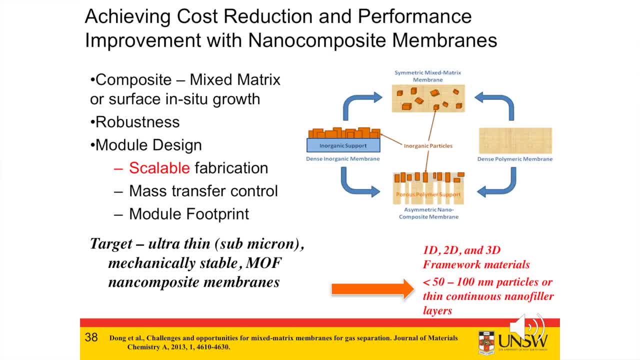 ways to think about is: take your dense polymeric, we add the inorganic material or the, the other nanocomp materials, and you're using basically chunks of that material, and I would I call this the the chocolate chip cookie. you so you get benefits of the nanoparticles or inorganic material, but you don't 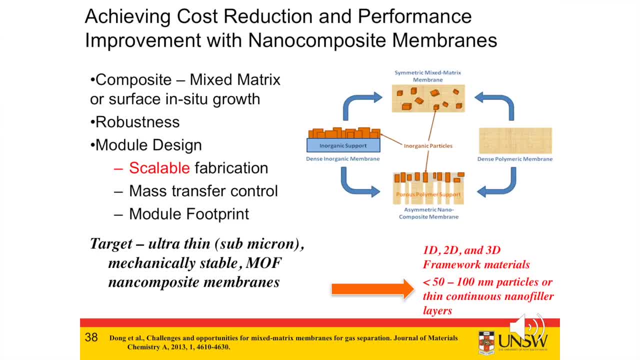 necessarily get all the benefit. you have people who grow these denser metorganic or other new bit on top of a dense inorganic material, but often that they can be quite thick and again, but it's a much more rigid support so you get a good balance. but what we really would like to think in terms of costs, can we? 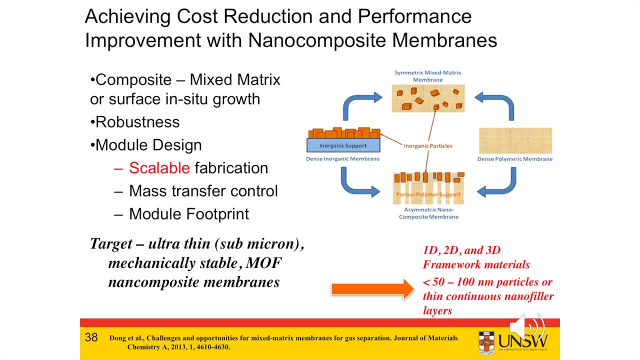 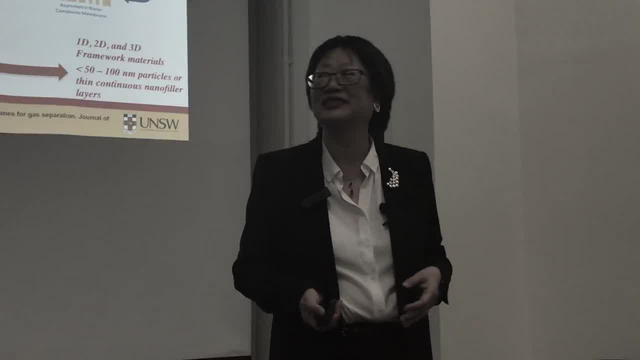 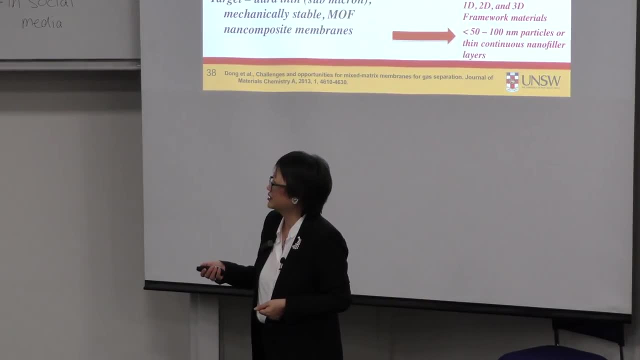 actually have an ultra thin layer where those nanoparticles are confined to a very thin separation layer and use a microporous support to give you that mechanical stability. so we're looking in terms of robustness, but we also look about scalable fabrication, mass transfer, control and the module footprint, because 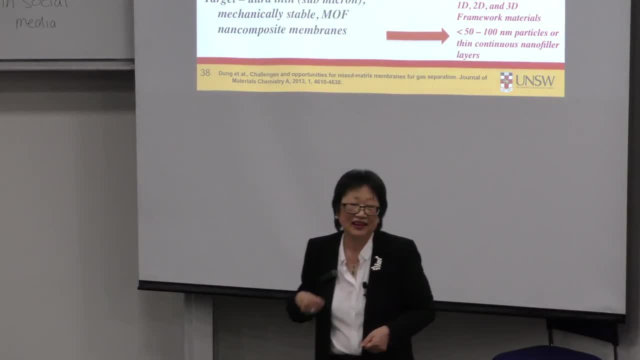 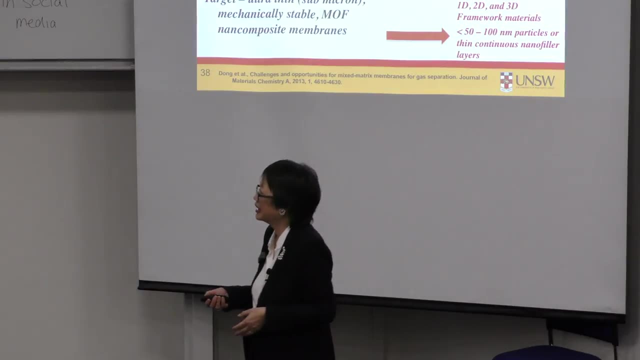 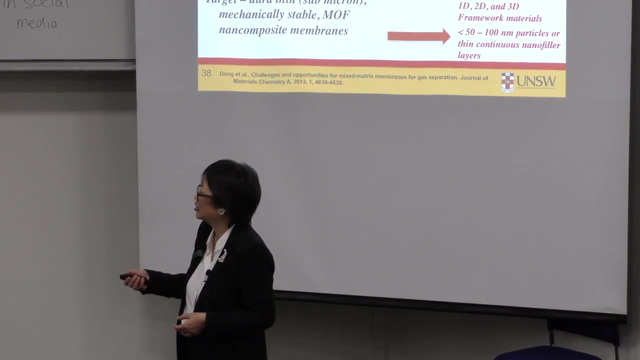 the membrane material may be only 10% of the cost of the whole process. You think about modulization. the headers, the pumps, the pipework will probably swamp the cost of the membrane materials itself. So this is quite important in terms of the whole membrane module cost, not just simply. 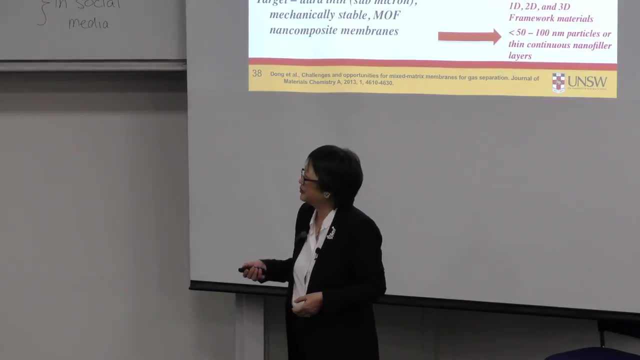 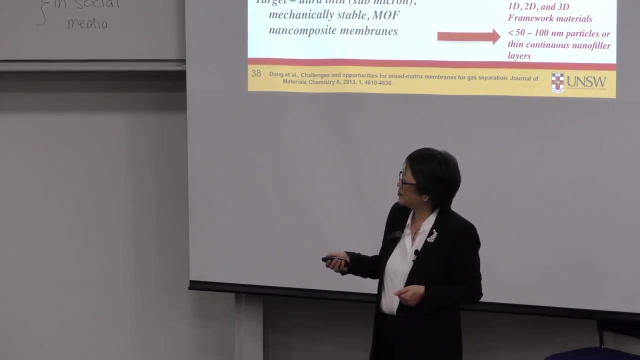 the membrane cost. So in order to get that ultra-thin layer, we really need a submicron, mechanically stable MOFs or other nanocomposite materials, And that means looking at 1D, 2D, 3D material in the very small particle size or confined. 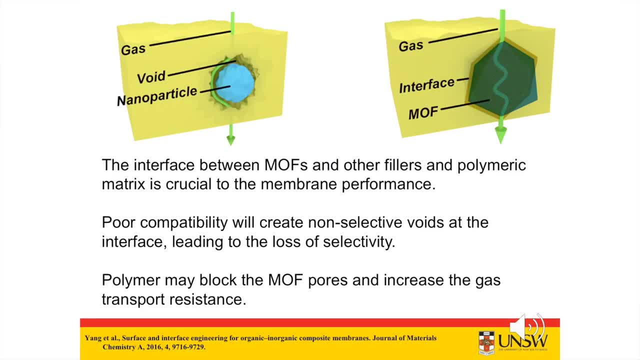 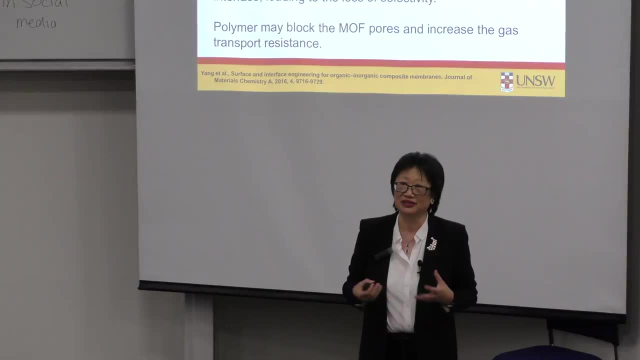 into very, very thin layers. So one of the other challenges any time you add these nanomaterials is that you've got issues with voids and forming Compatibility is really important. Potential blockage of the interface, for example in the mineral organic framework materials. 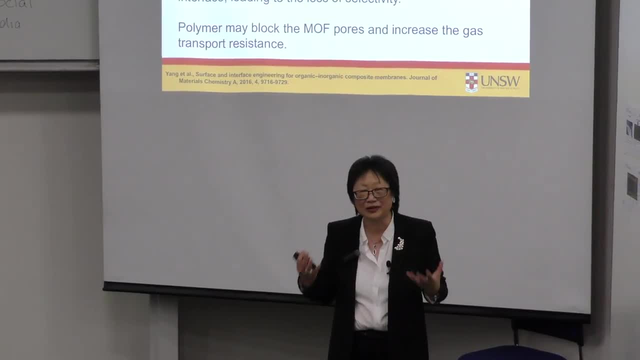 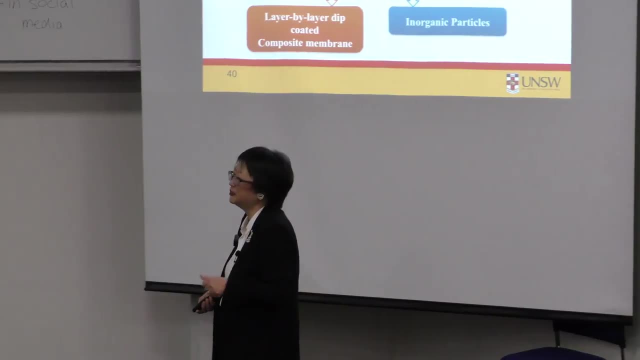 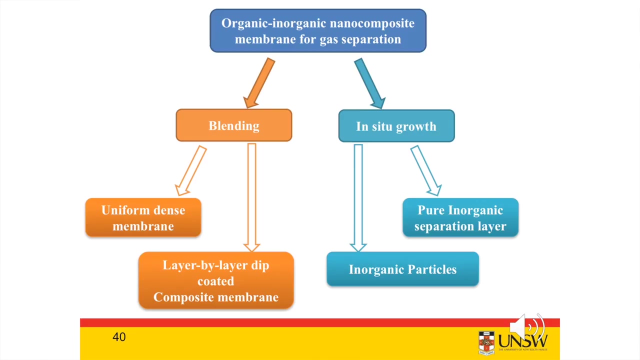 is also a concern, So we need to think about compatibility, Modulization of those materials as well. So today I'm going to talk about looking at a couple strategies we've used and to give you slightly different types of membrane: nanocomposite membranes for gas separation. 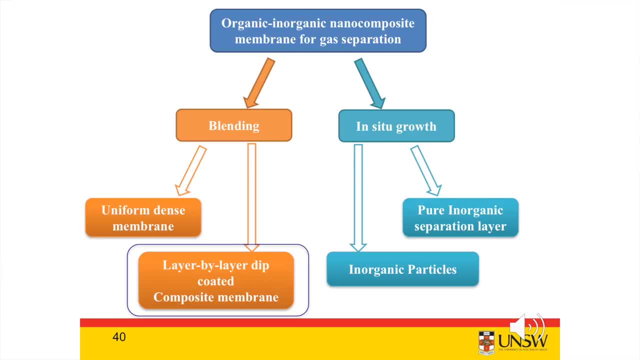 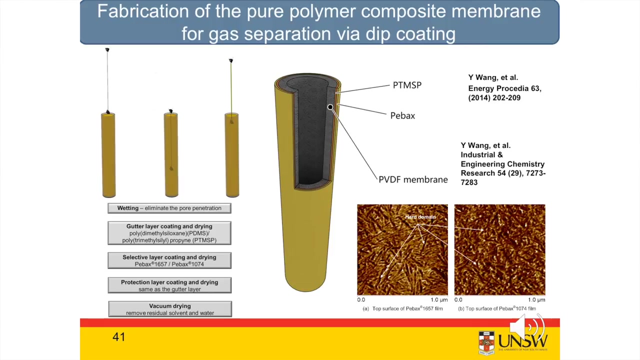 One is to look at layer by layer coatings to give you that ultra-thin, scalable membranes. The second is: are there strategies we can grow inorganic layers on top of the membrane structure and still get that gas-seving performance? Now, in terms of composite membrane, it's really a very simple. it's taking basically a porous 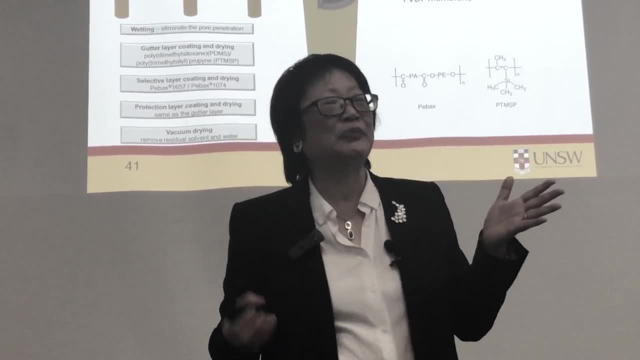 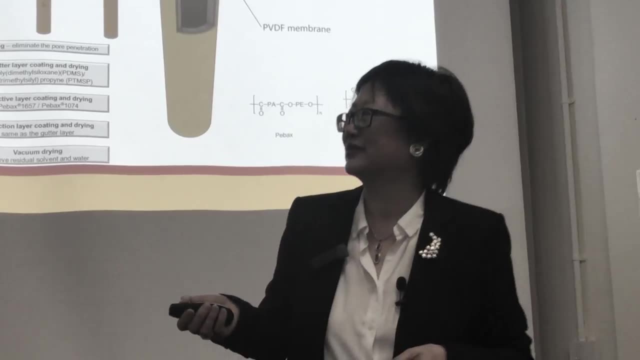 substrate and coating it with a gutter layer. Gutter layer prevents penetration of the separation layer, And what we're going to use is PBAX, which is a block coat polymer with polyamide and PEO, So the PEO has a very high selectivity for CO2.. 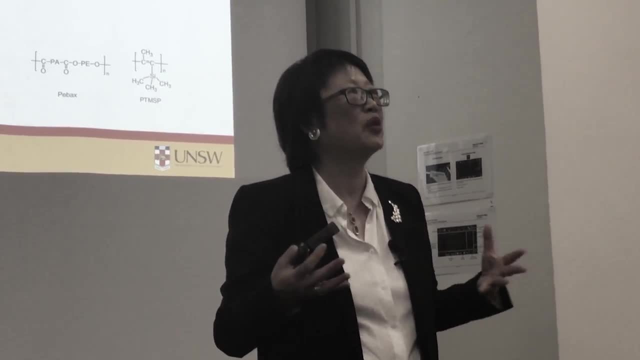 So we're going to use PBAX, which is a block coat polymer with polyamide and PEO. So we're going to use PBAX, which is a block coat polymer with polyamide and PEO. The polyamide gives a little bit more rigidity. 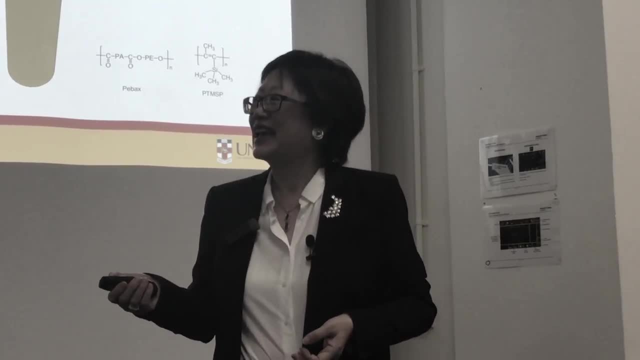 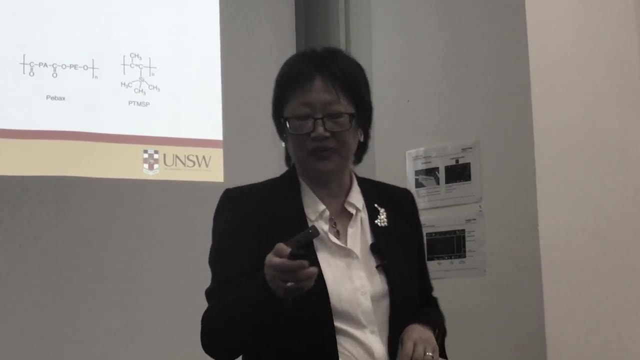 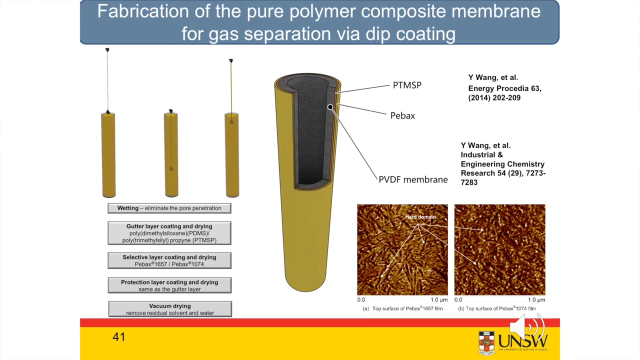 And the gutter layer we use is the PTMSP, which prevents, basically, the selective layer wetting through the whole thickness of the membrane. Now, this is quite important to think about Once we're starting to use these sort of block coat polymers. these are sensitive to micro-phase. 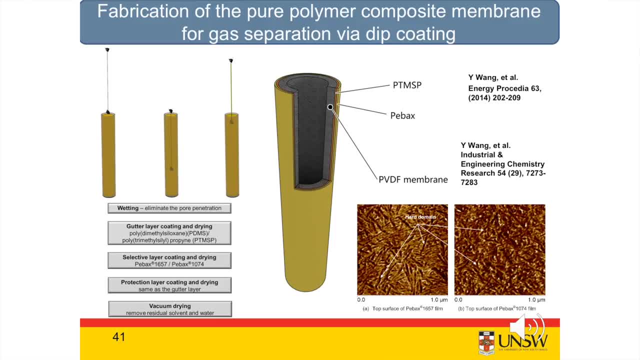 separation. So if you look at the, This is AFM, This is AFM, This is AFM. Depending on the solvent you use, the drying conditions, you can get quite different micro-phase separation in the hard polyamide block and the PEO block. 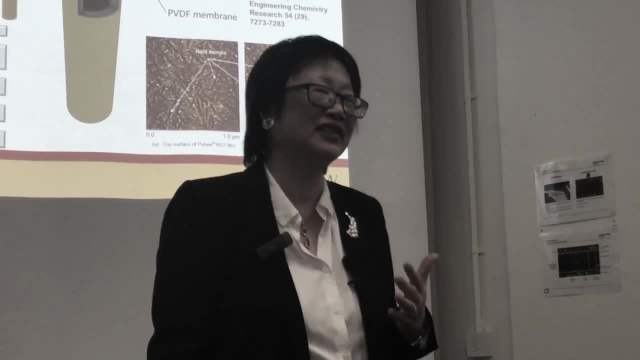 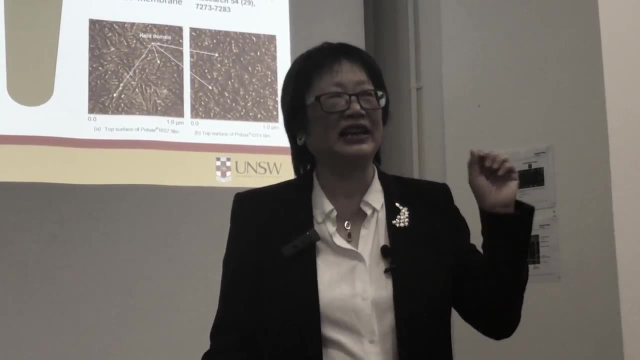 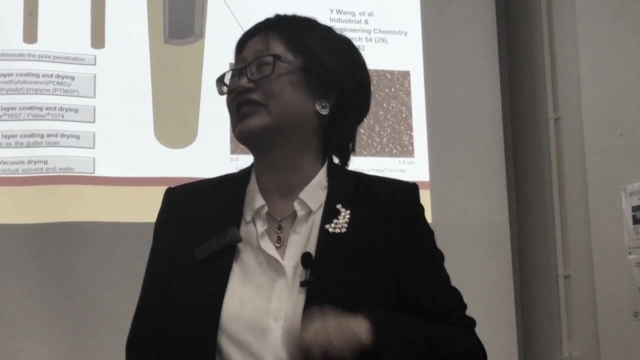 And that depends, as I said, And that can change both the separation efficiency as well as the permeation. So now, when we think about putting a nanofiller into that mix, that will also change those micro-phase separation potentially. Now, if you look at the 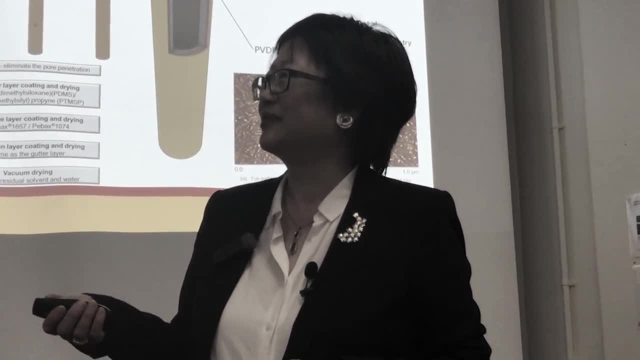 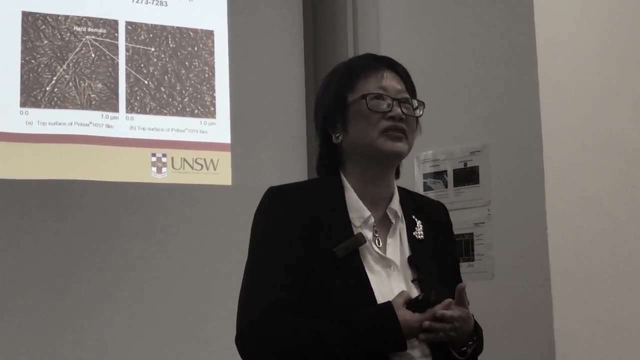 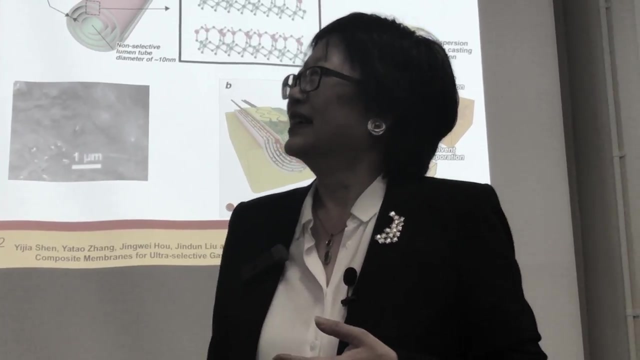 Now these membranes have quite good Polymers, have quite good selectivity on their own right. The other thing about PVAX that's really nice is that I can actually cast this out of alcohol water solutions, So it's actually quite a green polymer fabrication process. 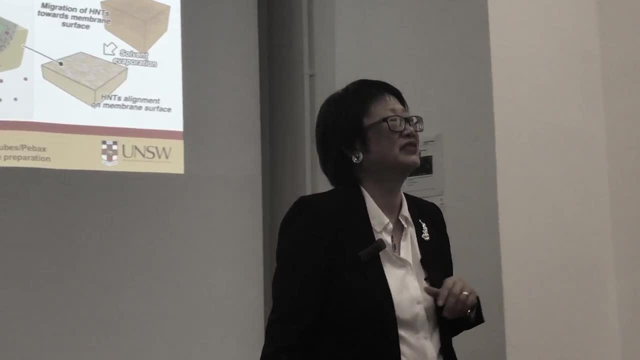 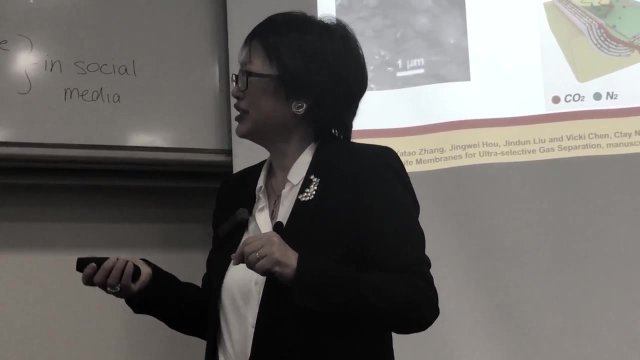 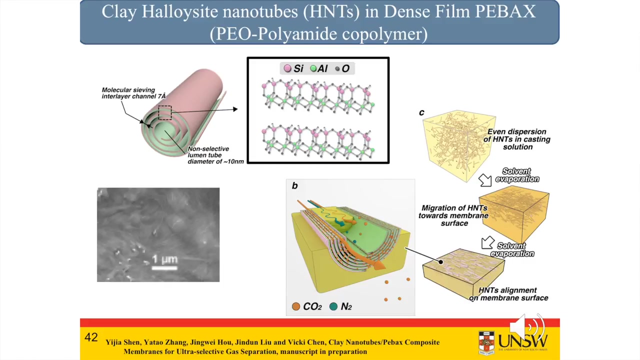 So what are the things that we can do to tweak the performance of these block coat polymers? As I said, I mentioned hollow-side nanotubes, One of the things that This is about, Basically aluminum silicate rolled clays, essentially, except they're much, much smaller. 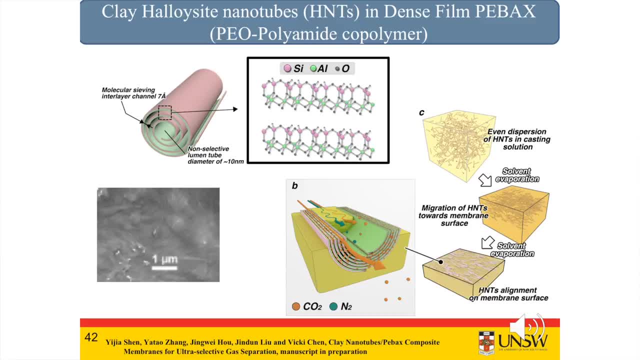 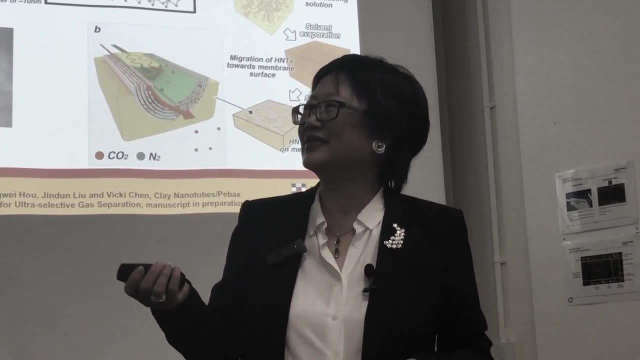 And what people found with my colleague, Professor Yatou Zeng, is when they actually suspend the hollow-side nanotube solution and they just do drop casting over time, those hollow-side nanotubes actually will migrate to the surface and form quite a dense layer of those hollow-side. nanotubes on the surface. Now these, Now these hollow-side nanotubes have interesting inter-layer spacings which can or can't. It's on order of 10 nanometers in the middle and about seven angstroms in between the layers. 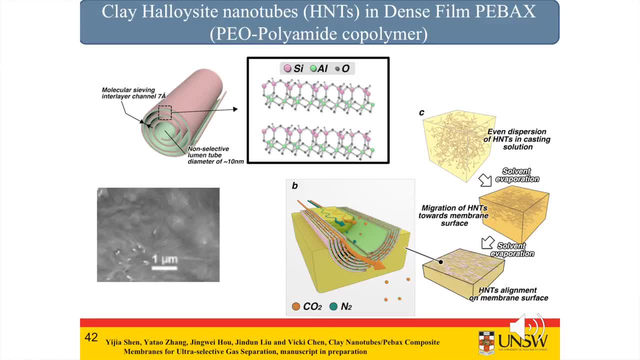 So it was in the back of my mind: well, what is the transport process? Is it through those inter-layers or you know? obviously it can't be. If there's going to be any selectivity, it can't be through the lumen, because there's a way to. 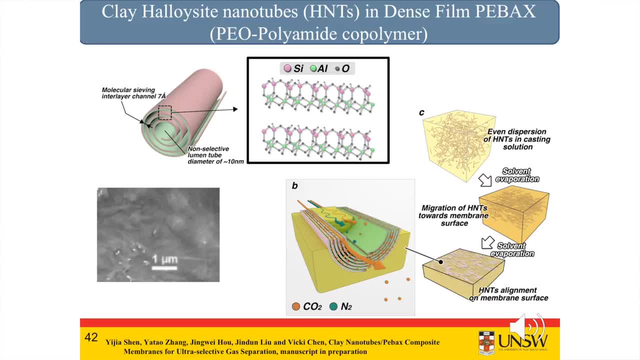 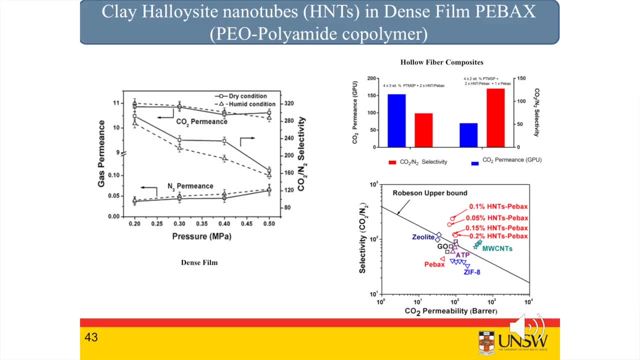 I mean it can't be through the, It can't be through the, It can't be through the lumen, because there's way too big for any selective processes. What is quite interesting is when they actually add those hollow-side nanotubes we went from. 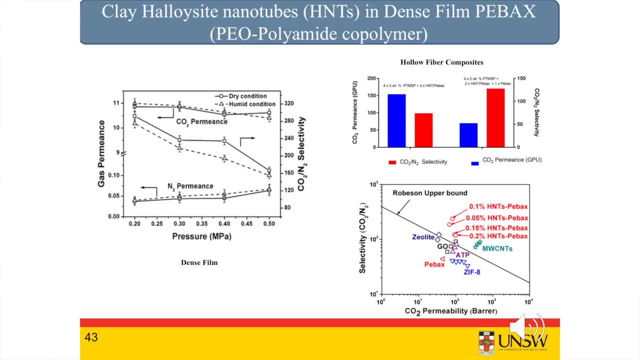 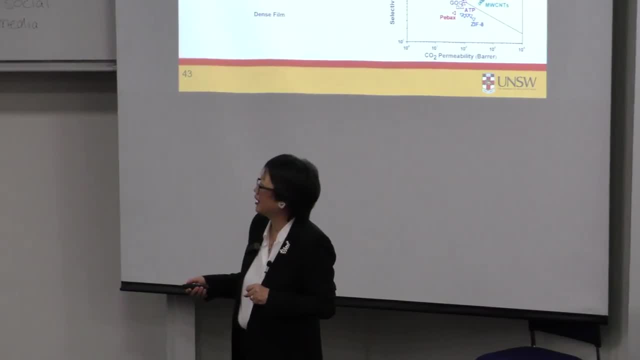 a selectivity about 40 to a selectivity of over 200, okay, Now, this is not a lot of. We're not adding a lot of hollow-side nanotubes, so this is quite a dramatic increase in terms of selectivity. 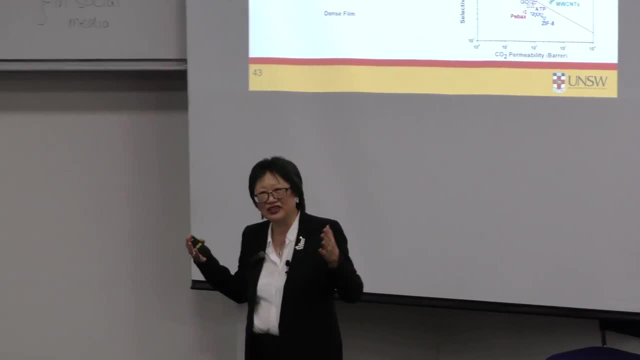 We thought, well, is it the high packing density? Is it Is, Are they, Are they, Are they, Can they actually be really characteristic? And how do they actuallyчик all those interlayers that claim that lumen silicate? 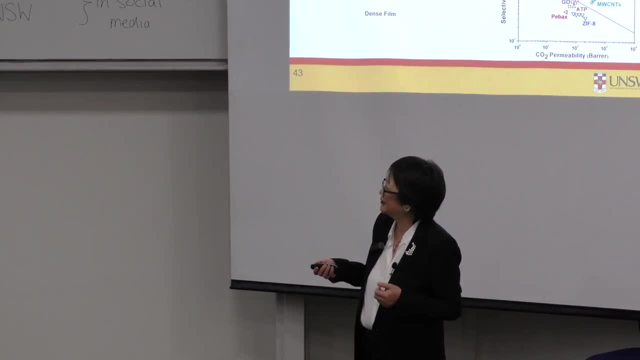 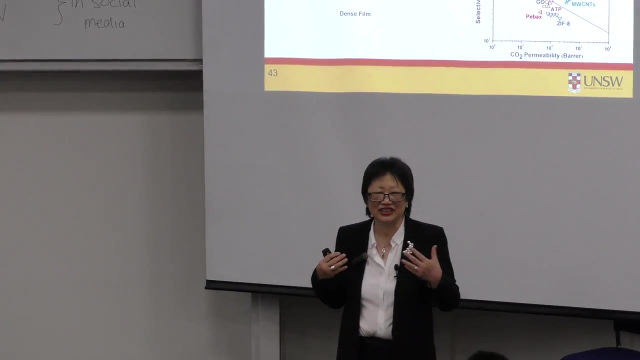 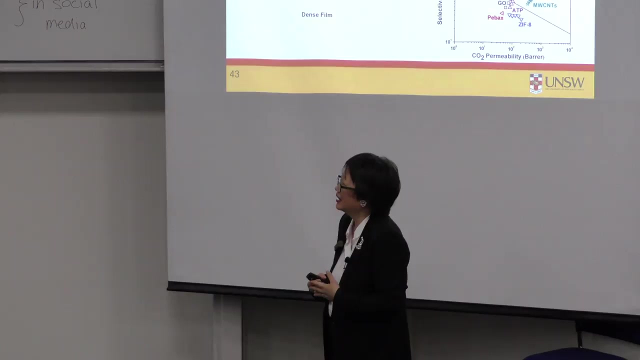 But actually when we actually disperse this hollow-side nanotubes in randomly and actually put in a dipcoated hollow fiber membrane. although we didn't get such a huge increase in selectivity, we still went from 40 to 120 in terms of CO2, nitrogen selectivity. 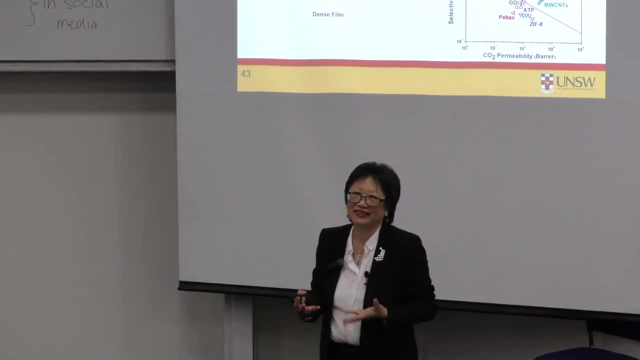 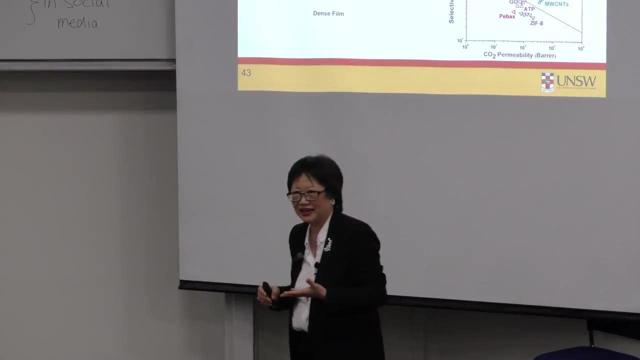 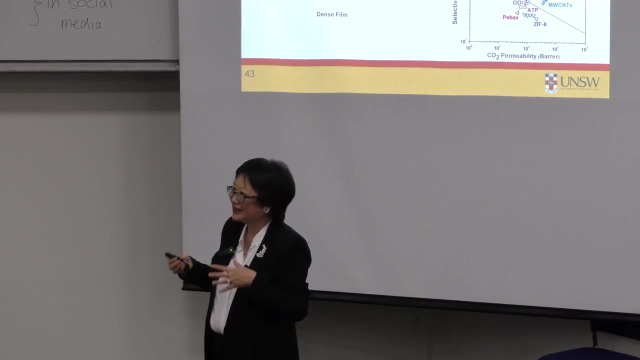 So it's not just the fact that they have that surface segregation. What we think is, those hollow-side nanotubes are quite. nanotubes have somehow changed the, as I say, the macrophage separation of the PBACs, So their range of influence is actually much higher than the amount that we're just putting. 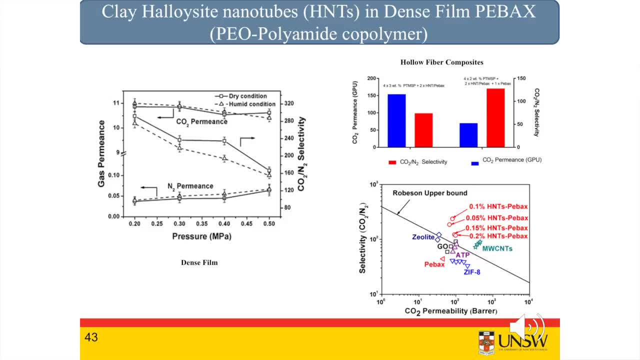 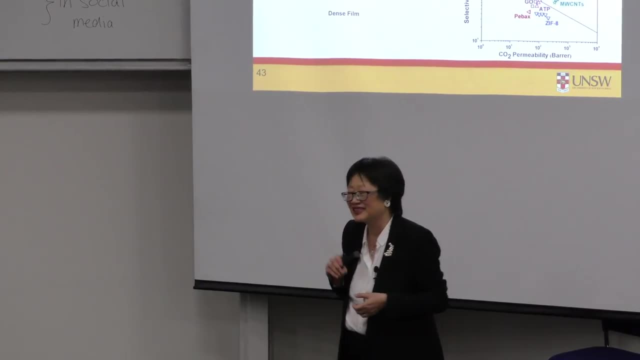 in into these PBACs membranes. Interestingly, if you're just simply looking at the permeability and selectivity, the addition of those halocyte nanotubes would push the selectivity, of course, way beyond the ropes and bound. But I would say, you know, are we really talking about ropes and bound? 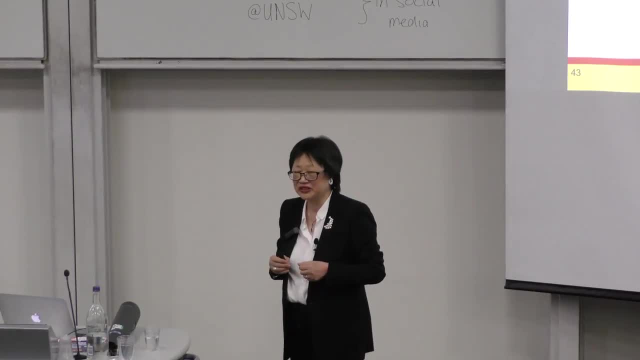 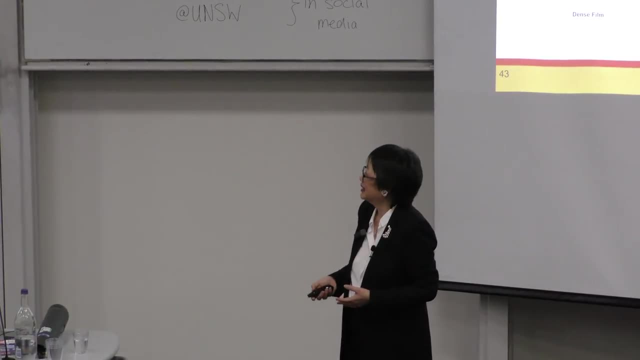 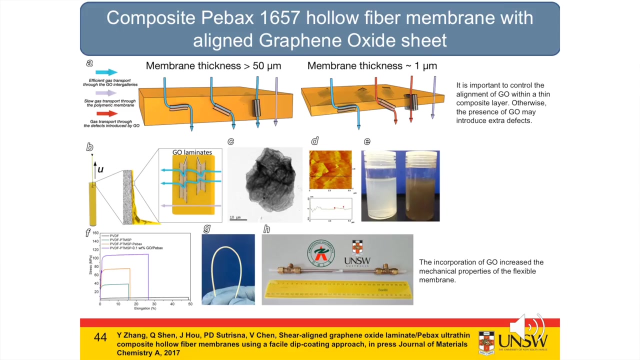 Because it's not a heterogeneous- sorry, a homogeneous- material. You have basically a surface-segregated layered structure. So this is quite interesting, that putting these nanomaterials can have a zone of influence much higher than just their volume fraction. The other thing that we can do is put a 2D material, and graphene oxide has been used. 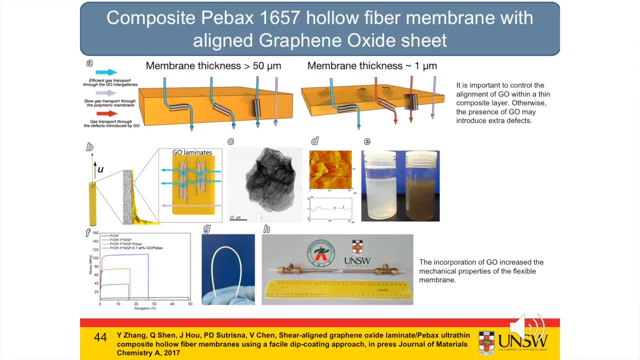 quite frequently in much of the literature. So we thought about thinking about: well, if we put a 2D material- graphene oxide is not specifically. we think about that as a barrier rather than necessarily a CO2 selective material. But what way? 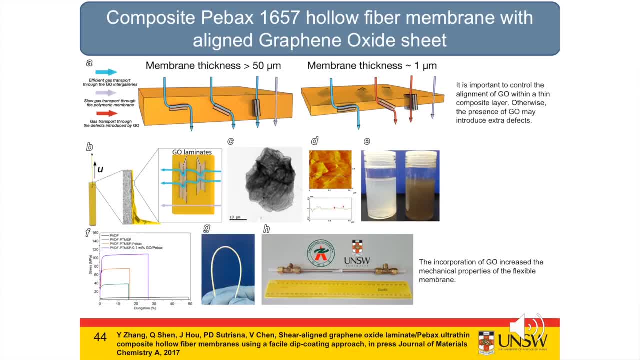 What we found is gas transport through those interlayer structures. the geolaminates are much faster than the solution diffusion. So if we disperse this material in thick membranes, it doesn't really matter so much in terms of the orientation. But once we start to try to push down the membrane thickness, the alignment of those 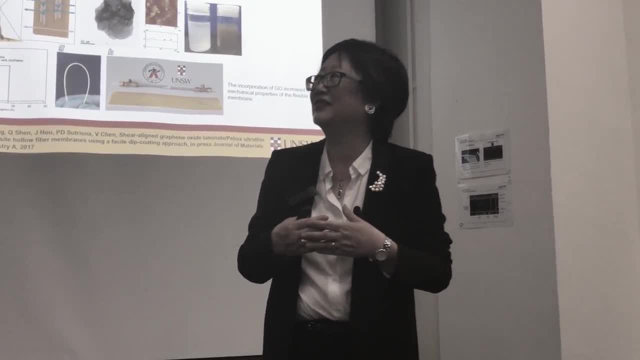 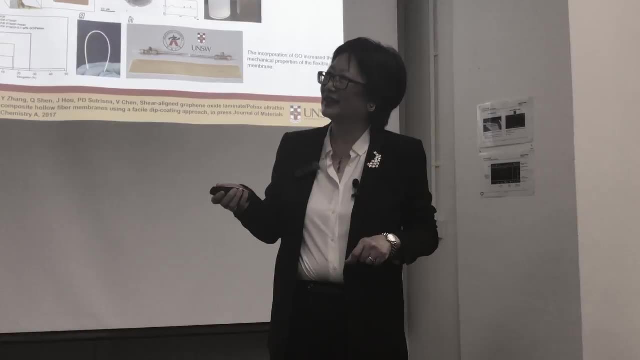 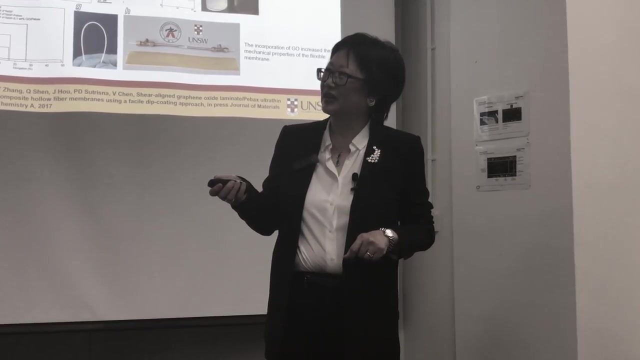 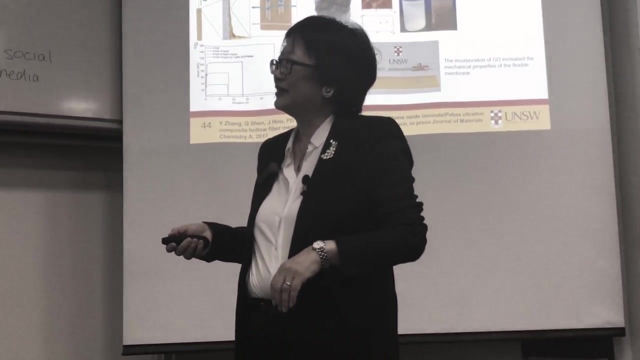 layers become critical, right, Because you start to get potential for defects and other issues. Now, putting that ultra-thin Geo in the ultra-thin layer, or do it by, say, dip coating, so we're basically coating the surface, just pulling it out and allowing the surface film to drain, we get really quite. 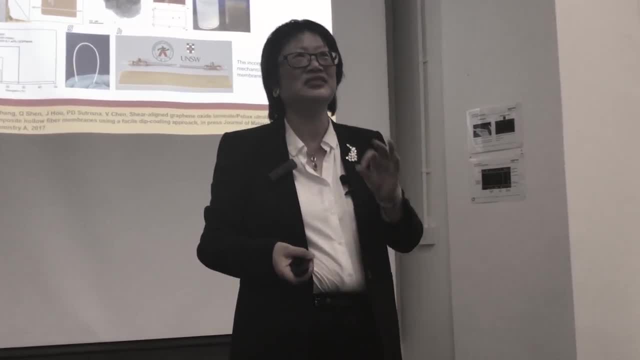 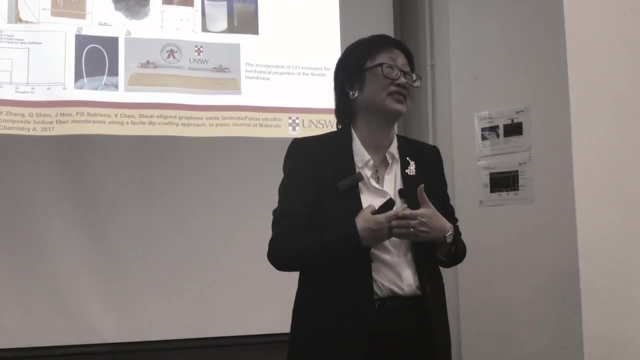 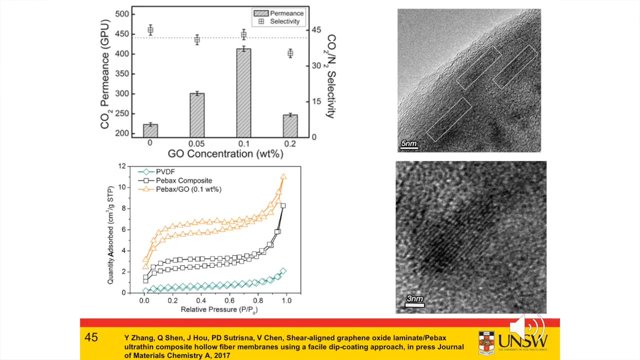 an incredible increase in terms of mechanical stability. So this is just a sub-micron layer of polymer plus graphene oxide and you get just the addition of that graphene oxide. It increases the mechanical, The mechanical robustness of that membrane enormously. What's really awesome: if you actually now look closely at the graphene oxide, you notice 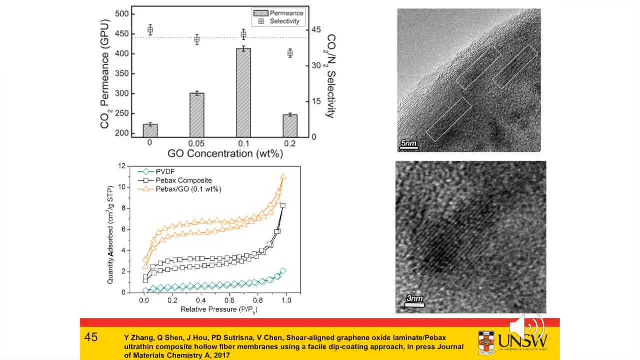 here. at the right coating conditions, you can actually get those graphene oxide to align parallel to the surface. Now that turns out to be quite important because, as I said, if you have a crumpling of those graphene oxide, you actually start to induce defects. 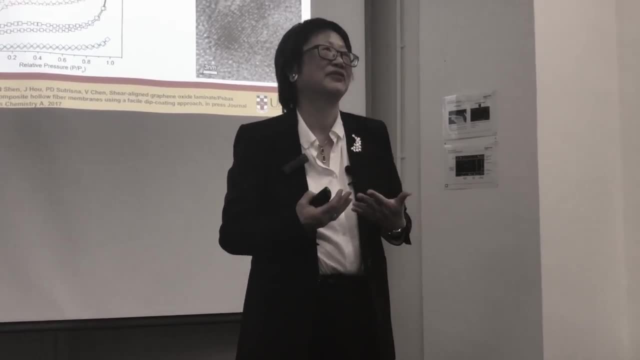 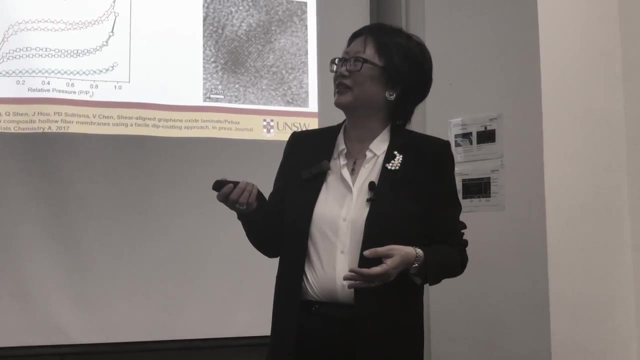 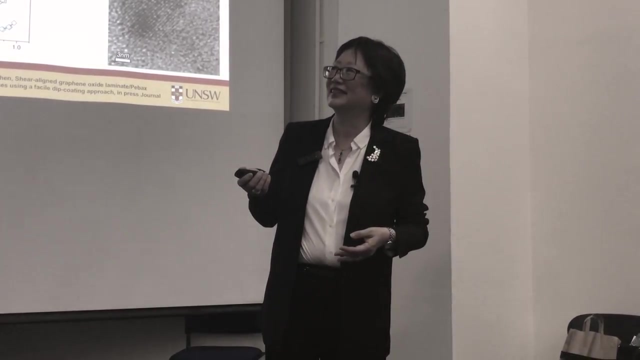 And we see that If we add too much graphene oxide or we don't have the right coating speed, So the graphene oxide we can increase. for example, we can almost double the permeance of the CO2 in these membranes, while still maintaining the selectivity. 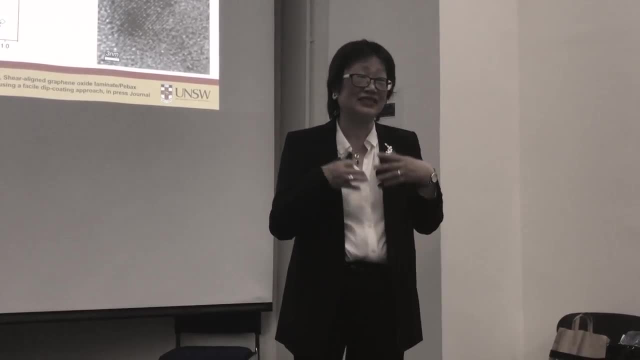 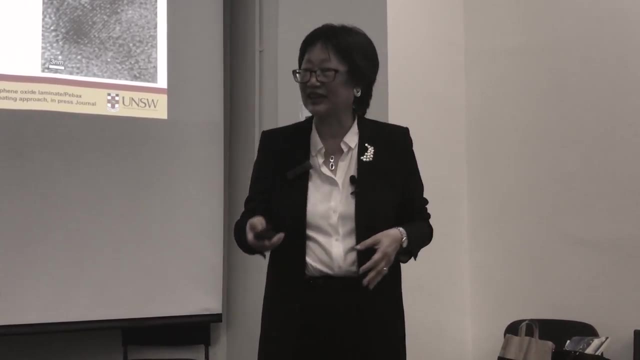 If we put in too much graphene oxide, we start to get aggregation. This is often the main problem with nanomaterials: High loadings, you get aggregation and then again defects starting to come up. So you, So how do we actually get the alignment? 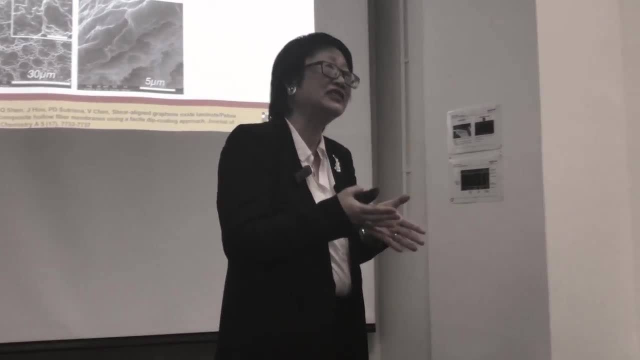 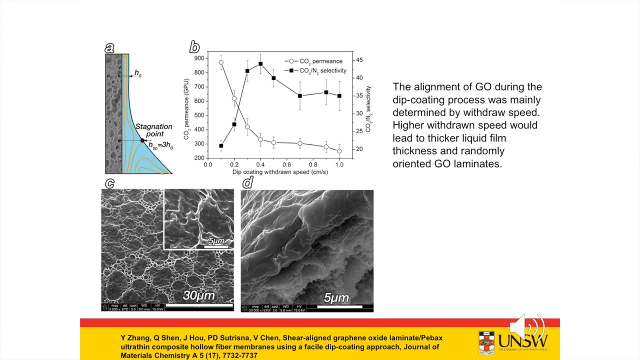 Well, one of the things that we explored is basically changing the withdrawal speed during the coating. So it's basically like a pure hydrodynamic issue. If we get the stagnation point of the draining fluid to be slightly smaller than the lateral size of the graphene oxide, they actually are pulled by the surface tension into parallel. 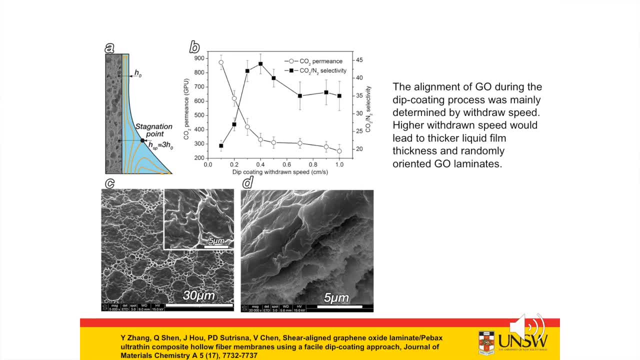 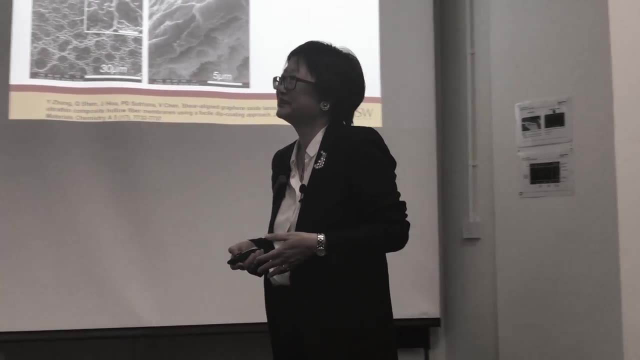 on the surface. If the stagnation point- what's in the coating? It's too small, It's too big, The graphene oxide layers can actually tumble and crumple and you start to get a defect. So this is really a hydrodynamic issue about coating rather than a chemical issue. 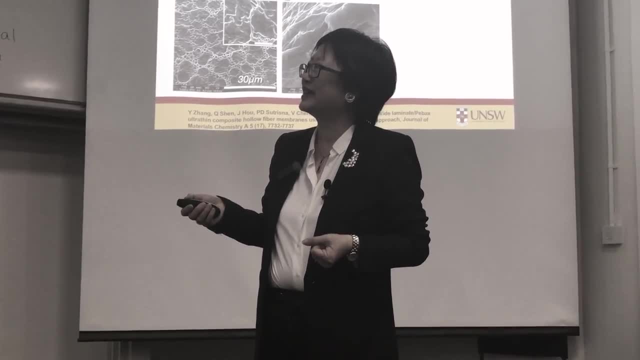 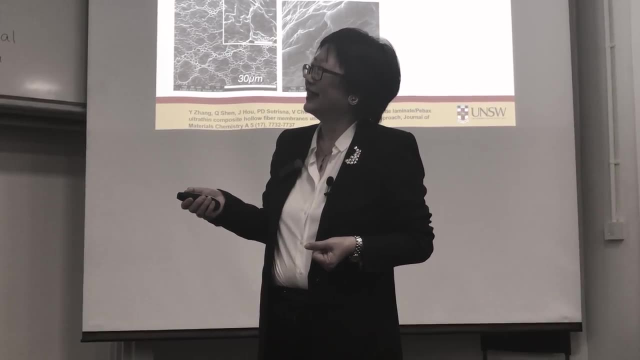 So we get a compromise between permeance and selectivity and we get some kind of optimal, as I said, with being able to go from a very high permeance but really low selectivity to sort of, as I say, maintaining your selectivity. 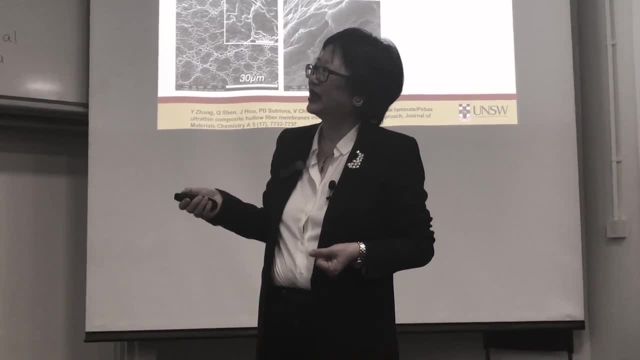 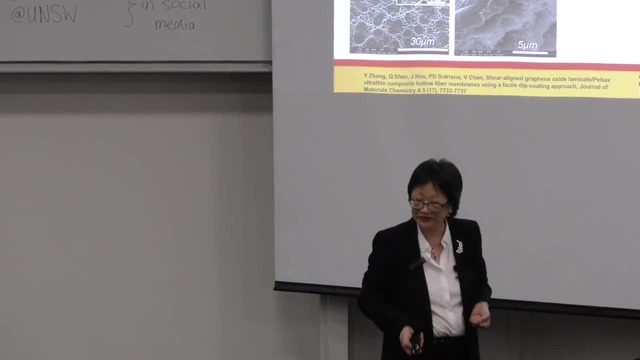 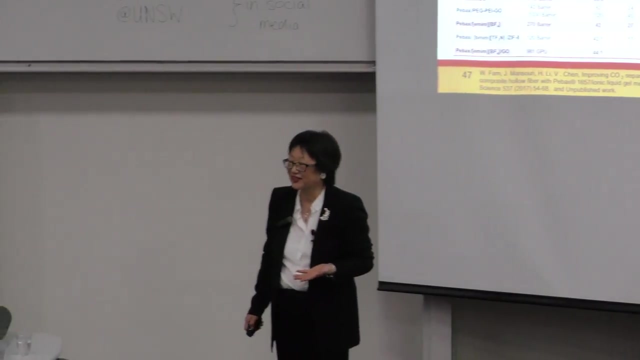 Maintaining your selectivity, close to what the polymer matrix is, but much higher, but being able to still have significantly enhanced permeance of the CO2.. So you can play a lot of games with these sorts of material. You can actually functionalize the graphene oxide. 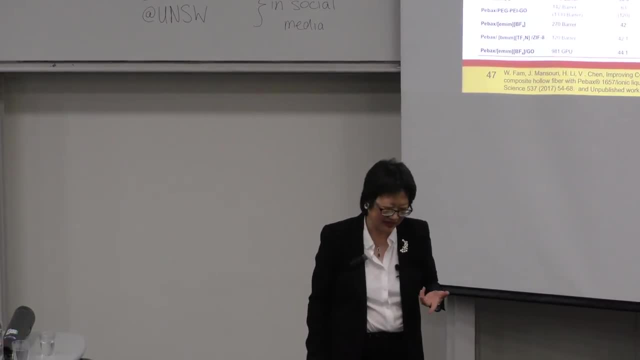 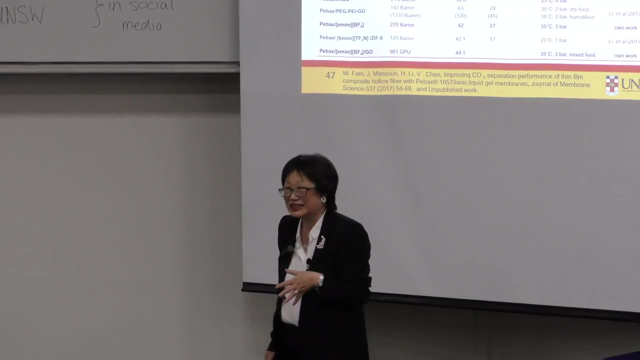 Some of the things we're doing is, for example, coupling with the ionic liquids to improve the permeance of the CO2.. But it turns out that ionic liquids can also functionalize graphene, Yeah, Graphene oxide, and basically you can get again. you start to be able to push up the 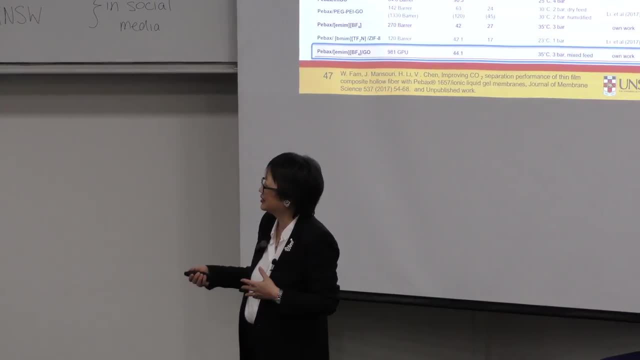 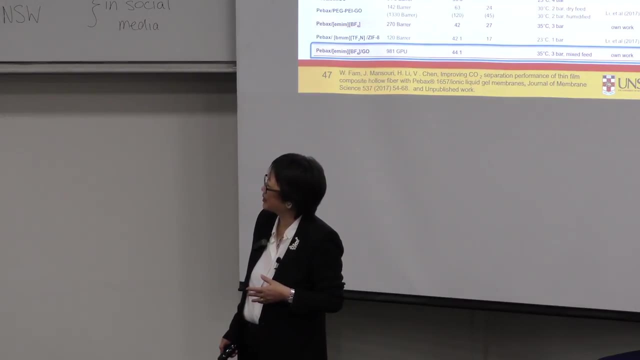 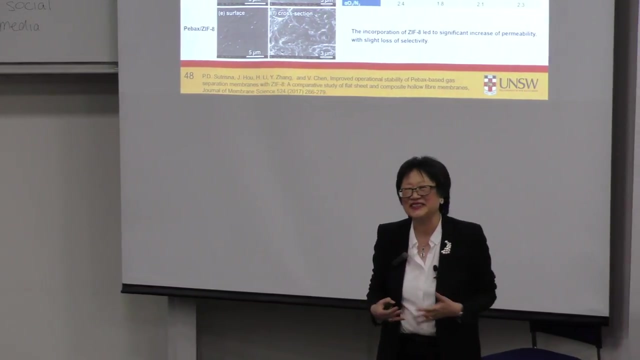 performances of these composite membranes up to, as I said, the 1,000 GPU, still maintaining very good selectivity with these sorts of composite membrane. All right, So now, as I said, I've shown you 1D material, I've shown you 2D materials. now we're going. 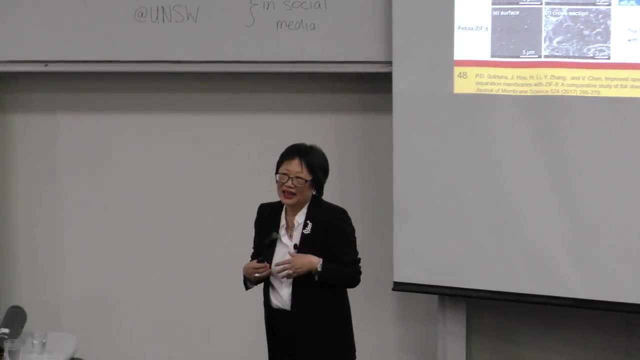 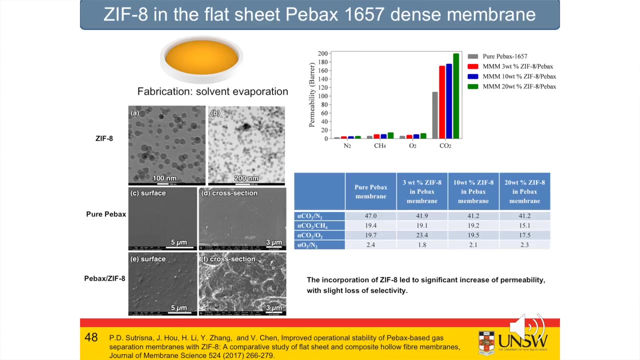 to come back to our framework 3D materials, Most of the approaches in terms of Using these net organic framework, other 3D zeolites and things is really what they call the mixed matrix membranes. Basically, you just put the membrane, you just put suspensions into the solvents and 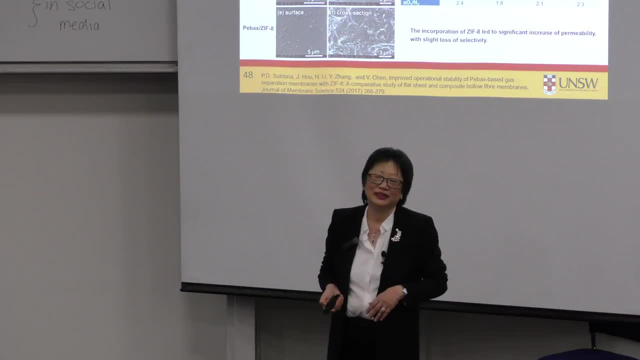 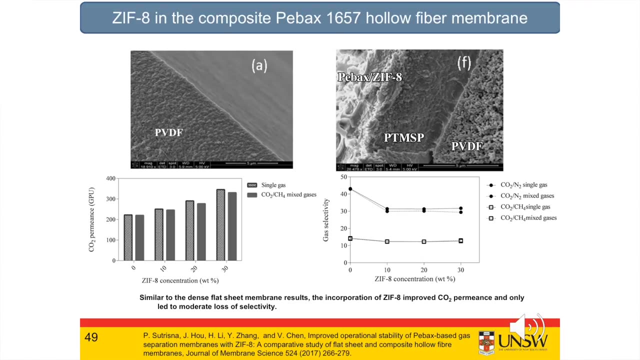 you just cast as a thick sheet and you get some improvement in the performance, but not usually much in terms of selectivity. What we found is that with putting things like Zip8, you get a slight decrease in the selectivity. We think it's because there are still some issues with myodefate. 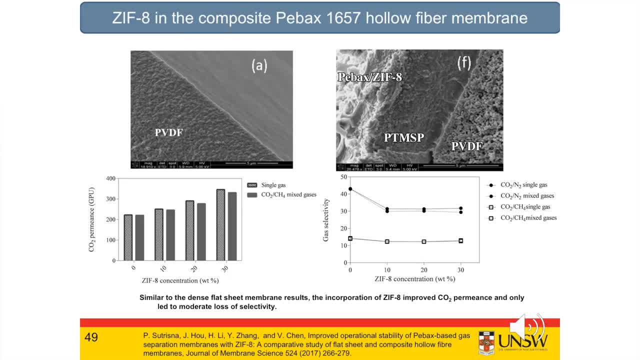 But we're going to come back to that. But the other thing to think about is some of these metal organic frameworks are not like crystals. They have organic ligands. they actually have a little bit of flex in them, right? So when we go to 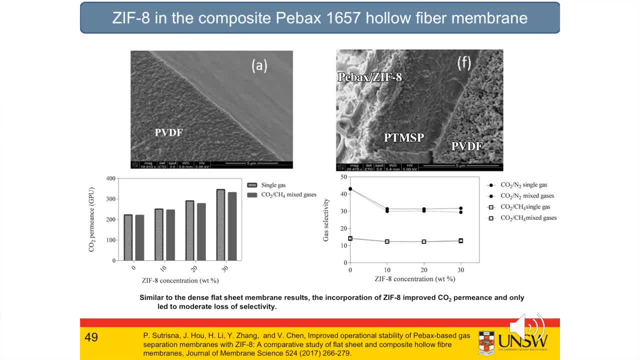 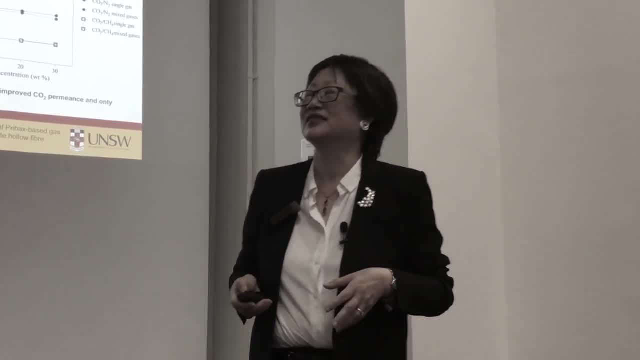 We start to pressurize these things, we may be causing, as I said, either producing a voice, or are we actually causing some changes in the aperture size of some of these metal organic framework? So, with more rigid ones, as I said, we don't see. 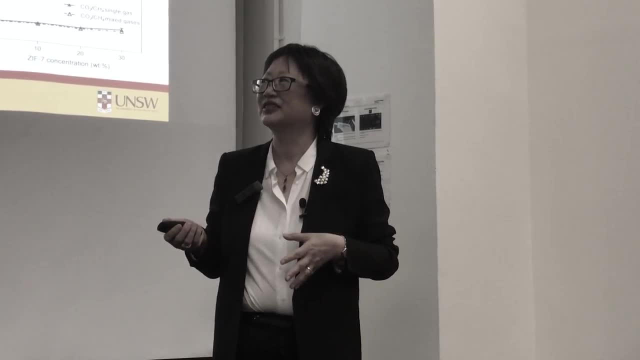 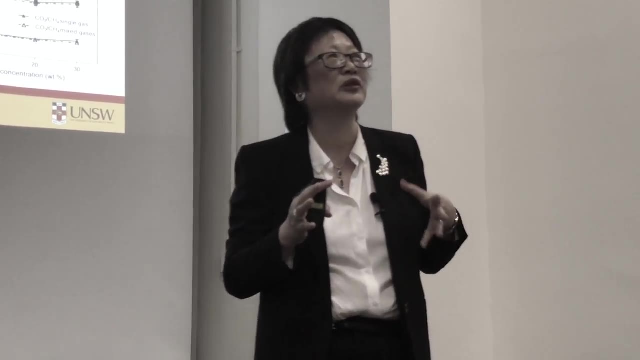 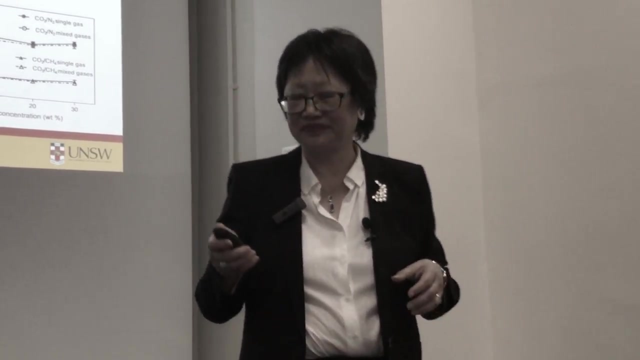 We see the slight loss in selectivity. so with the Zip7s. so it's not a Compared to the Zip8s. So this is quite important for you to think about these framework materials as not quite like crystals. They're kind of an intermediate between soft and hard framework. 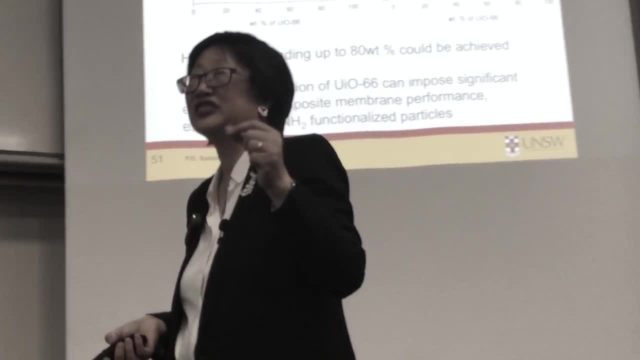 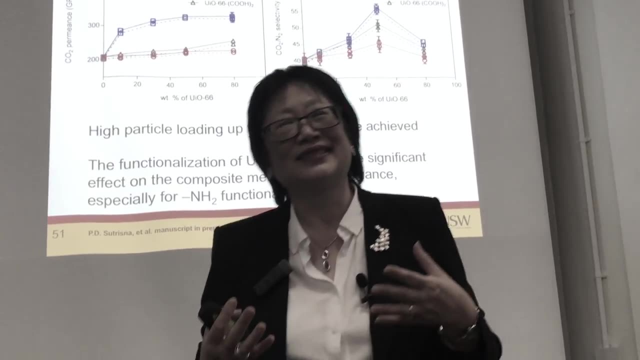 So the interesting thing is to take So Zip7. Sorry, Zip8, it gives you increase in permeability but not much increased selectivity. but Zip8 doesn't have much intrinsic permeability. It gives you intrinsic selectivity of CO2 over nitrogen. 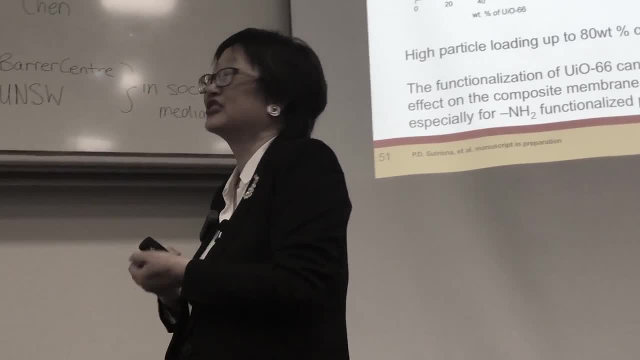 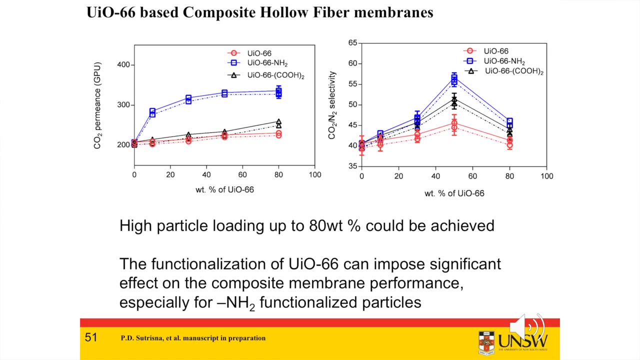 However, if we now move to the UiO66 with the zirconium coordinated framework, you can functionalize those with carboxyl groups and avian groups And what we find is when you add those material, you can get both: the increase in selectivity. 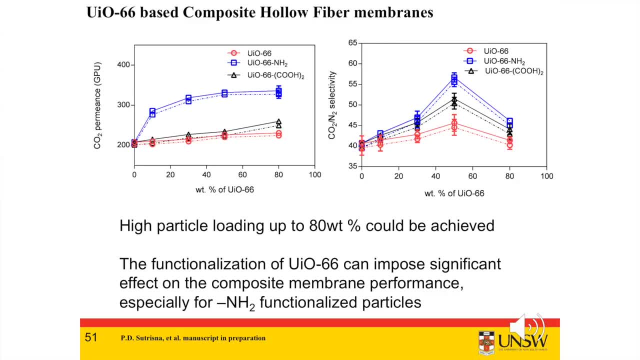 and an increase in permeance. And because of the functionalization, you can get up to extremely high particles loading. And because we're doing this in the Composite structure, we don't have to worry so much about the mechanical robustness of support that a freestanding membrane we need to have. 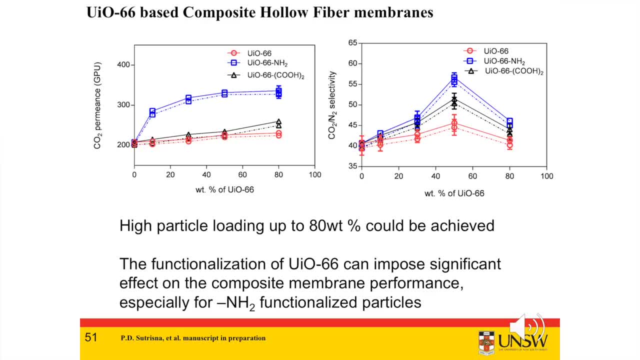 So this allows us to really play around with In terms of the kinds of materials you can add and going to extremely high solids loading to get that intrinsic performance from those metal organic frameworks to come out, not just simply be dominated by the polymer mix. 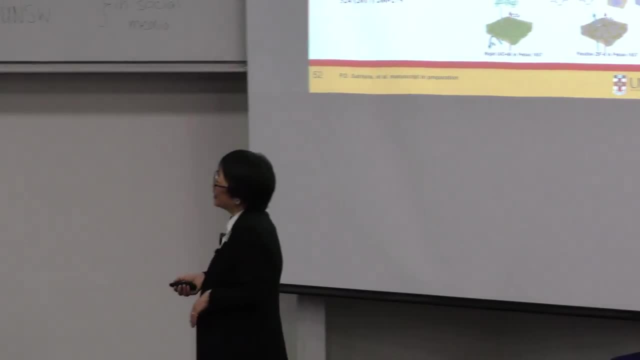 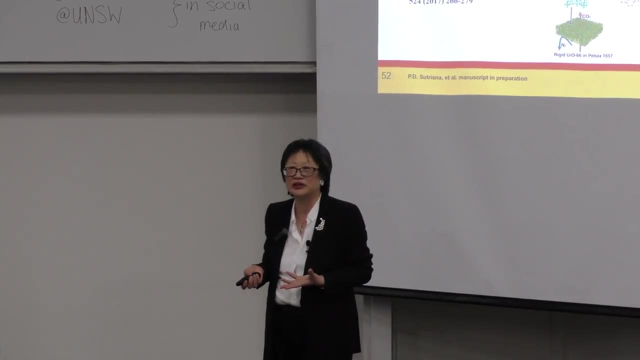 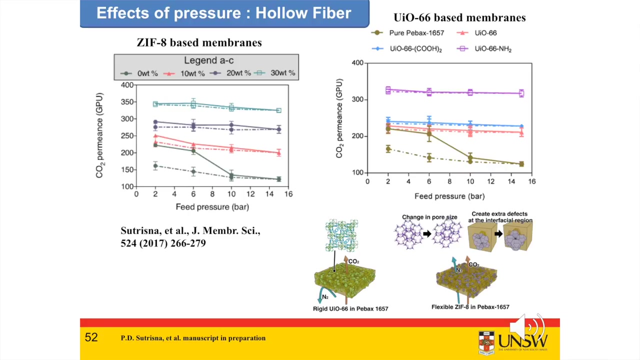 So, in the interest of time, just quickly, so that one of the interesting things- adding these particles not only increases performance but also in terms of compression. we don't We actually can show some rigidification of the coatings Without the nanoparticles. we get hysteresis. 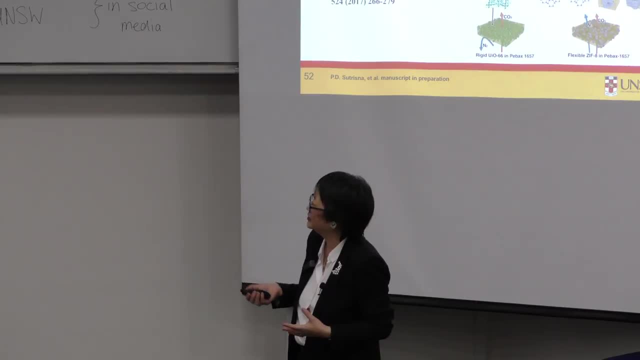 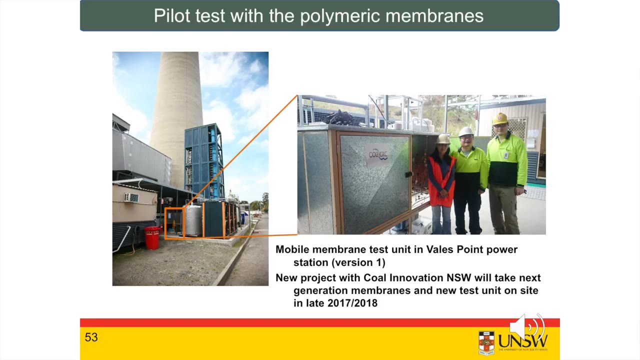 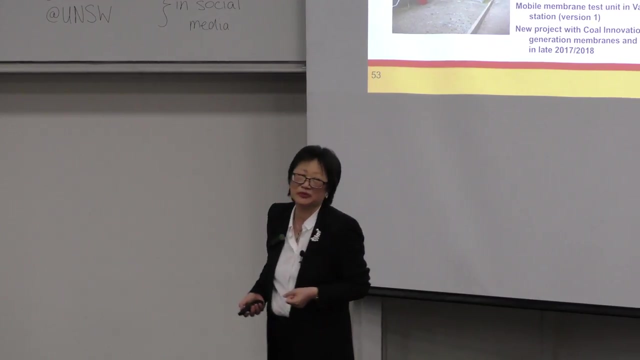 When we pressurize and depressurize, when we add these particles, we do get much more, greater stability. So we are taking some of these membranes. This is the flue gas power plant where we're actually going to test some of these membranes. 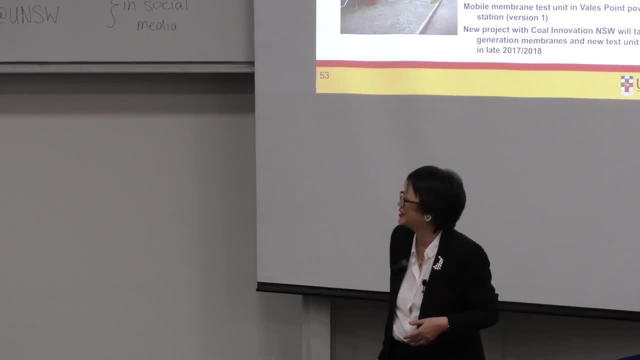 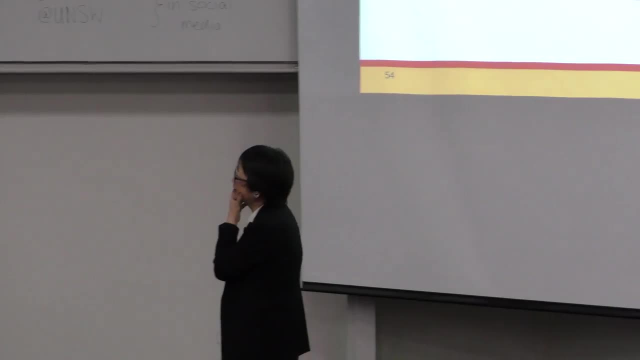 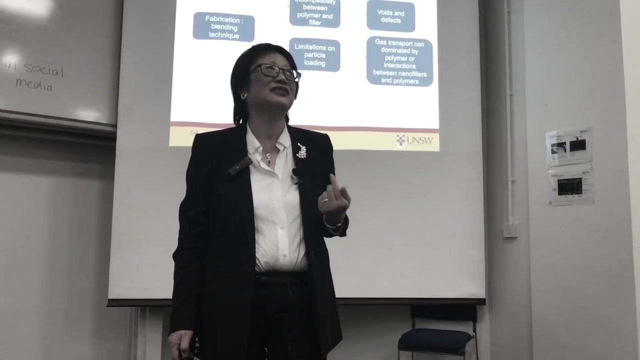 with real flue gas in the coming six months to a year. So I'm going to finally finish up by just talking about that. mixed matrix membrane gives you one lever, But it still has a lot of drawbacks. One is incompatibility. The polymer: 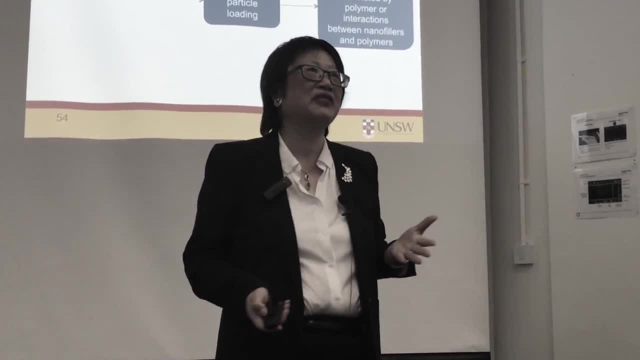 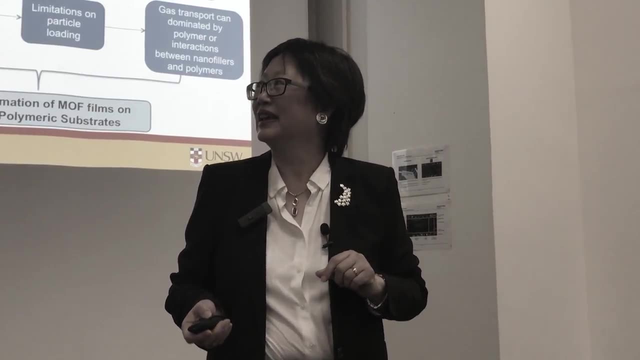 We can Limitation particle loadings. So can we get around that by saying, well, let's just make a layer that is fully? That is framework material. So we want to now think about in situ formation of MOFs on porous membrane substrate. 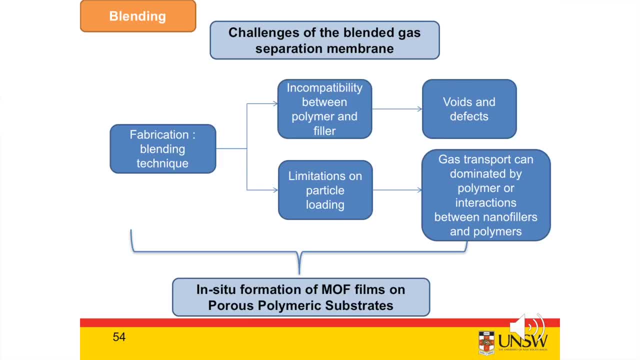 Now this is not a new thing. People have been able to create MOF layers on inorganic substrates, also in polymeric substrates and also by counter diffusion Right. But many of the cases that is very, very thick and therefore you lose many of the advantages. 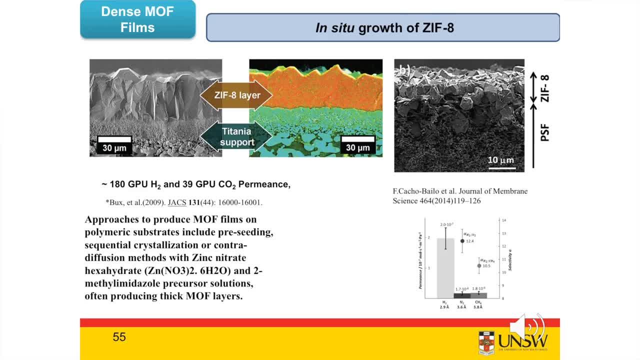 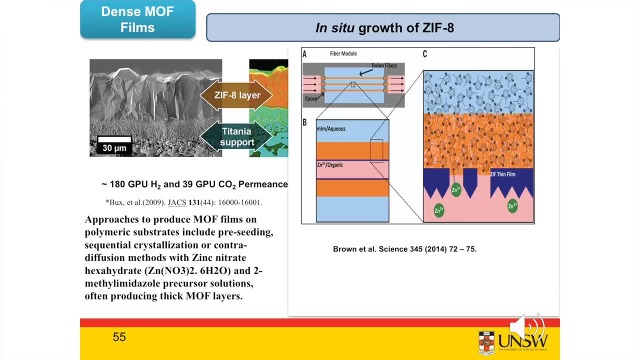 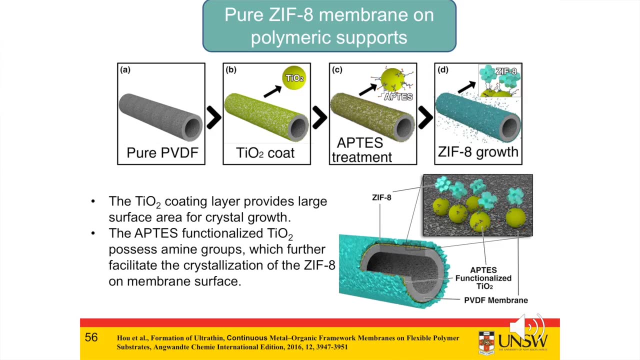 of the framework material. So we thought about a way that we can actually overcome that and say: look, let's make the surface really compatible and also provide the right environment to nucleate those framework materials and form those in situ. So what we did was actually we took those lovely titanium coated surfaces and functioned. 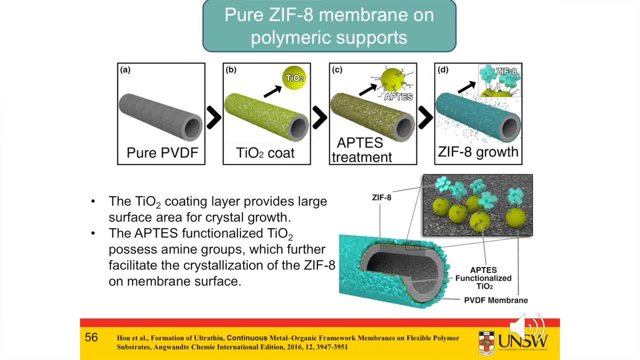 them. So we took those and we functionalized the silane groups and those groups can actually chelate the metal coordinating centers and actually grow the metal organic frameworks in situ. So they provide the hierarchical roughness that allows you to key in those growth of. 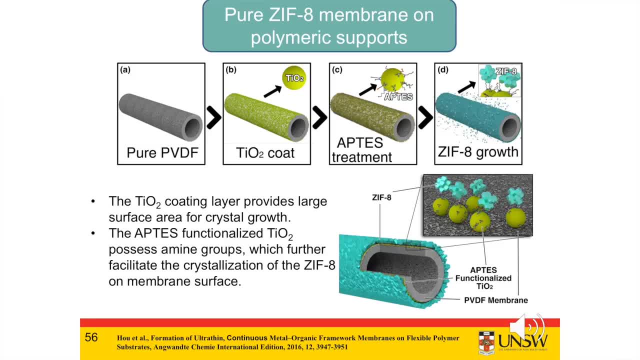 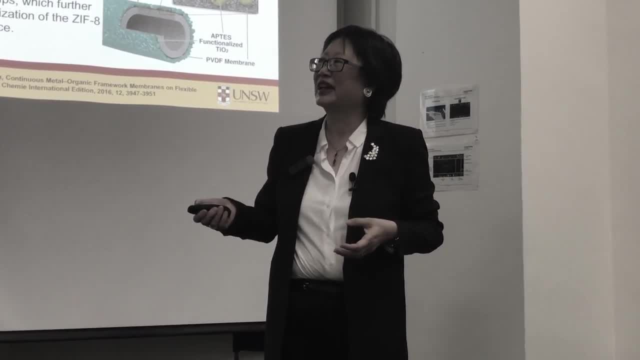 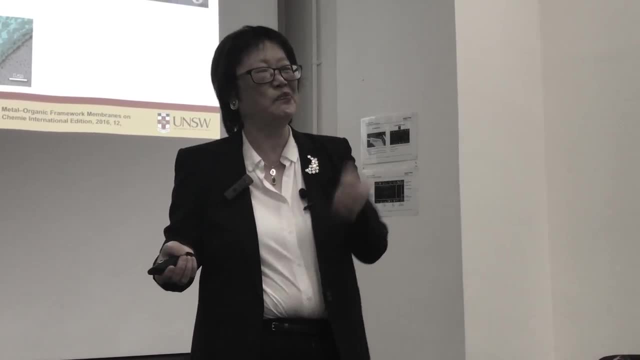 those crystals, but also allows them to grow evenly and smooth. In fact, we were able to do that: make a coordinated- sorry, a coherent- metal organic coating onto a polymer substrate. So So this is not under any evasive. We basically take the hollow fiber membrane and we just coat it with a titanium coated. 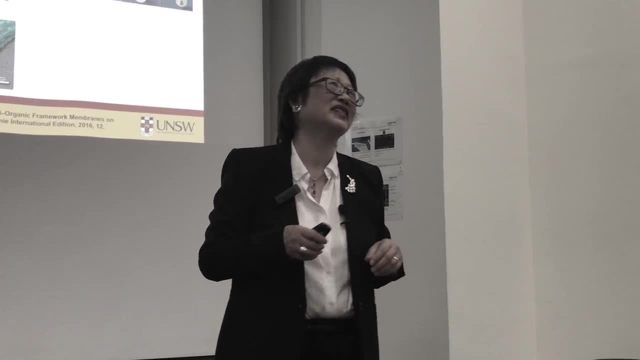 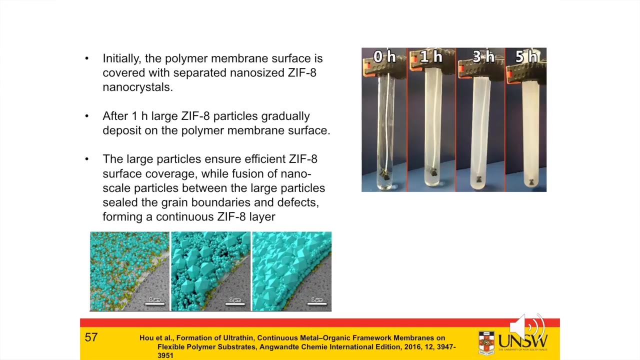 fiber membrane and just throw in the precursors for the ZIF-8 and basically it forms in situ. No high temperature, This is at room temperature. This is no solid thermal processing, just simple reaction in situ. So we can see the form exceeding growth of those crystals and coherency. 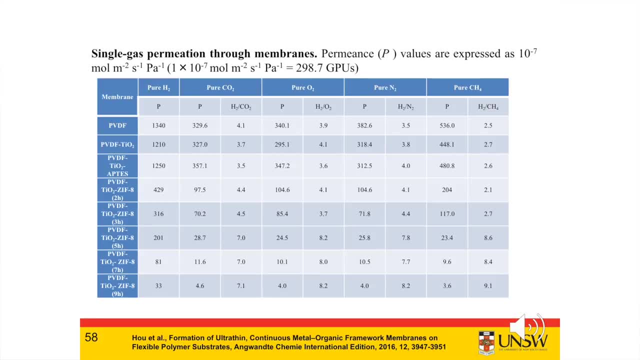 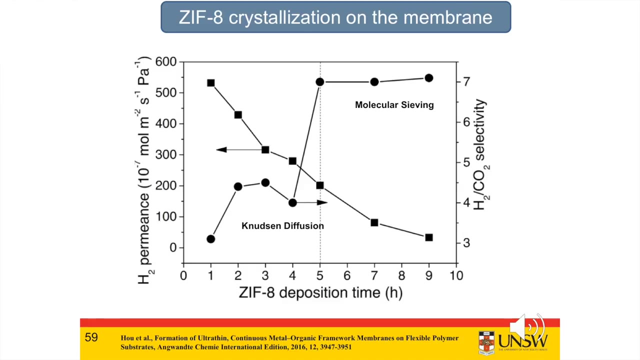 So So this allows us to grow ultra-thin layers and allows us to achieve, basically, molecular sieving at ultra-high permeation. This is for one of the highest reported CO2 permeate Permeances reported for these sorts of metal organic framework membranes. 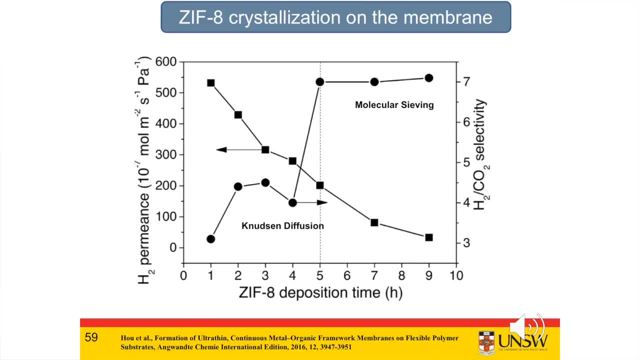 So, basically, we can show that we go from nuscent diffusion to molecular sieving. Selectivity is still not. that Is basically representative of the pure ZIF-8.. The permeate, The permeance, as I say, is extremely high. 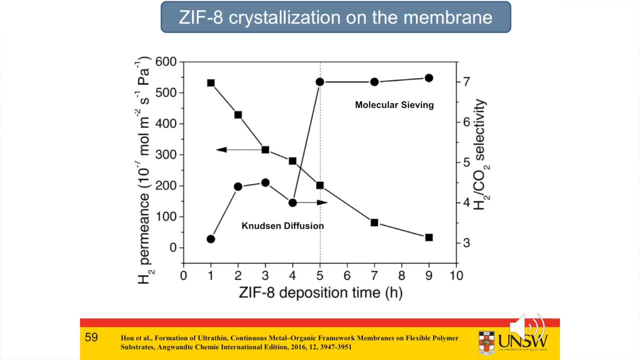 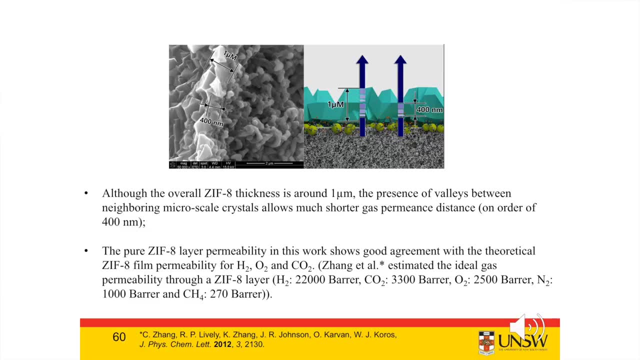 And what's interesting is when we back-calculated the permeance with Versus Chorus' group's calculation Evaluation of ZIF-8 permeability, we are basically in that right ballpark. So basically we're making a half micron ZIF-8 thickness and it has pretty much the same. 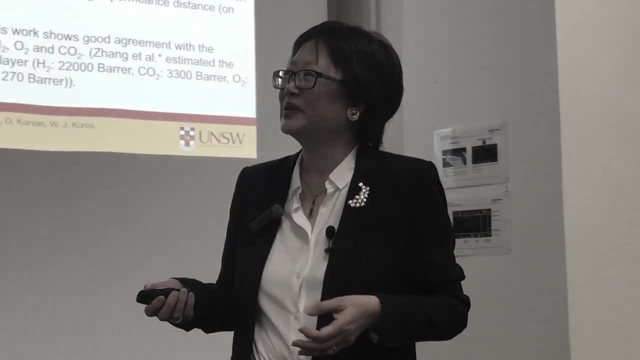 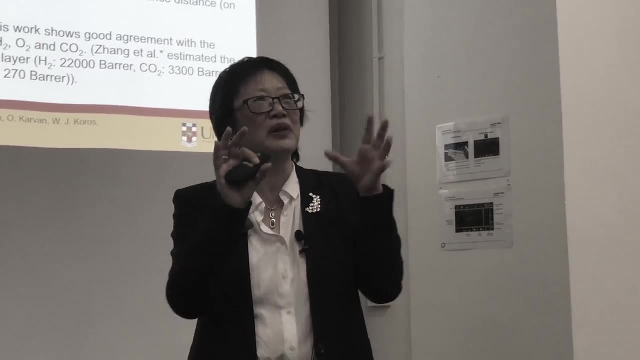 selectivity as for hydrogen and CO2.. For some of the other pairs it's not exactly pure ZIF-8.. Pure ZIF-8 behavior- And we think it's. Some of the issues- is that. remember we have a basically flexible substrate which may. 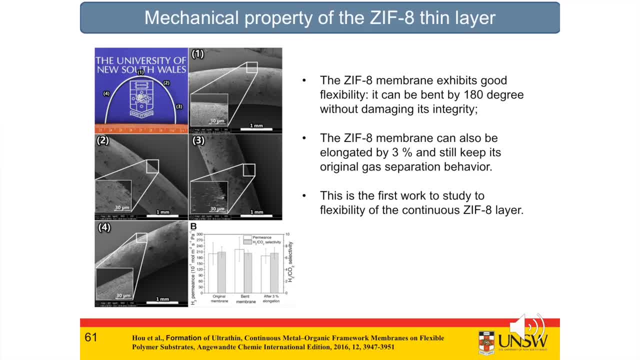 cause some flexing of the ZIF-8 coating. So this layer, as I say, is not fragile. It can actually bend a little bit because of those, Because it's ultra-thin And, as I said, ZIF-8 does have some flex in the structure. 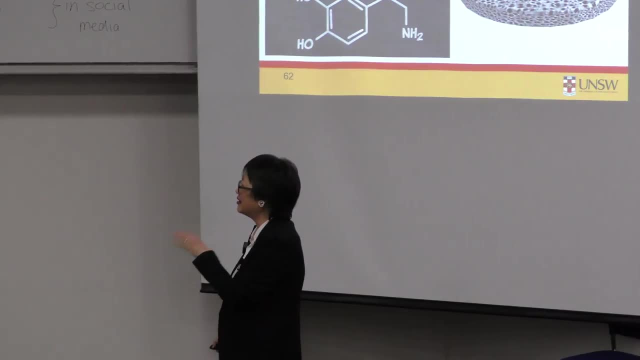 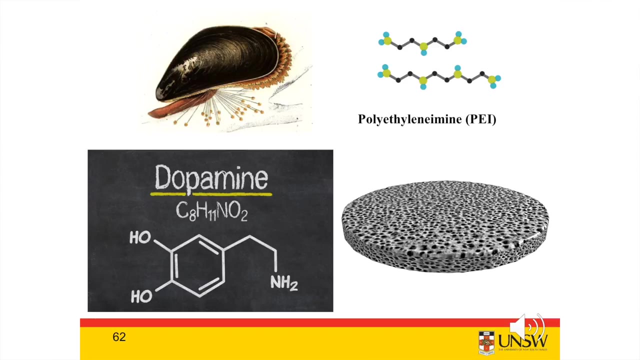 Now we can actually play the same game again in terms of saying: well, how else can we add catechol and amine groups to nucleate those metal organic framework materials? Well, we can add things like polydopylene and polyethylene amine and that form a very 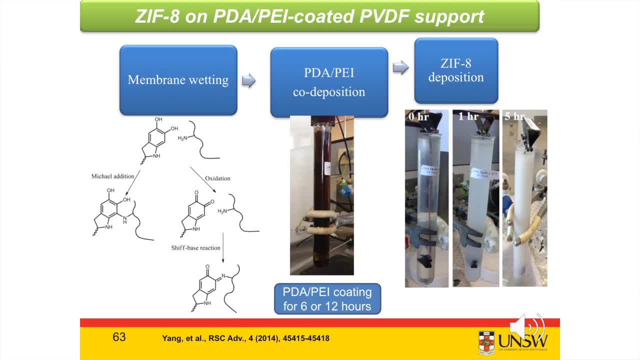 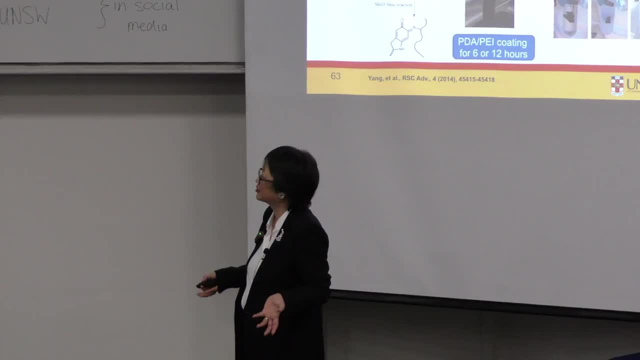 nice adhesive surface and then again chelating those metal centers. And in this case we simply coat it with PDA, PDI, and then again throw in the precursors for the ZIF-8, and they form spontaneously on the surface. 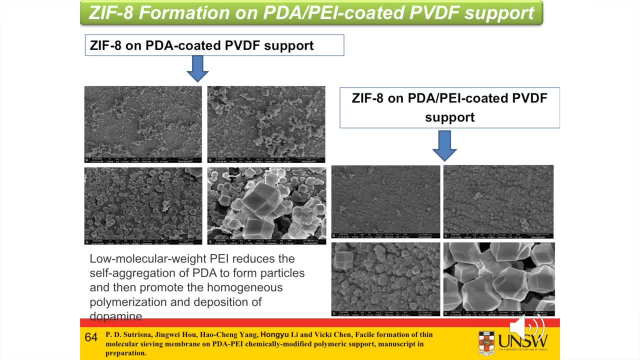 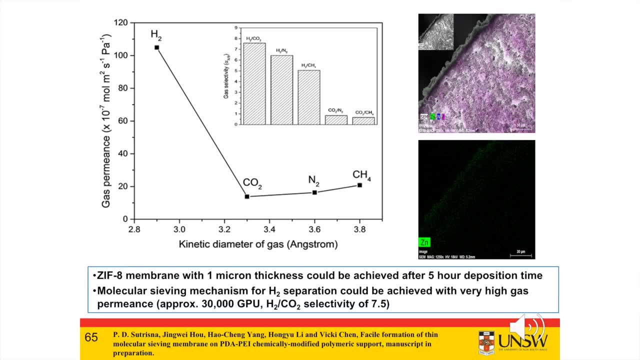 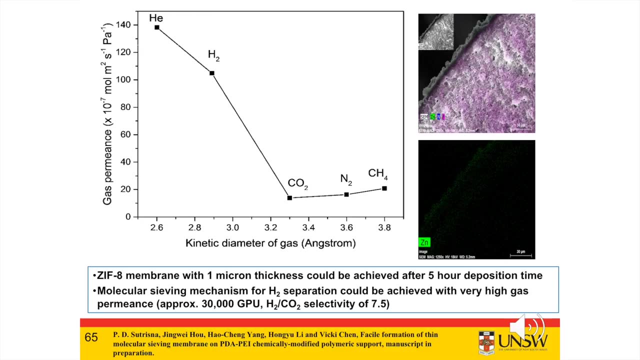 So So the PEI makes a much more even coating compared to just using polydopamine, for example, And we can see again. we get high, for instance, about half of what we got with the titania-coated surface, but we still get molecular sieving. 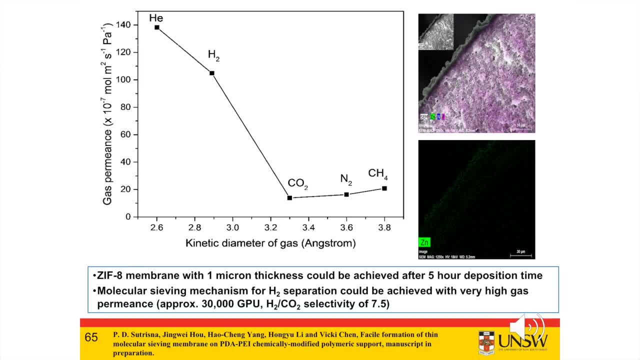 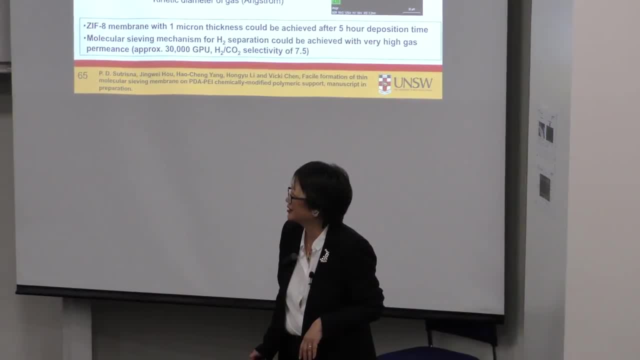 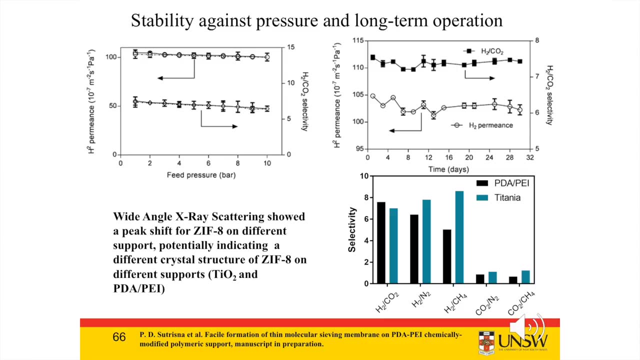 And we're here for helium hydrogen and CO2 separation. so very, very high, but ultra, But still very, very thin layers Interesting. We wanted to be sure that we can have stability, so different feed pressures, number of days. 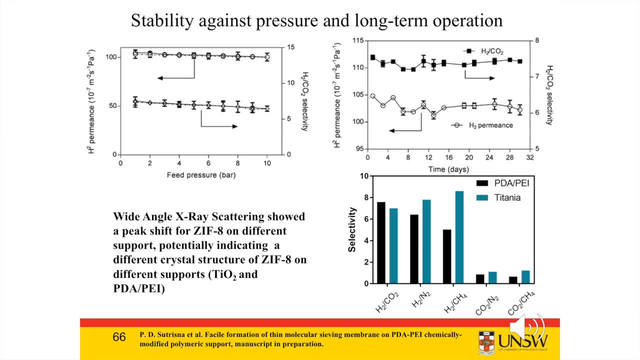 So this is quite a stable ZIF-8 structure. What's interesting is we compare the two types of metal: organic The MOF layers we get for the titania-coated and the PDA PDI coat. they're slightly different. 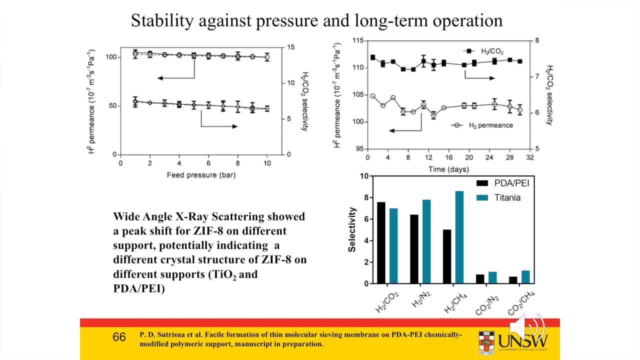 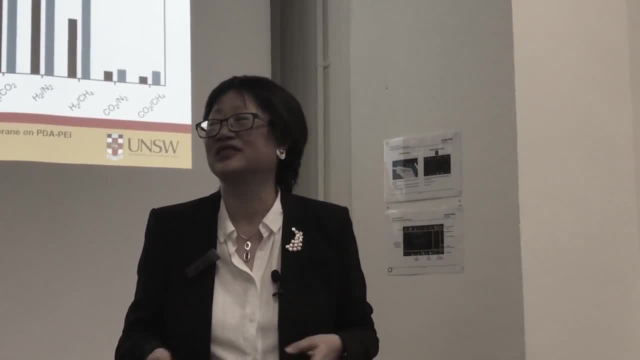 We get. We think that there's a little bit more potential, different crystal structure of the ZIF-8 that forms out of those coatings And that may be because of the types of- Okay, The chemical groups that we have introduced on the surface and the density of chemical. 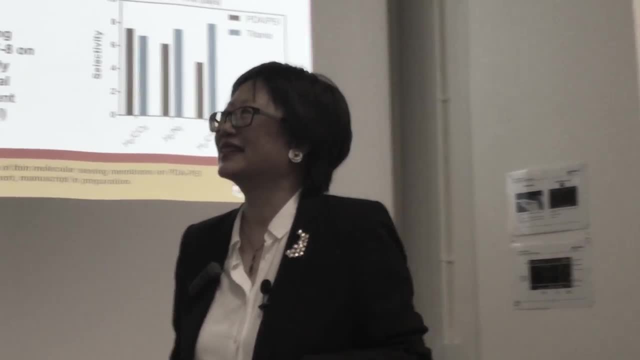 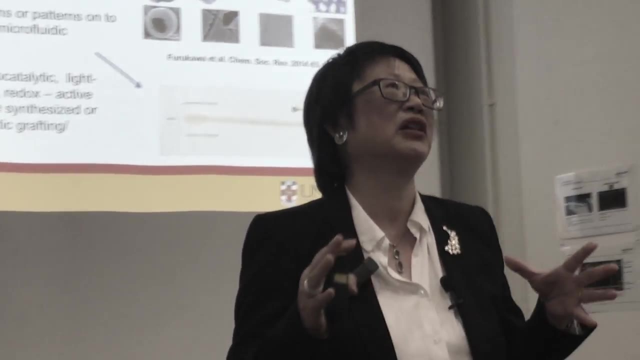 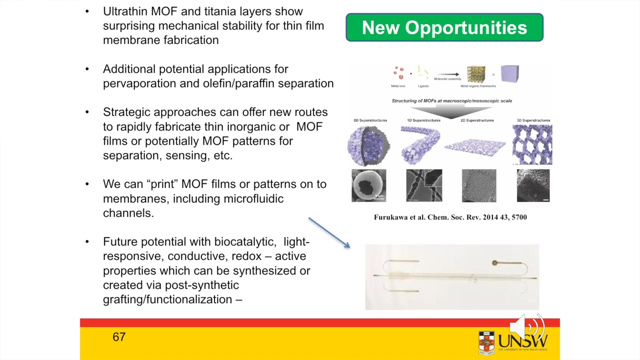 groups that we have on the surface. So where does that take us in terms of what else can we do with this? Well, one of the things is now you can think about. We can now coat polymer membranes with ligands that can generate framework materials on demand. 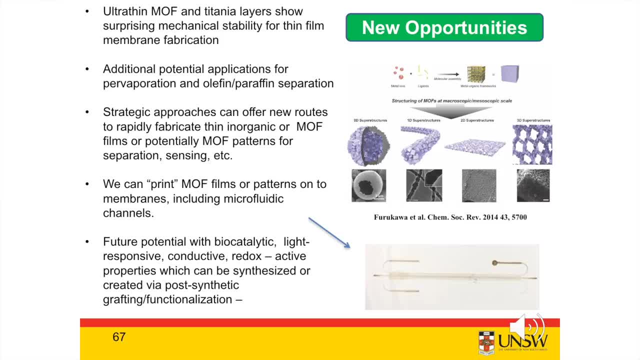 so to speak, And that allows us not to just coat flat sheets but hollow fibers and we can literally print metal, Metal-organic framework films. So we can print the PDA, PDI pattern and we can actually grow the metal-organic framework. 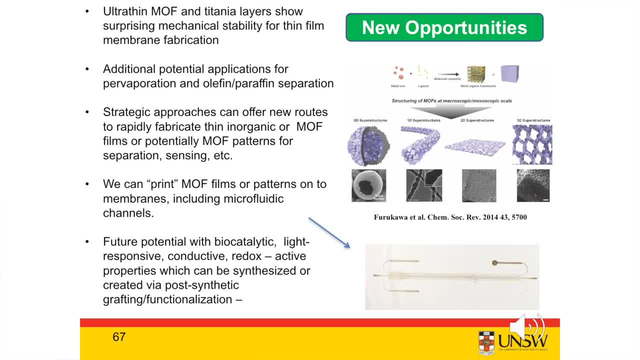 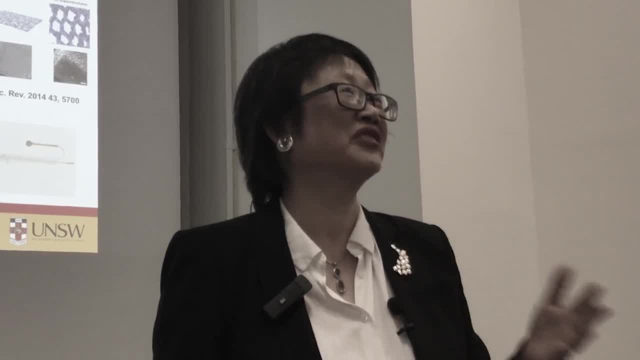 materials off polymers, other types of substrates. So that's some of the work that we're doing. We're also functionalizing some of those metal-organic frameworks with enzymes. It's a talk for another day, but if you want to come speak to me later about it, it's quite. 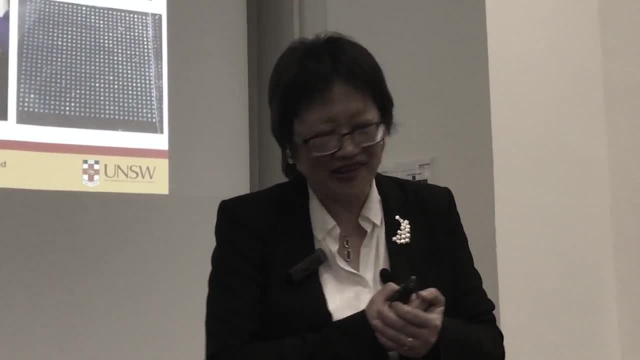 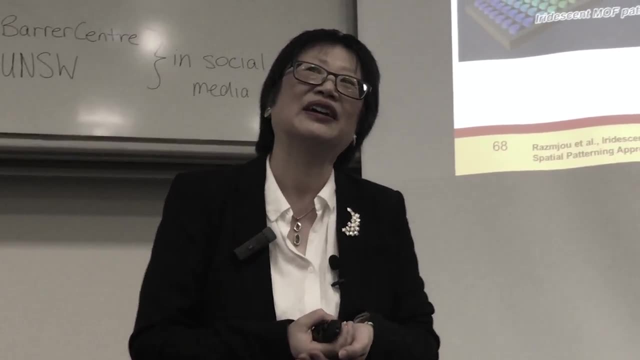 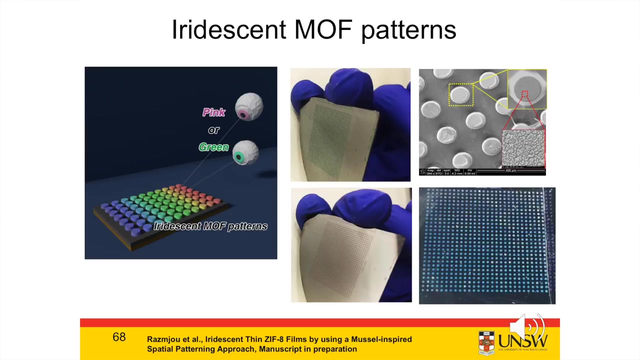 interesting, But I want to finish off by saying about printing. So we talk about membranes for separation. So one of the ideas that we have are looking at let's print metal-organic framework material by putting this PDA, PDI, and we can actually grow them into order arrays. 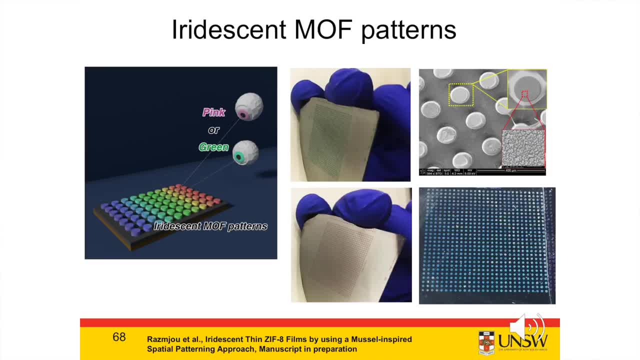 And they have some really interesting optical properties. So one of the things we're thinking: in the future, could we, on a membrane, be able to print metal-organic framework, not just for separation but also encapsulating catalyst particles, encapsulating enzymes. 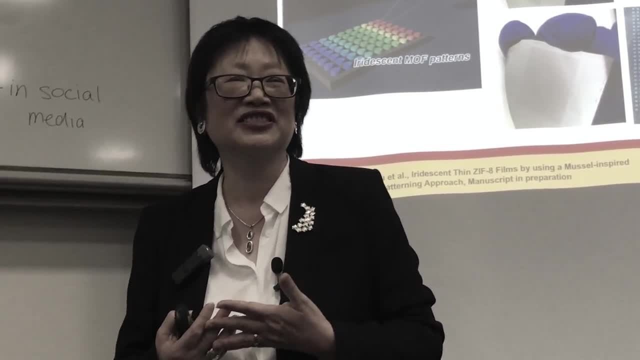 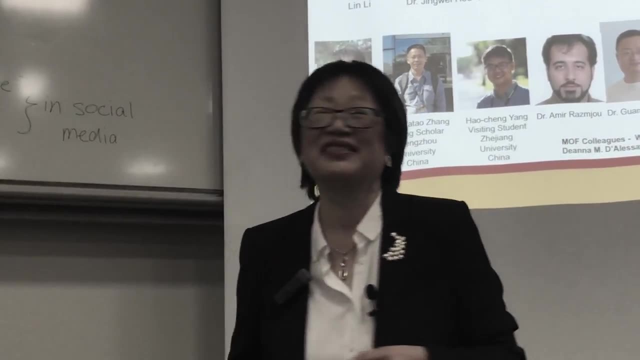 So that's one of the things that we're thinking about. Okay, So will the future be 10,000 months? Can we actually expand and be able to make sensors and microfluidic devices out of them? So with that, I want to finish up by thanking, basically acknowledging the huge amount of 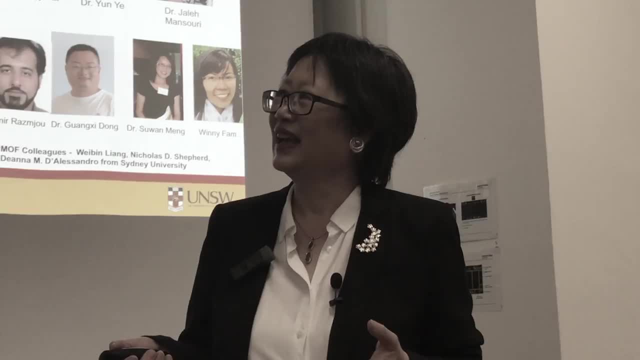 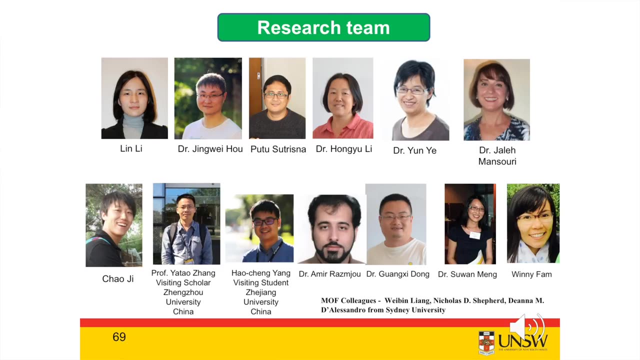 work from my research team, Who's here did a lot of the work in terms of the nanomaterials, integration with membranes, the graphic oxide, the metal-organic framework, has worked on the pervaporation And other students have worked on the.